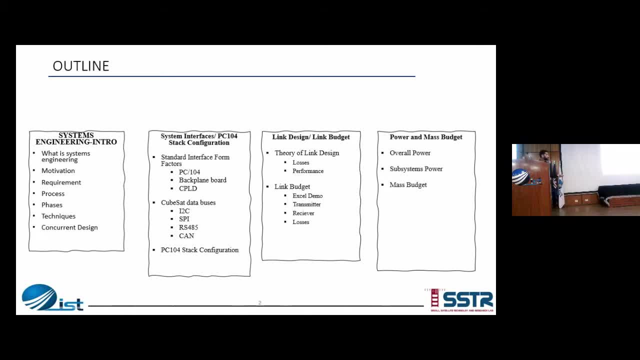 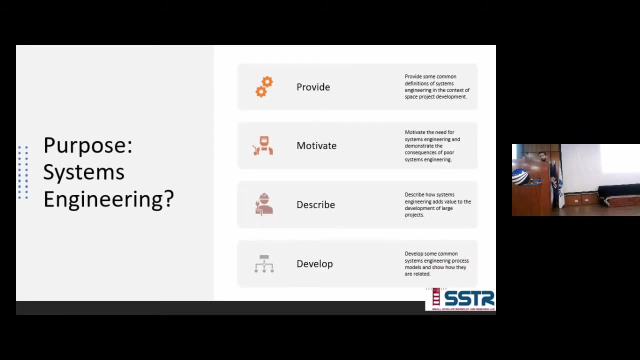 the power and mass budget for our system. So what is the purpose of system engineering? So it provides, basically we have to when we have to develop a system. so in the end the process of integration and during the phases also the integration takes place. So the system engineering plays an important role in that. so it describes that how system 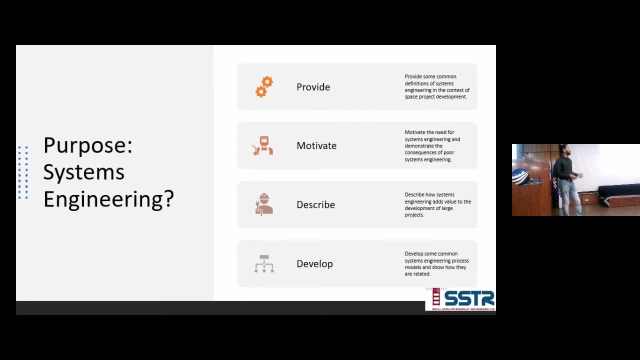 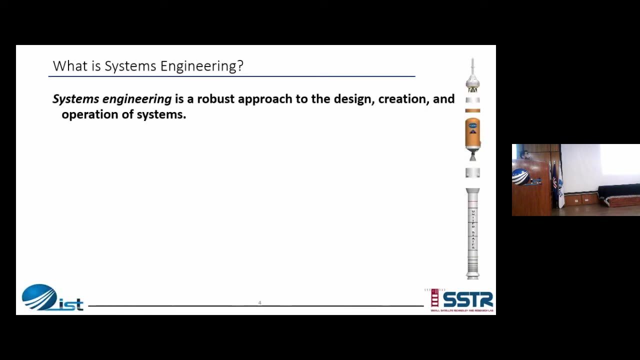 engineering adds values to the system and if it has not been done properly, it may appear that at the time of integration the error and faults may appear, which would result in the failure of the whole system. So this is a robust approach to the design, creation or an operation of systems. 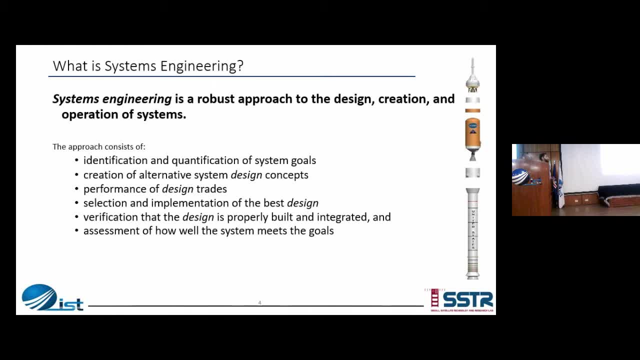 This approach consists of identification and qualification of goals. Similarly, creation of alternative system design concepts. We design some performance tables for that and the selection and implementation that is made based on those tables. Then the verification process is carried out and after that assessment is done that how well the system meets its required values. 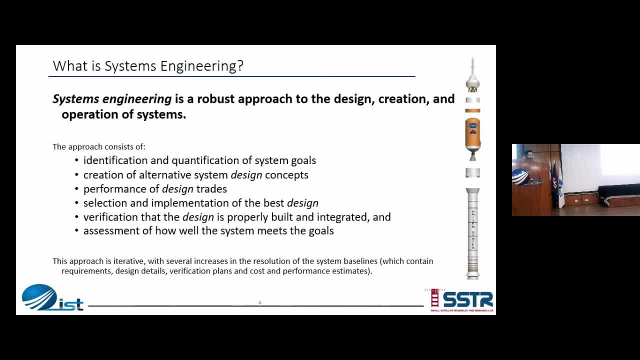 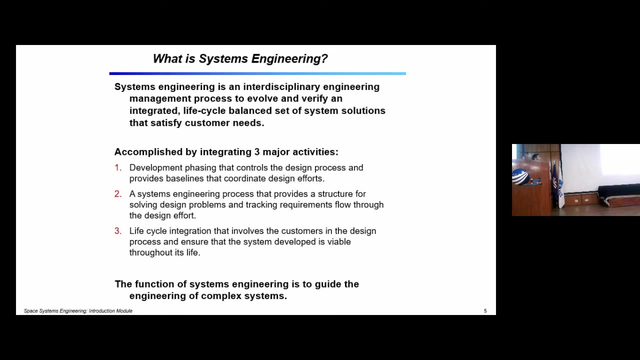 So this approach is iterative and with the passage of time we make improvements and changes to its design and in the end it gets better. So again, the three major activities that are accomplished in this: the number one is development phase, which consists of controlling the design phase and providing the baseline and requirement. 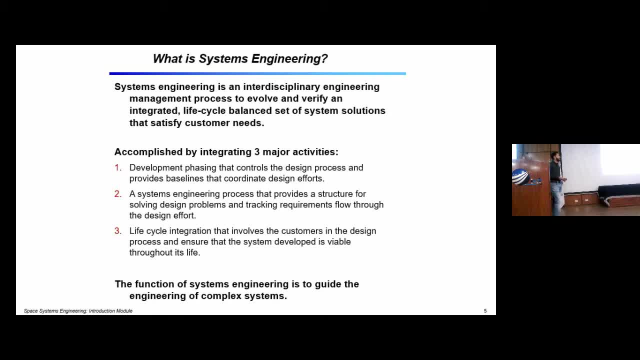 Then, after that phase of integration, we have the design phase. It provides a structure for solving different problems and tracking requirements through the design effort. and the third one is life cycle integration, which involves the customers or end user design process and it ensures that the system which is developed is viable. 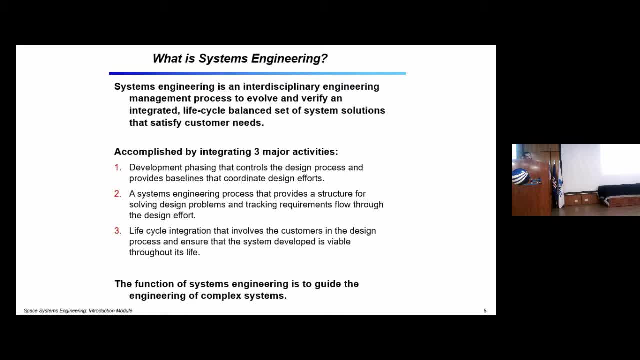 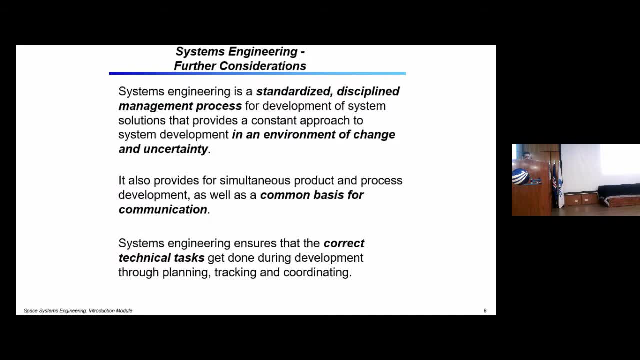 throughout the life. So the function of system engineering is to guide the engineering of complex system. There are some standardized discipline management process for the development of the system. So it provides simultaneous product and process development as well as common basis for communication. So this ensures that the correct technical tasks get done when 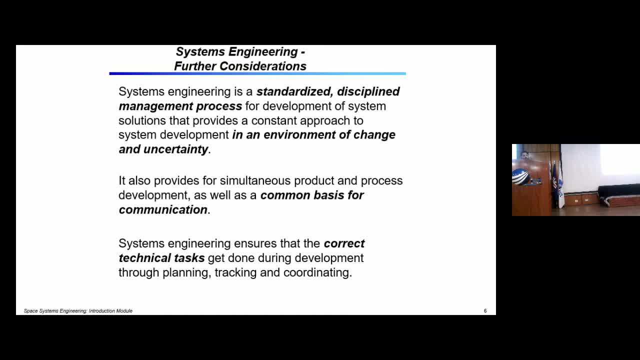 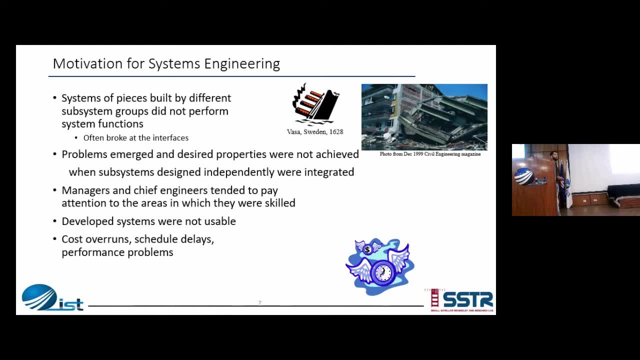 during the development, planning, tracking and coordinating phases. So what is the motivation for this systems engineering field? So, as you can see in this picture, this is a ship that was designed back in 1628.. So what happened? that the center of gravity of this ship was not in the proper place, so it sank. 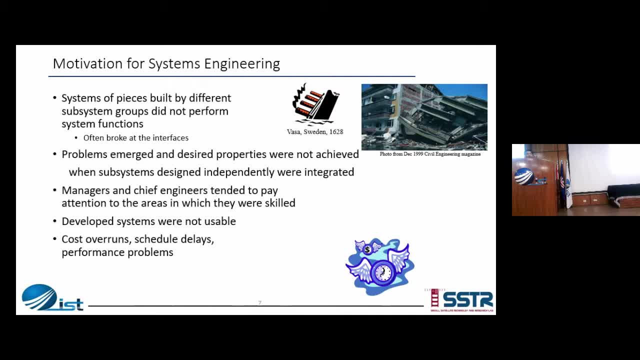 Similarly, this building- we can see it also destroyed at the point of integration or where the things were balancing. So these kind of integrating the things, that is an important aspect of the system. So the integration and the overall system understanding and development is an important phase in that. So what happens if the things are not initially designed or organized? 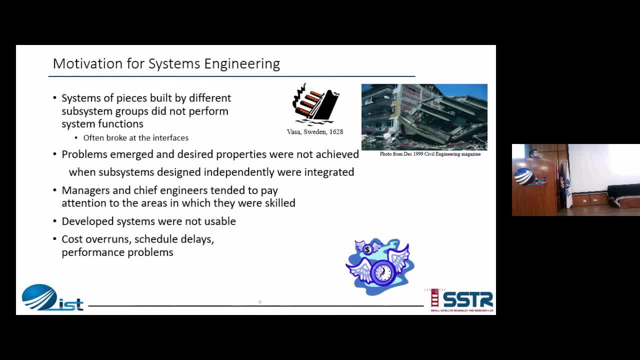 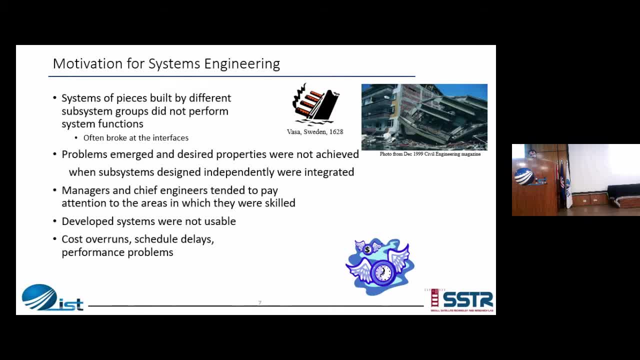 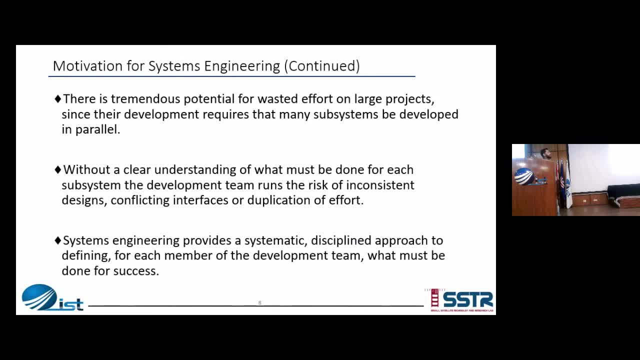 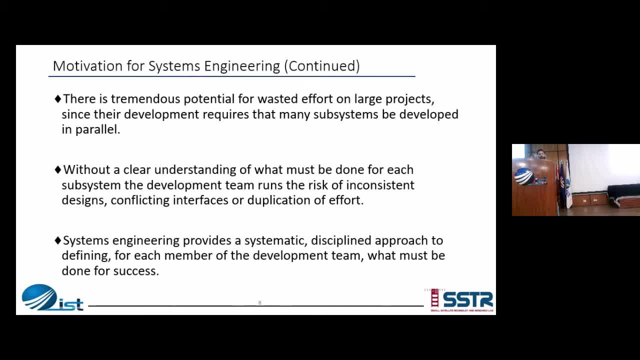 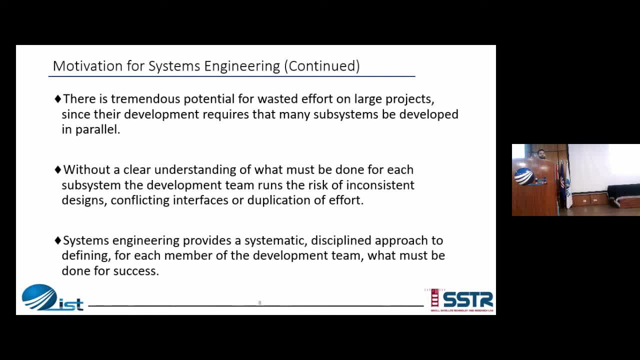 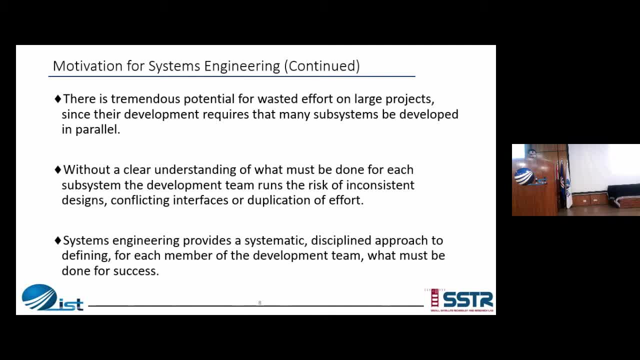 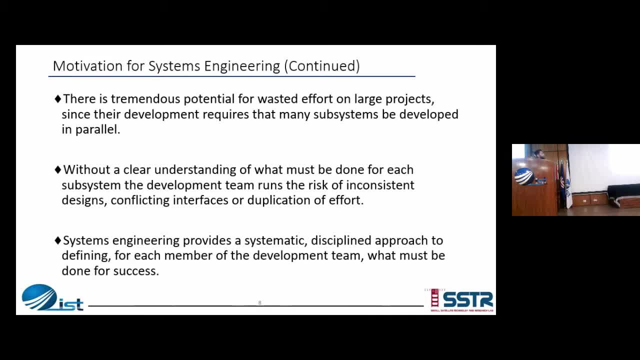 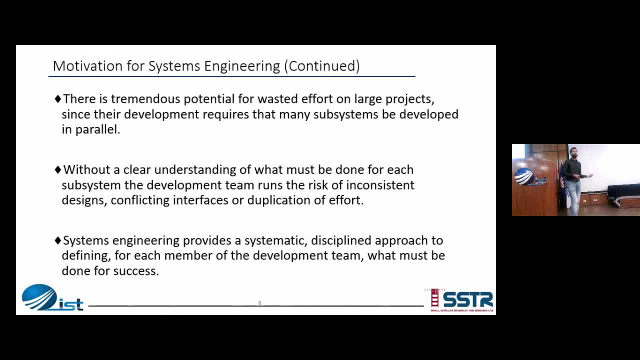 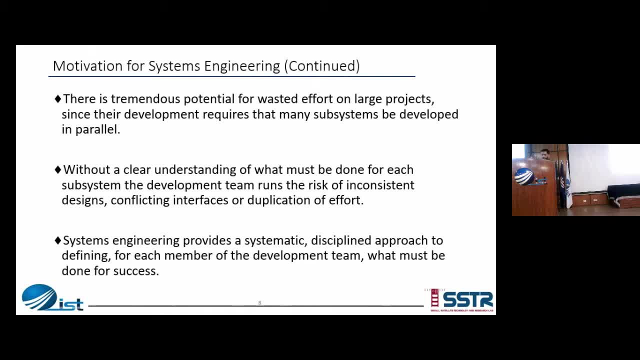 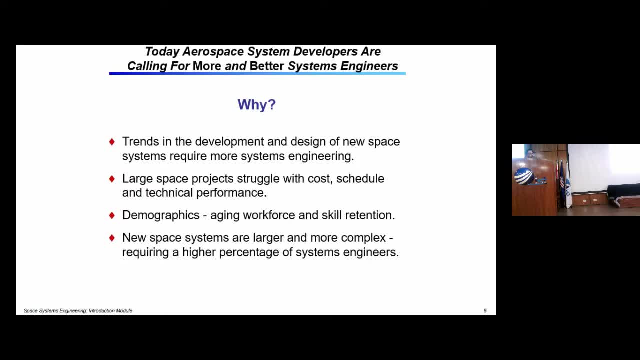 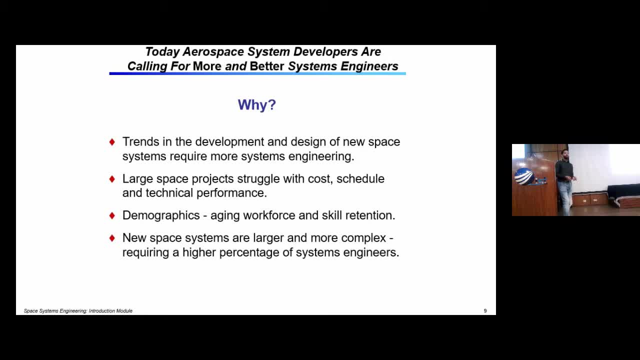 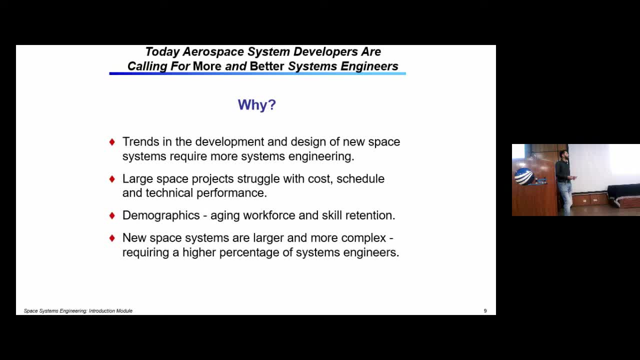 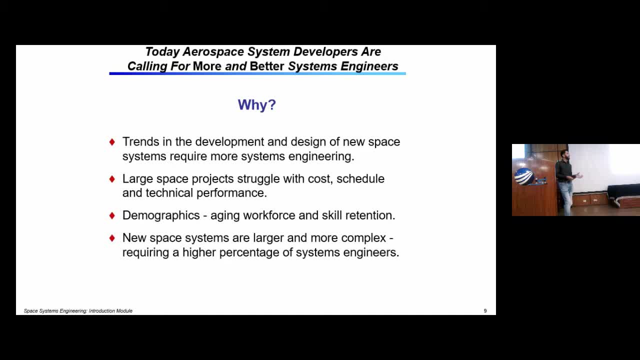 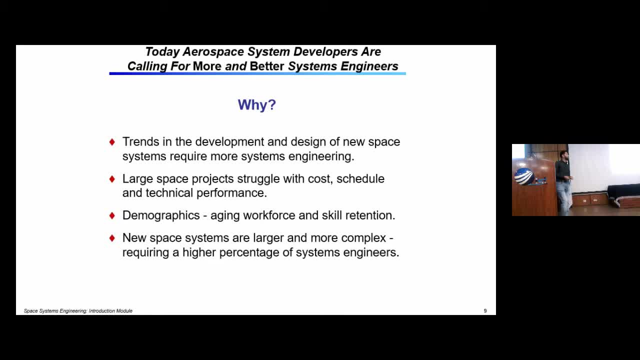 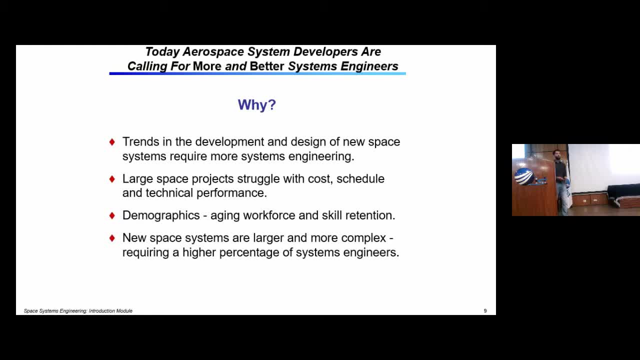 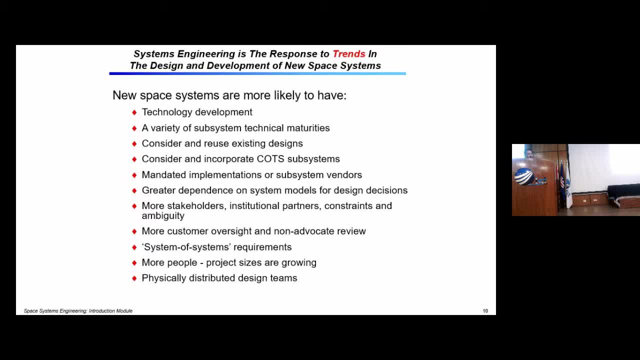 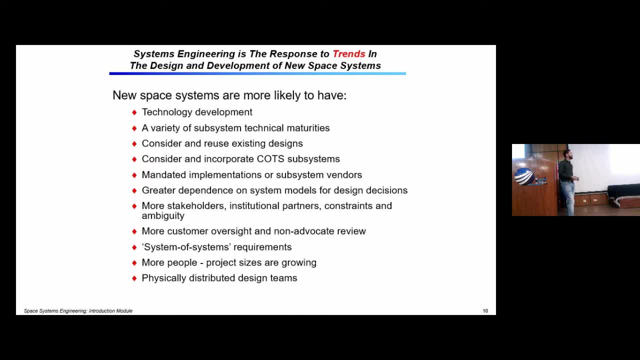 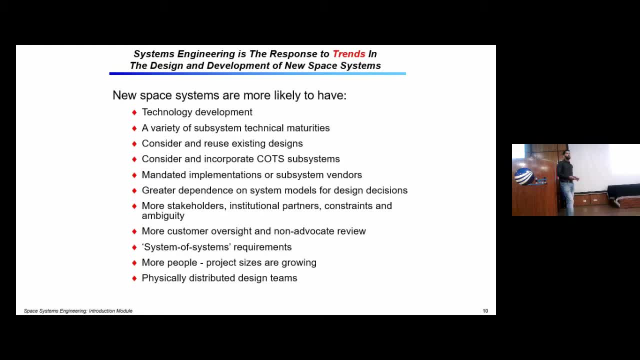 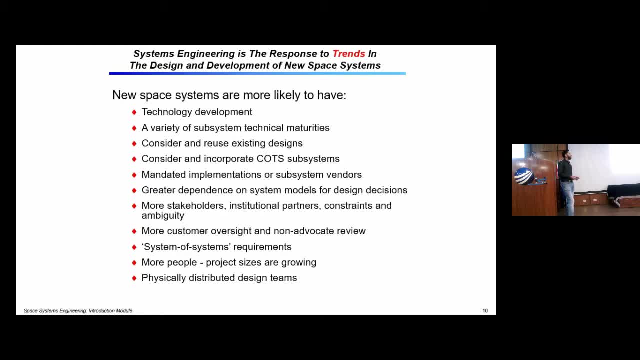 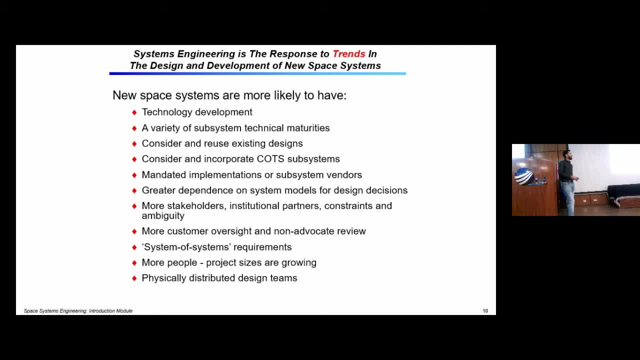 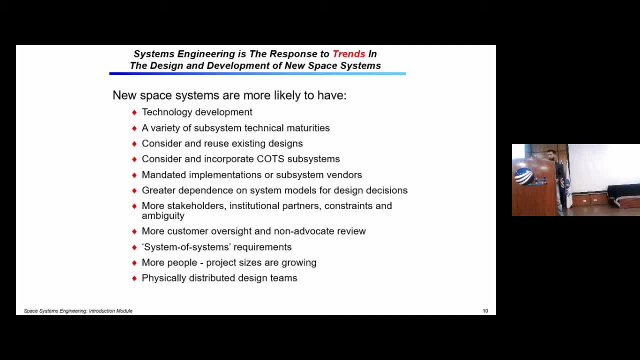 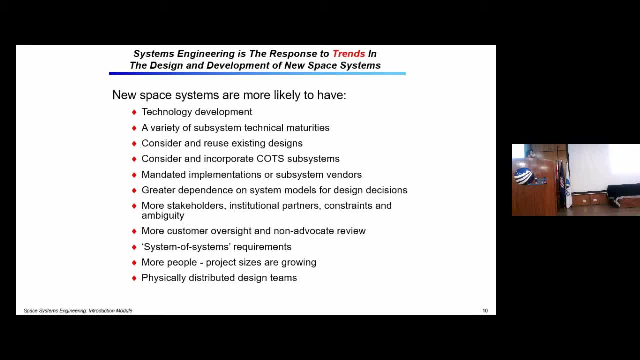 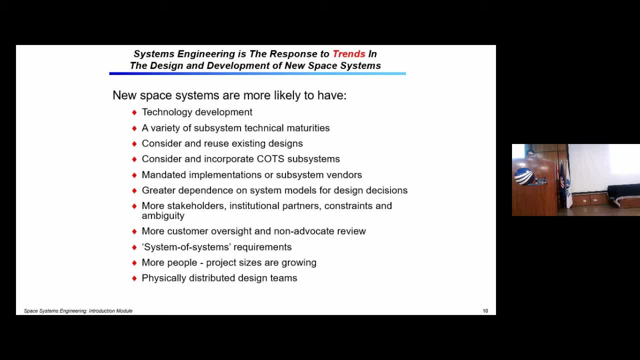 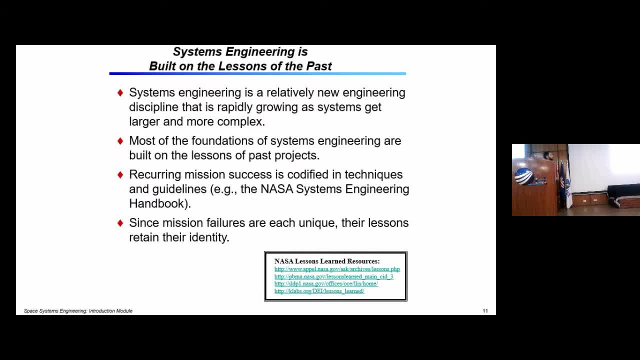 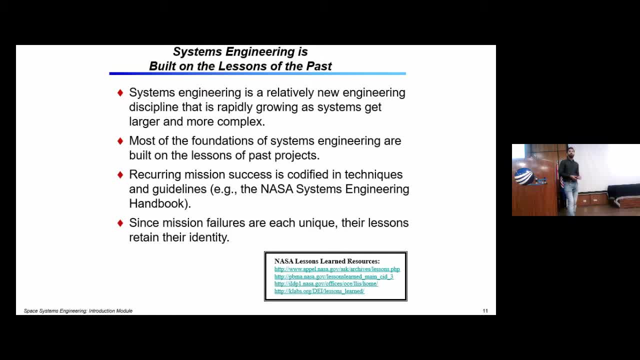 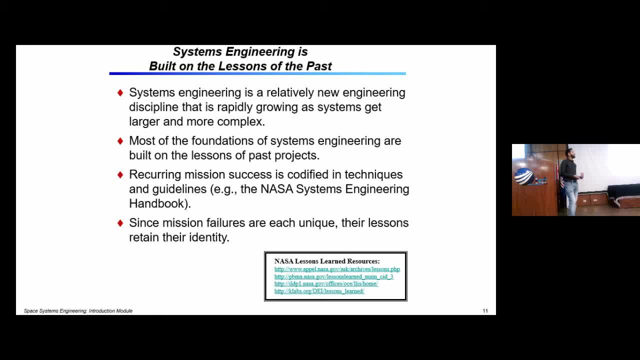 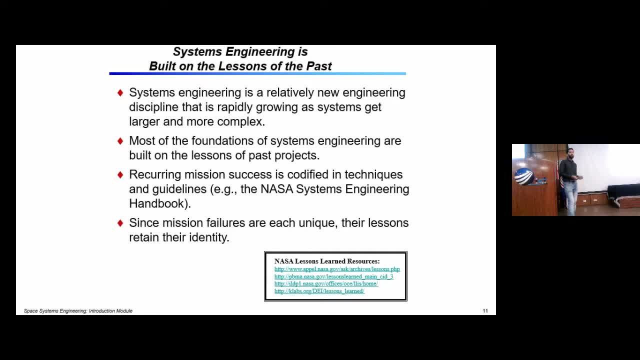 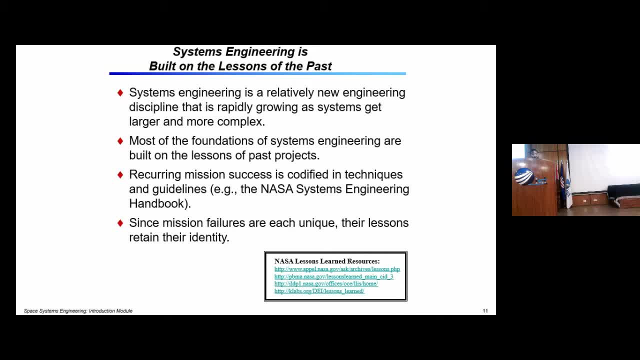 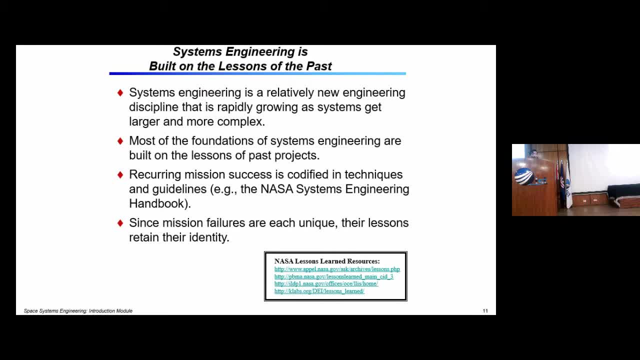 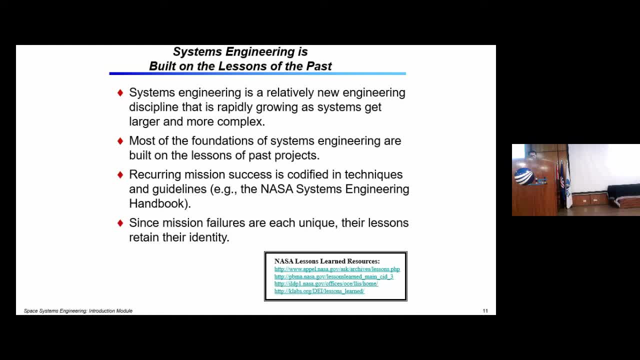 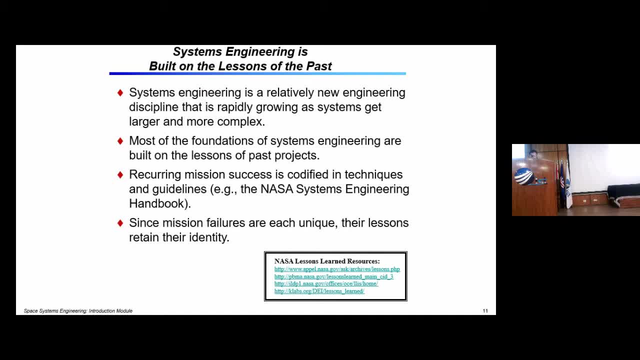 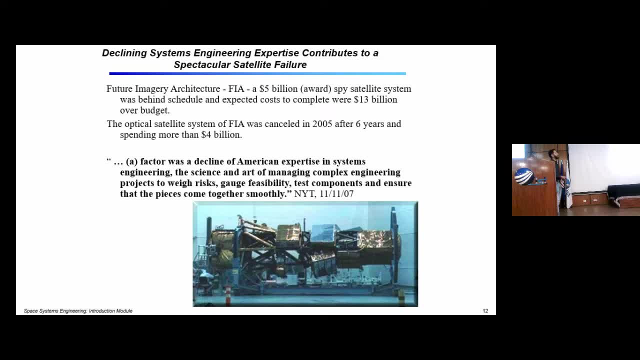 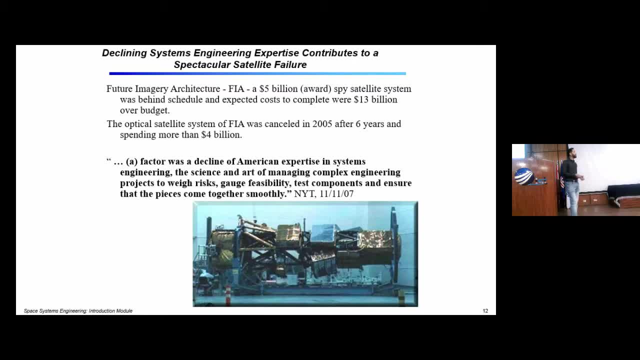 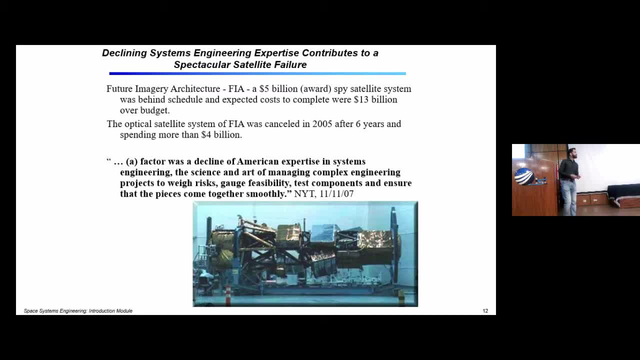 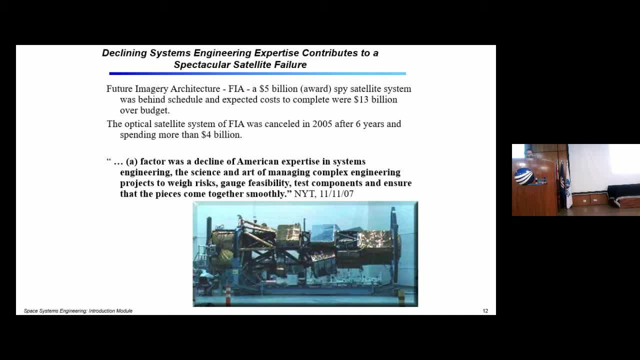 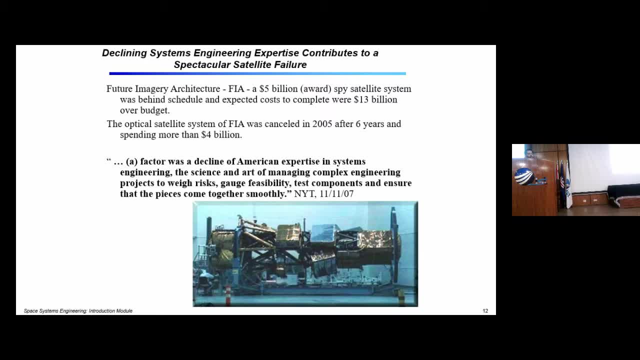 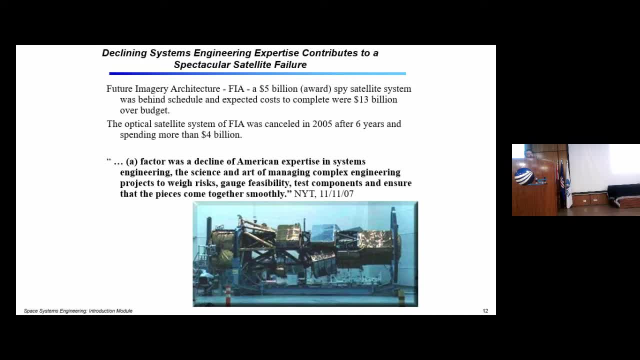 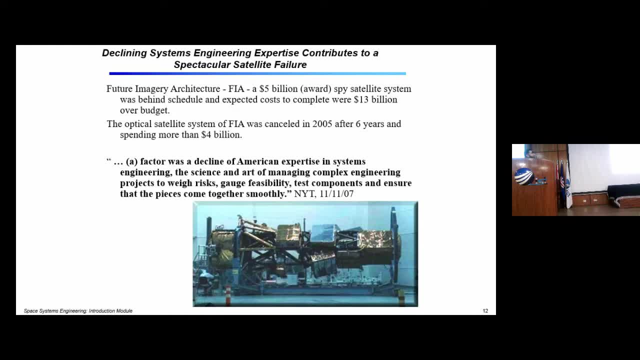 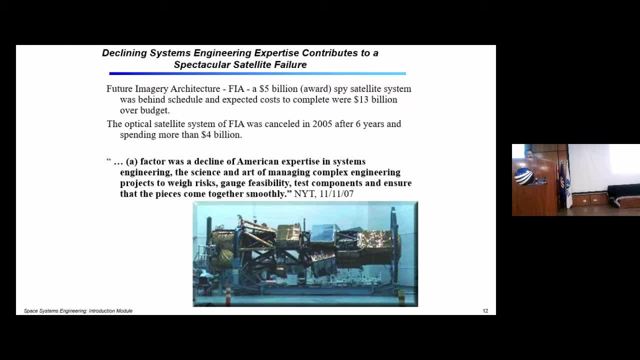 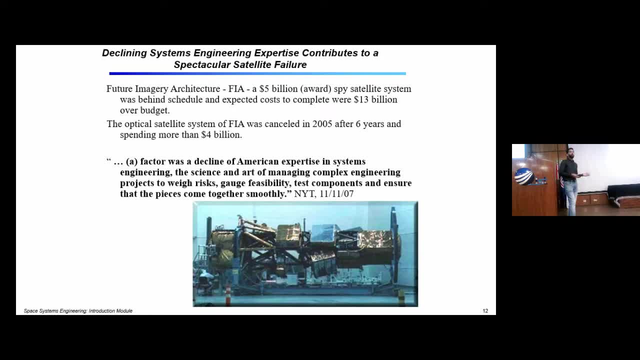 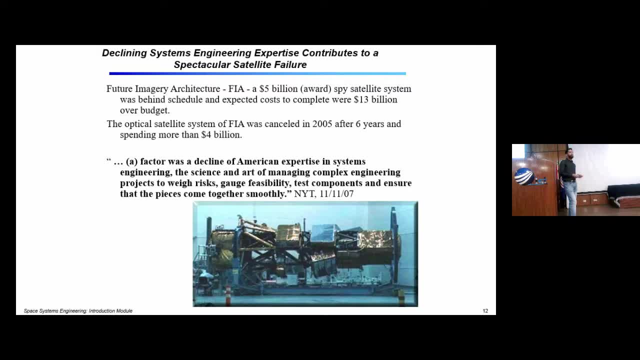 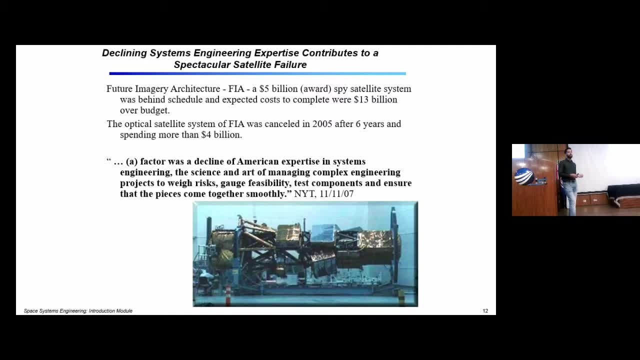 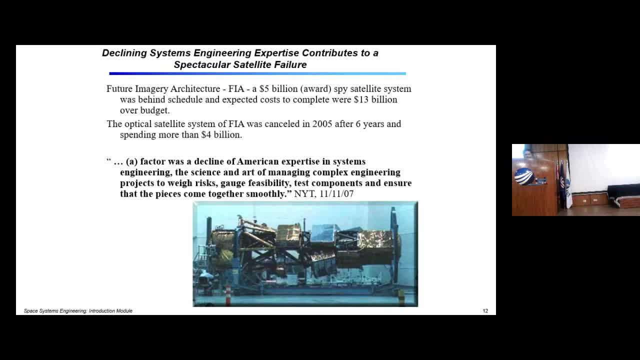 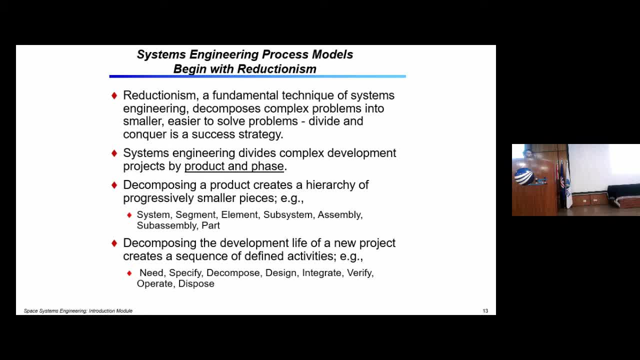 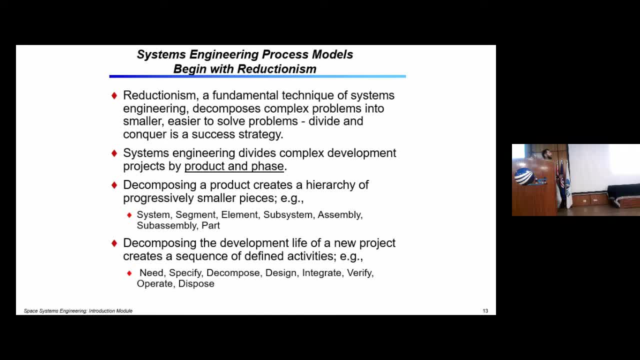 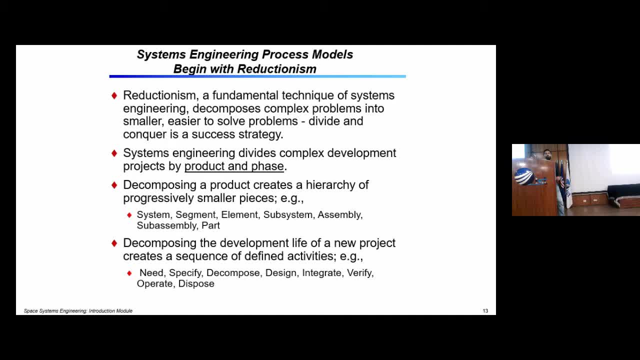 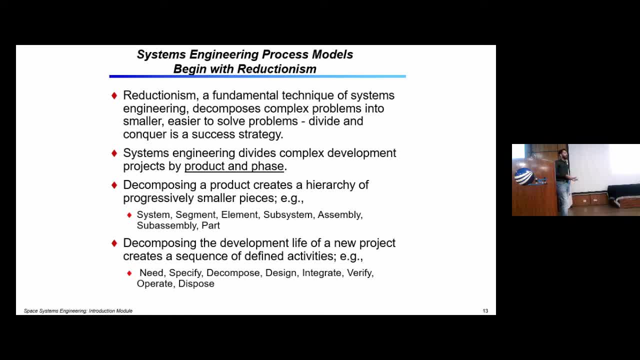 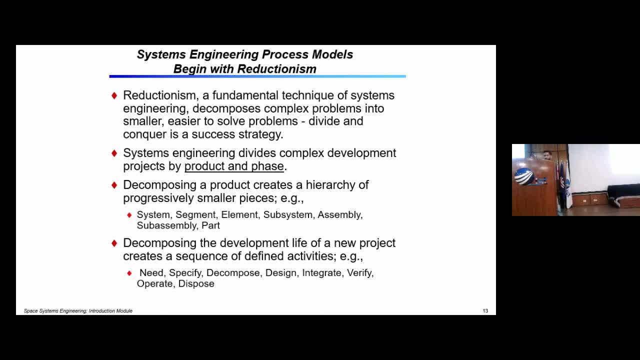 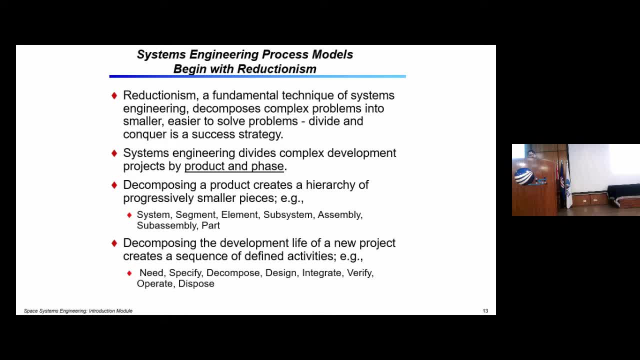 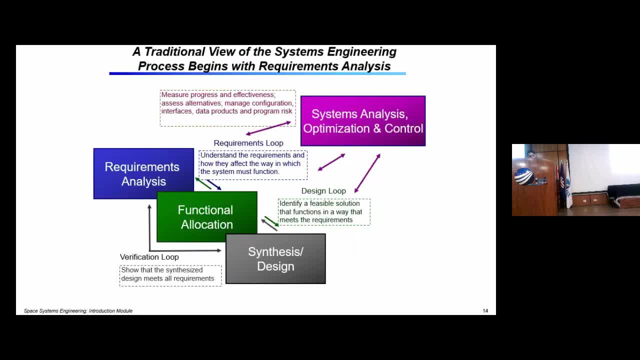 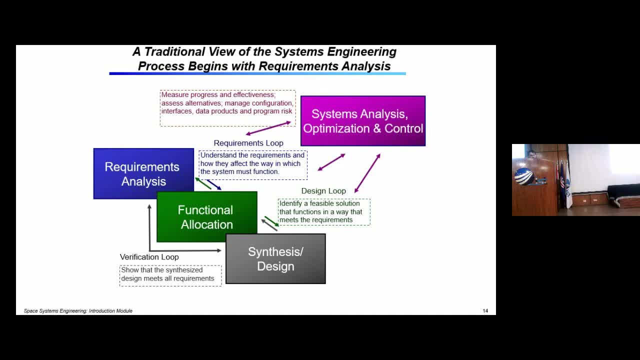 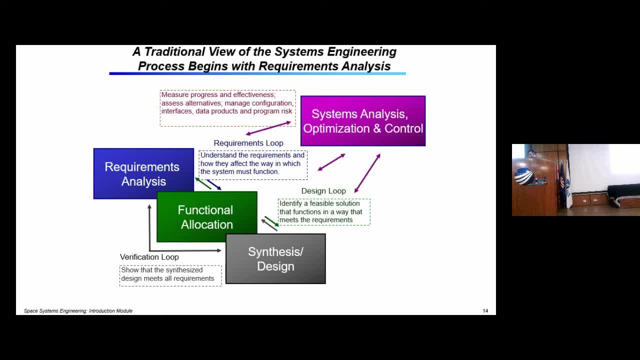 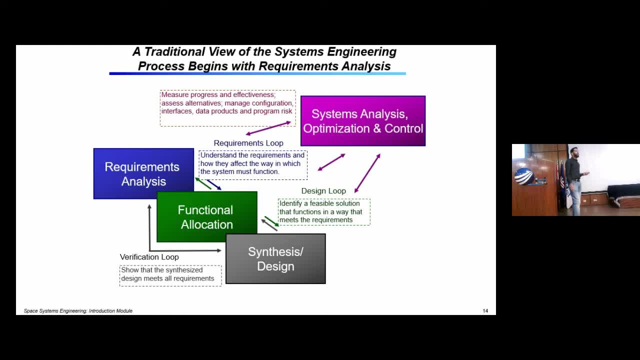 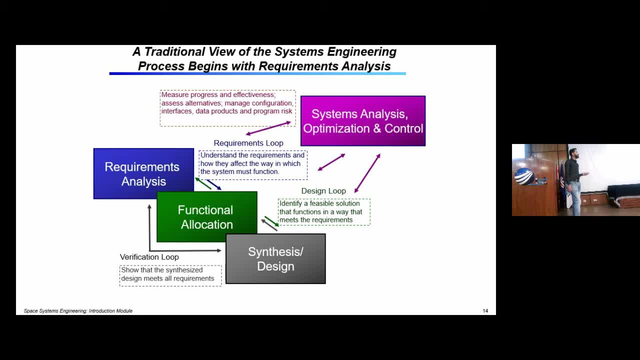 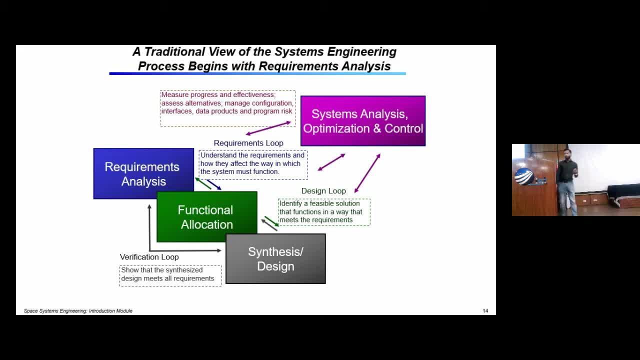 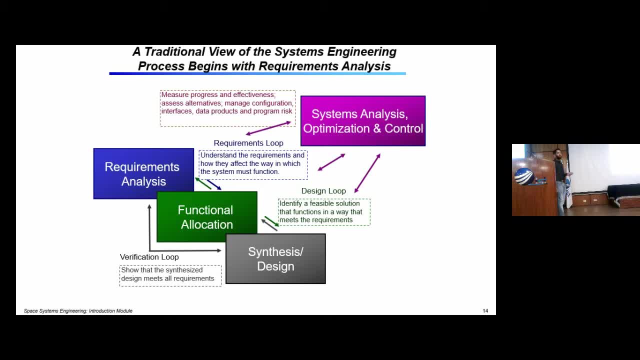 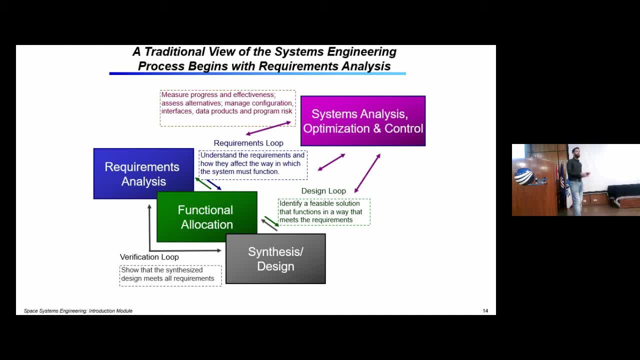 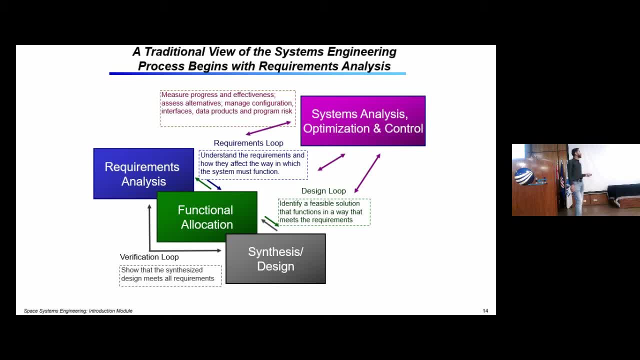 So the problems emerged in the later phases and the development system that could not be designed or organized. All of these things are interconnected and whenever there is some new requirement or new changes, so this all loops back and it continues until the final product is achieved. 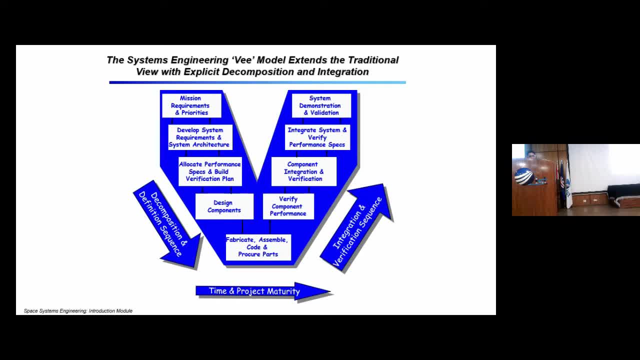 So this is also the process flow diagram, but it is in form of the V shape. There are different models, like the previous one was a traditional model block and this one is a V model, which is an extended view of decomposition and integration. And this also starts with the mission requirements. 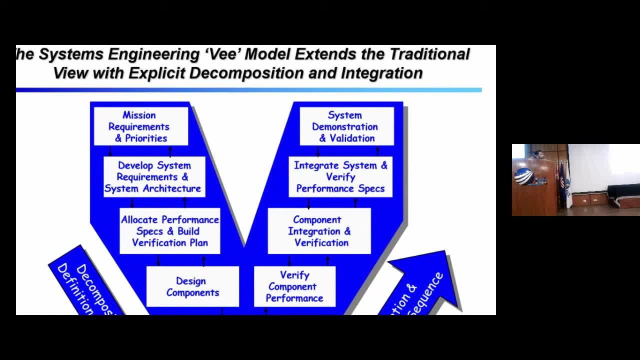 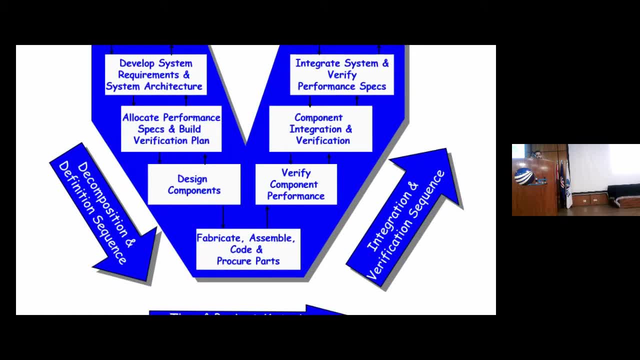 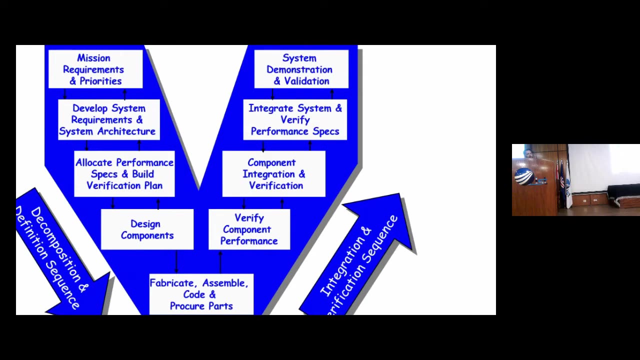 And then we have developed System requirements, a system architecture, and then there is a block for allocating performance specification. Then there are design components And then comes the fabrication or assembly, And then comes verifying and integration phase. so In this we have verifying the component performance and then integrating them. after that we demonstrate and validate our system. 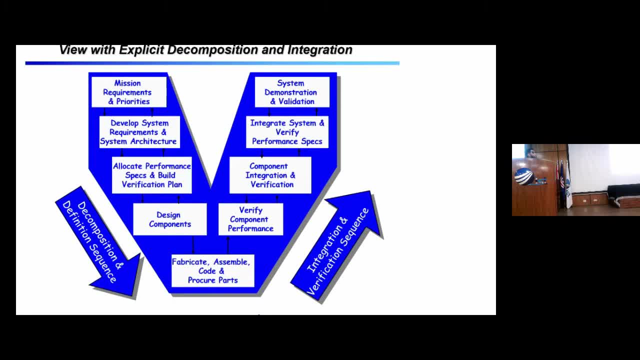 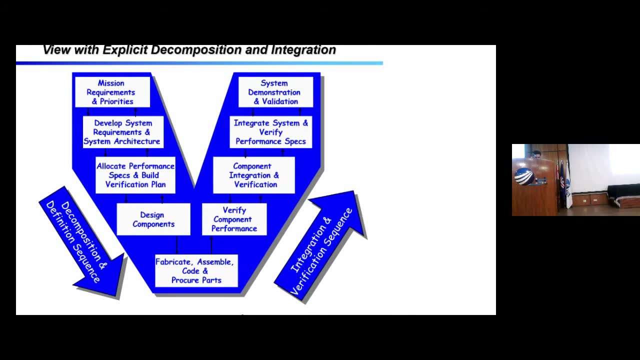 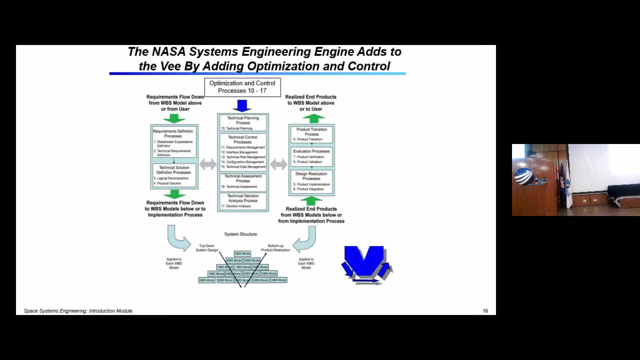 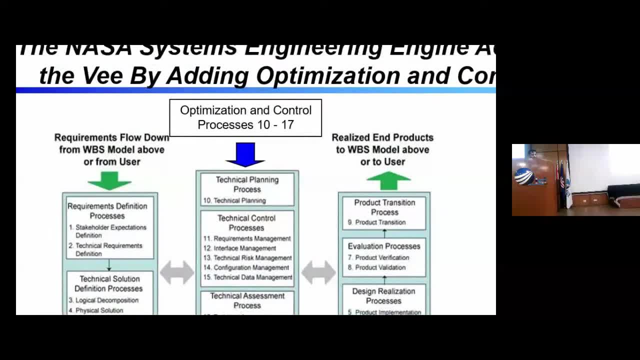 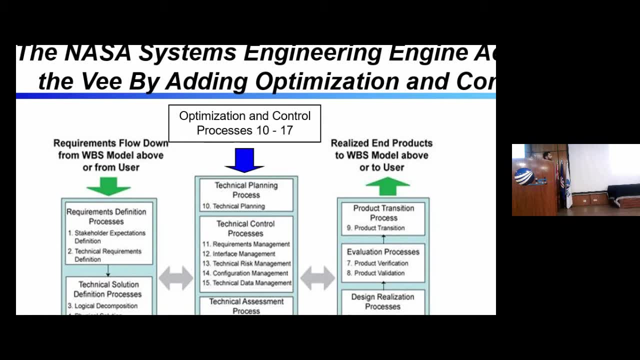 So, So, So, So, So, So. Okay, The last slide. we discussed about the V model, So this is the advanced or optimized version of that. So in this one they added optimization and control process, which are from number 10 to 17.. 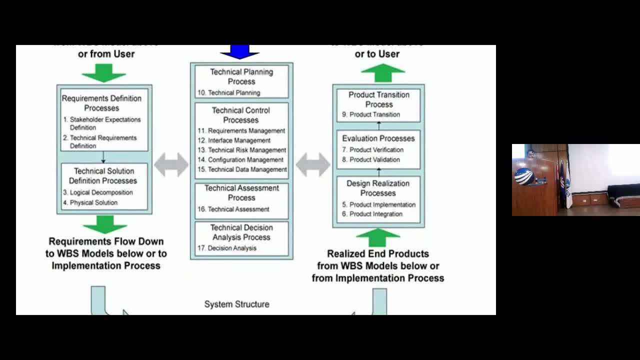 If we look at them individually- So in the previous- we just see the whole blocks of requirement and development and integration. So if we see them individually, we have The, The Stakehold, Stakehold, expected definitions in the requirement, Then we have technical requirement definition. 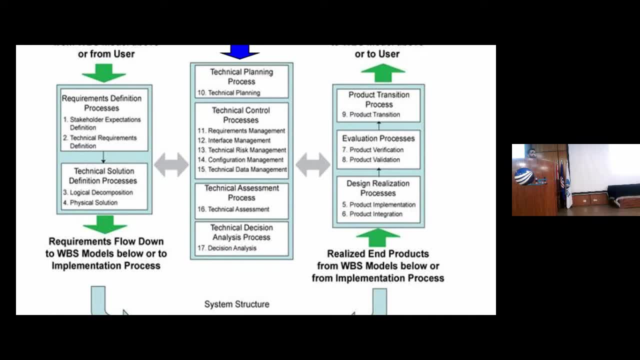 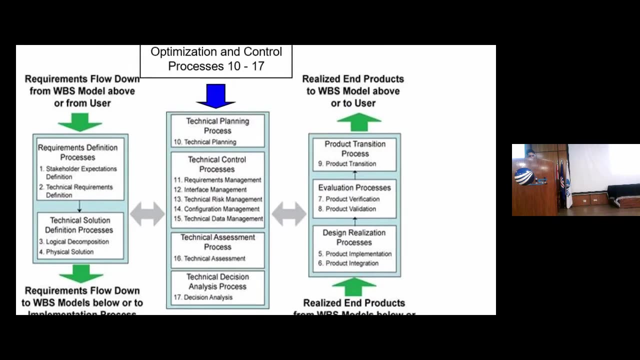 So all these things are in the requirement definition process, which was a whole block in the last slide, Then the next one, three or four. These are their technical solution definition process, which consists of logical decomposition or physical solutions, And after that we have design realization process, which are at number five and six. 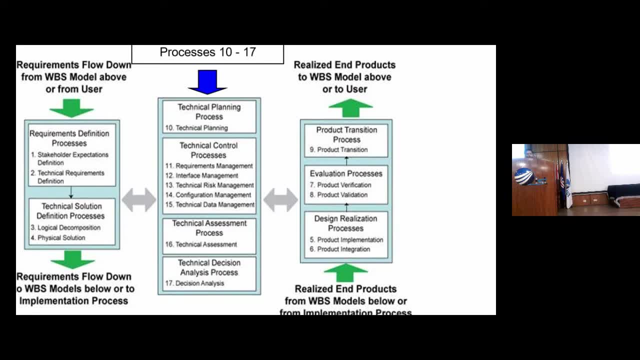 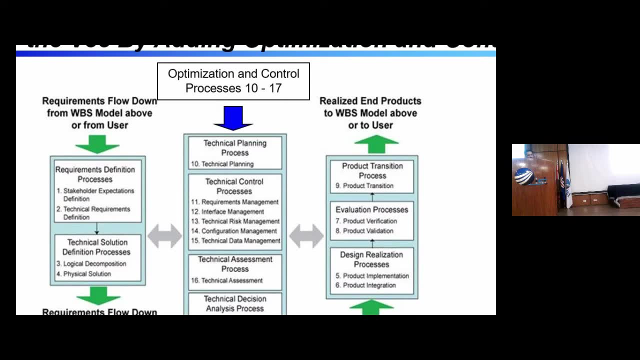 And we can find that here And we can find that here- six, So it consists of product implementation and product integration. And then there are seven, eight, which are product verification and product validation, And on the nine we have product transition And the numbers which are in the 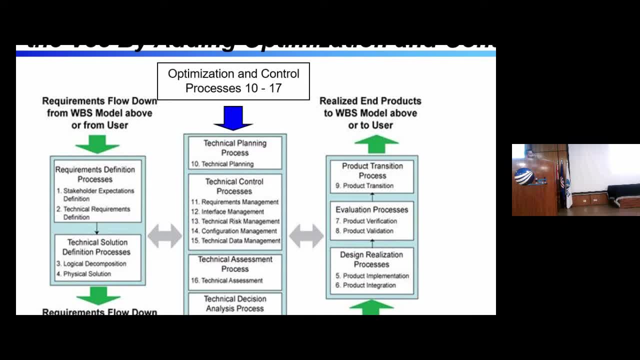 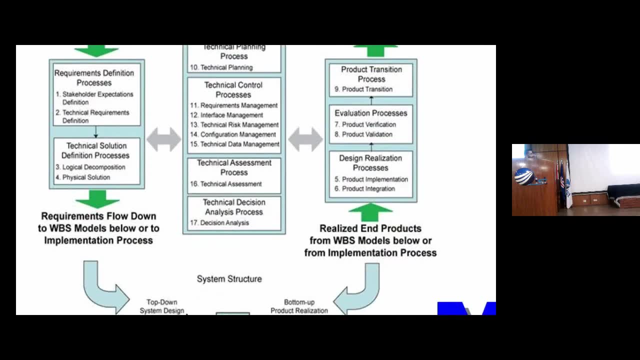 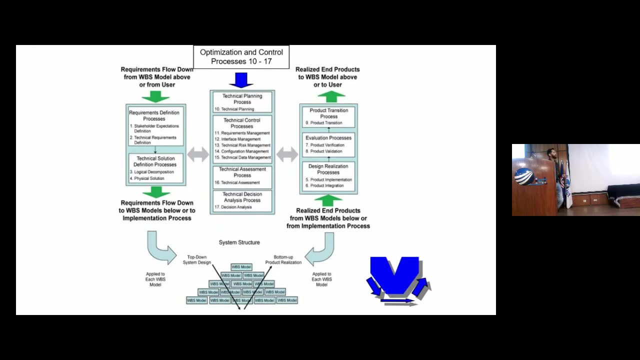 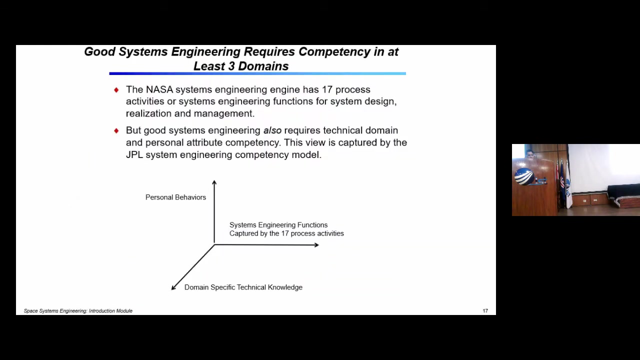 optimization and control process. it consists of technical planning requirements and management, configuration management, technical data management and then decision analysis. So this was the V diagram, And this is an extended or exploded view of the dead V diagram, which demonstrates and describes the whole system engineering process. So the good. 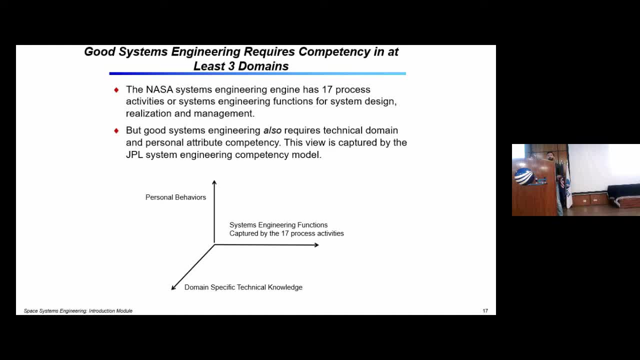 system engineering requires competency in at least three domains. So what are those three domains? This consists of personal behaviors, domain domain, specific technical knowledge and then system engineering factors. So these 17 process activities which are discussed in this model, this slide. So the good system engineering model must have. 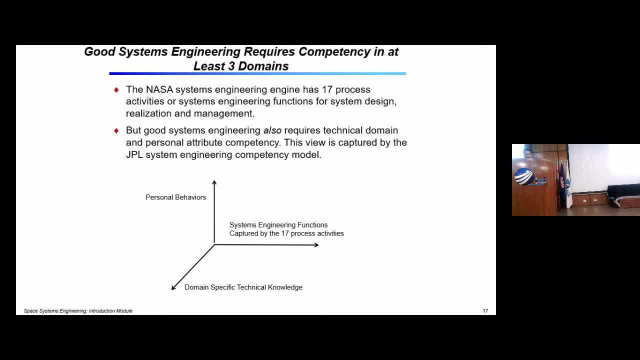 knowledge about these 17 activities And the personal behavior. it consists of team management, team leadership, developing and distributing tasks between different team members. So all these things comes in the heading of personal behaviors. It also consists of attitude, communication, your intellectual and self confidence. So all 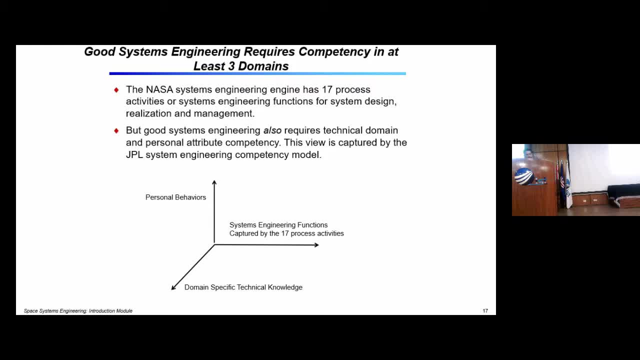 these things comes into the heading of personal behaviors And the domain related specific technical knowledge. it consists of data system engineer must know about, maybe guidance, navigation and control, or if they are designing some microcontrollers or onboard computers. So they must have know how about all of these overall subsystem propulsion? 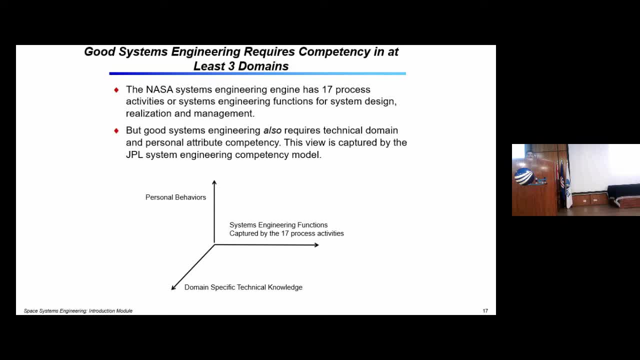 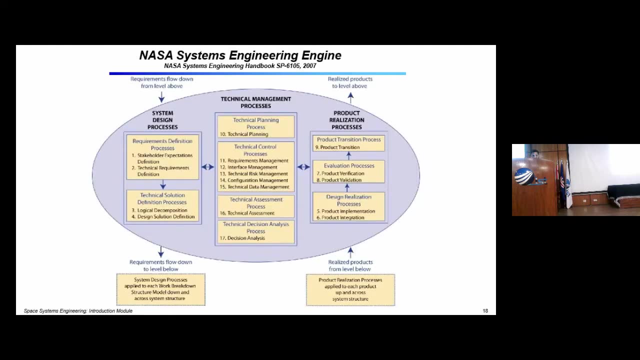 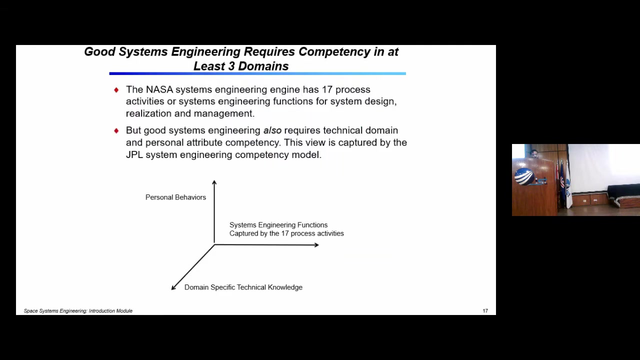 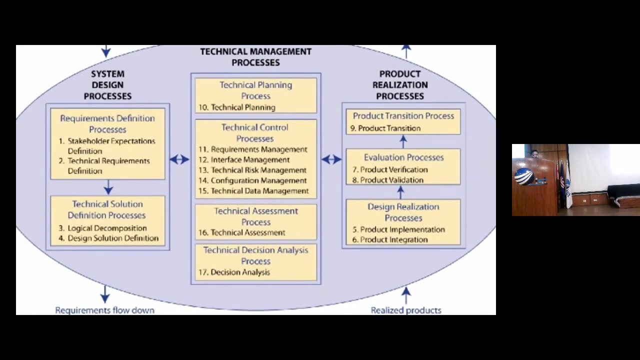 systems software engineering techniques. So these three overall combinedly create a good system engineering domain. So these are the 17 process. These are also mentioned in this added optimization block diagram and it is also in this one. This is taken from NASA system engineering handbook. So if you 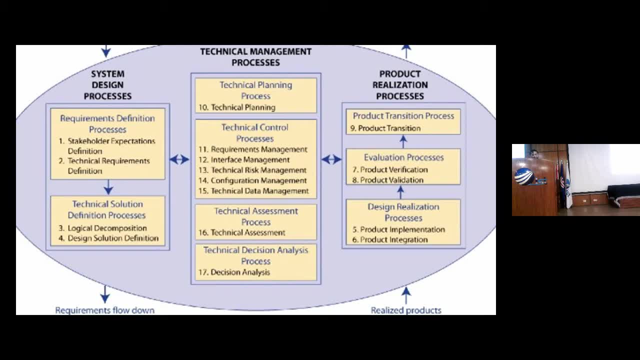 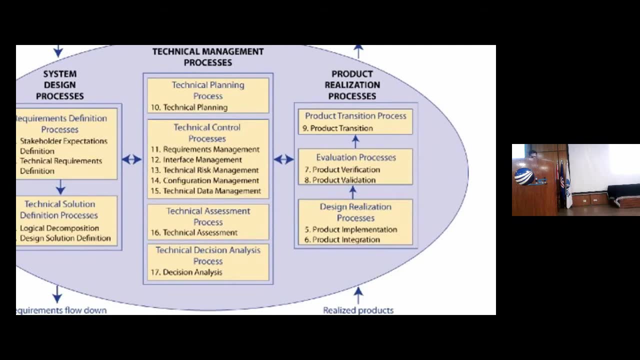 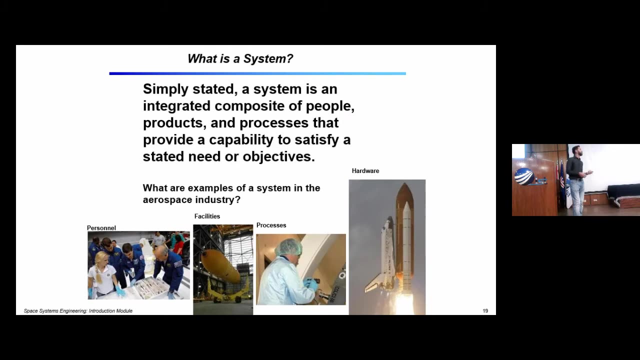 look at this. These are the 17 points which we were discussing about in the last slide, So we already told you about these before. So, moving on to next one, What is a system? So, simply stating, a system is an integrated composite of people, product and processes, And we utilize those. 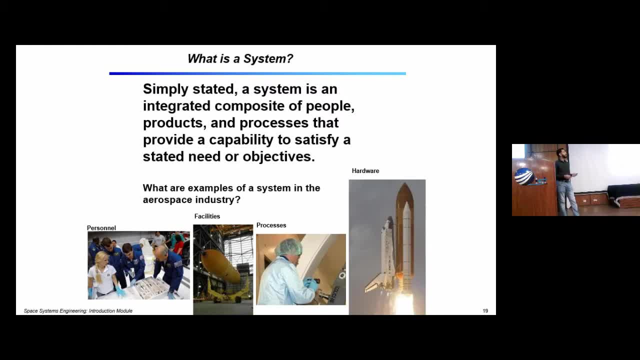 capabilities and develop our or achieve our end objective. So this is basically a system. So there are some examples which are shown in these figures. So these are the team members, facilities, processes. This is a hardware. So overall, all of these make a system. 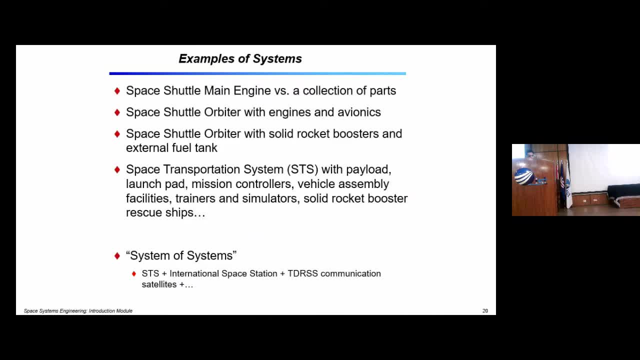 So these are also examples of a system: Space Shuttle main engine versus collection of parts. Space Shuttle orbiter with engine and avionics. Space Shuttle orbiter with solid rockets. Similarly, space transportation system with payload, launch pad And then system. So and then there is. 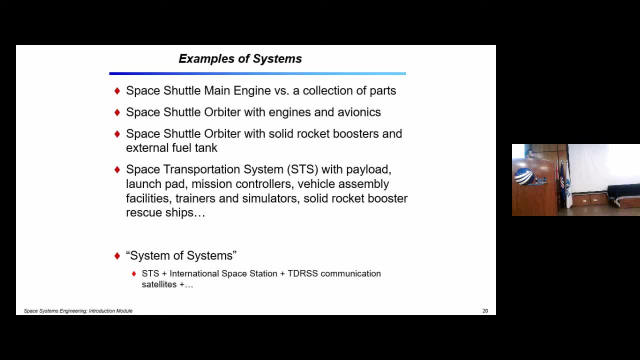 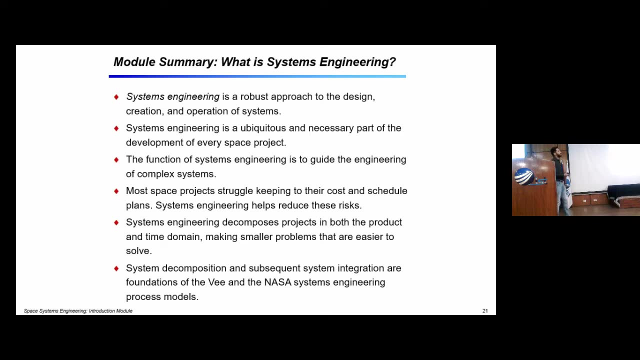 vehicle assembly facilities, trainer and simulators, solid rocket boosters. So all these are examples of these systems. So summary: this slide discusses about overall summary what we have discussed so far. that what is the systems engineering? So basically, it is a robust approach to designing, creation and operation of systems. 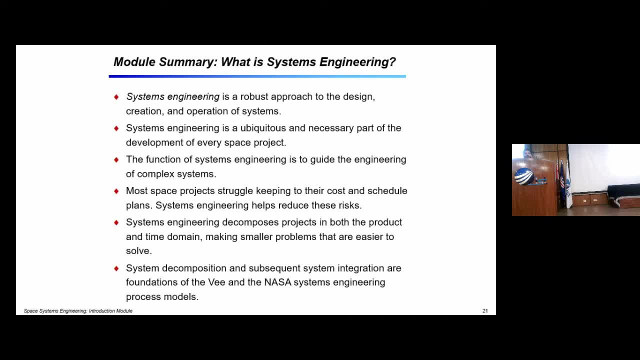 So necessary parts And development of every space project is carried out using that, And the function of system engineering is to guide the engineering of complex systems, And most space projects struggle keeping up with their schedule because of this, if they don't have efficient or 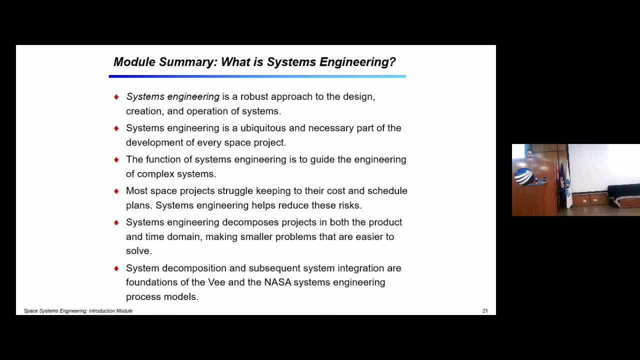 efficient time domain system. so they will let the schedule. Similarly, system engineering decomposes project in both the product and time domain System decomposition and subsequent system integration or foundations of the and as a system engineering process model. So this is also. the 17 points are which are taken from system engineering handbook. 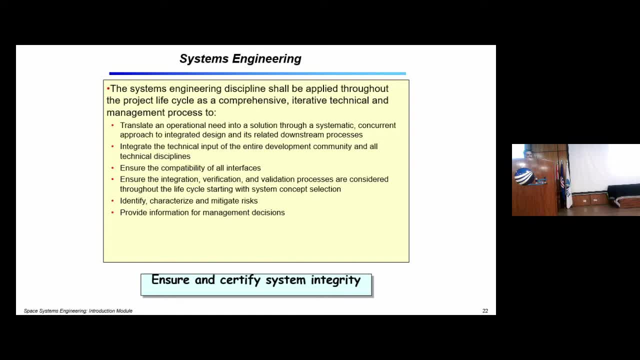 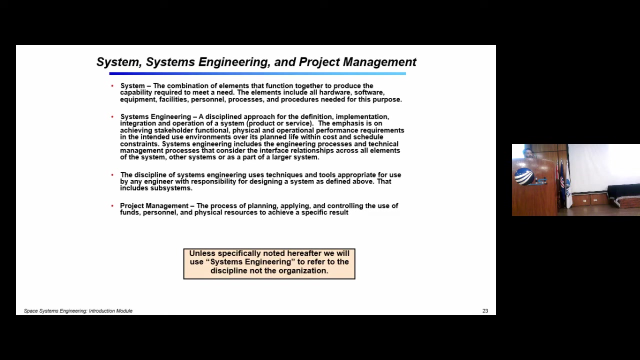 So the system engineering discipline shall be applied throughout the project lifecycle and it is iterative, technical and management process. So this in shape We have seen, This ensures and certifies overall system integrity. The project management- okay, the process of planning, applying and controlling the 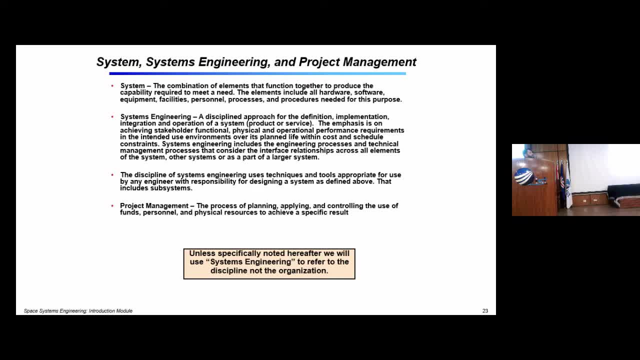 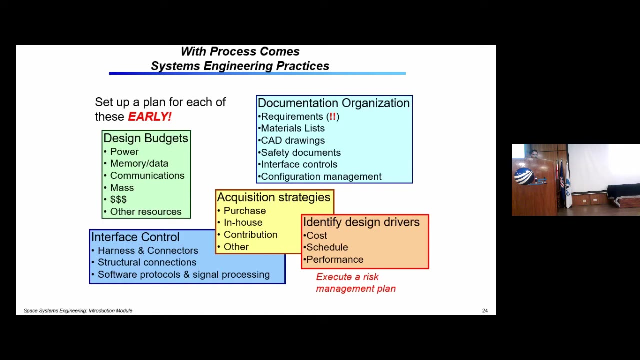 use of funds, personal physical resources to achieve a specific result. So we have discussed about systems, systems engineering. So the project management is overall management of all of these resources, The physical person, HR and overall team. So this block shows the further sub subheadings which are considered in the system engineering. 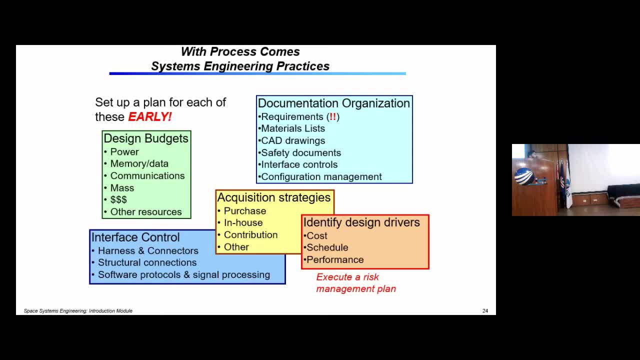 practices. So if we look at the green block, it consists of design budgets. So what we do in design budget is that we describe our power memory requirements. Similarly, we have the communication systems or protocols. then we define mass budgets. So we define our limitations or our requirements in this design budget phase. 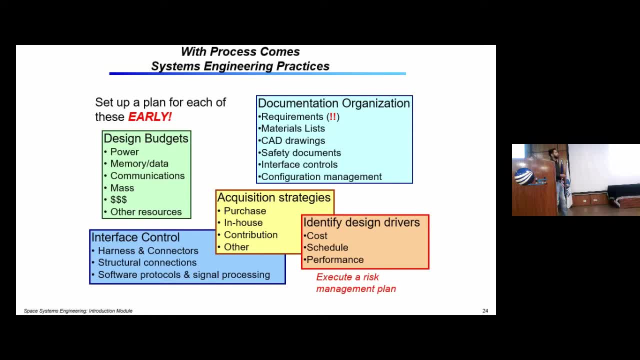 Then we have interface control, So it consists of the physical structural connectors and the software protocols and the signal processing techniques that will be used. Okay, so let's continue. And after interface control, We have this document organization. So documentation is also an important part of the project. 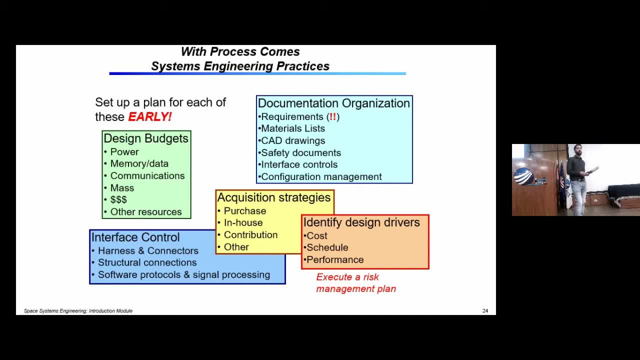 So what happens is that whenever in the HR team, if we don't have efficient documentation, so when that team member leave your, so there is a gap in the communication or our requirement fields. So the efficient documentation helps achieving those goals. So in documentation we should always document our requirements. 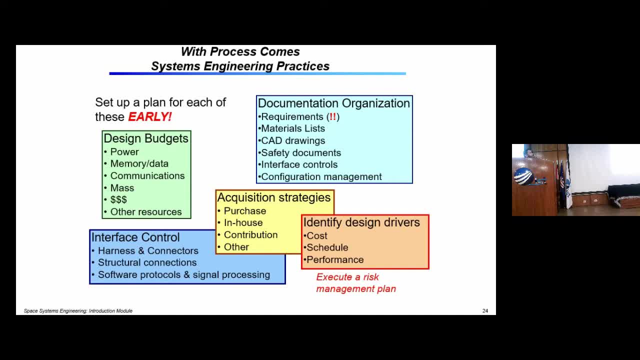 Materials, the CAD drawings, similarly safety documents and interface control documents. So all of these should be documented properly. Then we have acquisition strategies. In acquisition strategies we have to decide that whether we would purchase some parts or we would have in-house development or we would have collaboration. 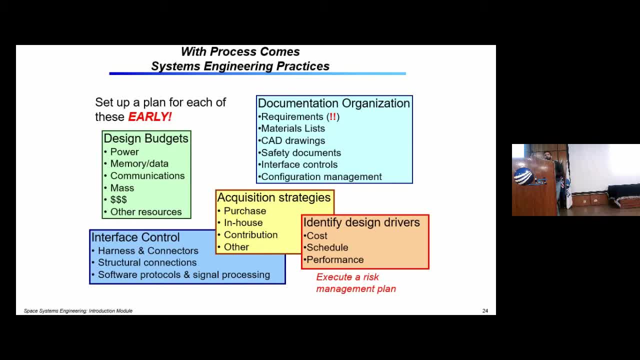 Or maybe there is a problem, So we have to decide that. Or maybe there is a combination of all of these things. We purchase some parts and we also develop some parts, And then we have to decide these design drivers. We have to identify our cost schedule and performance. 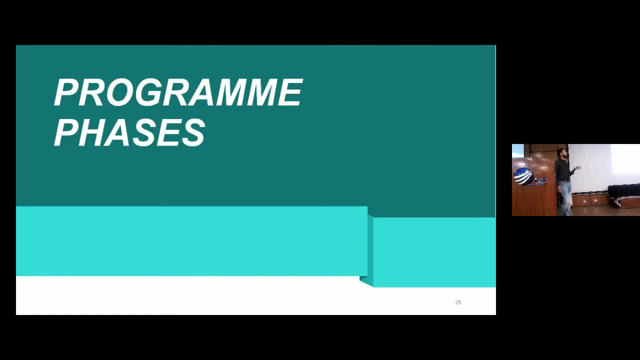 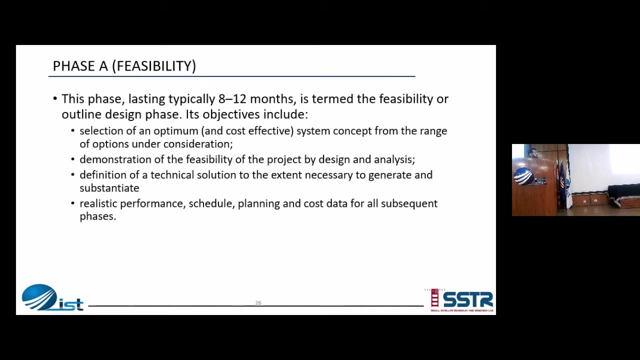 So this was the previous session. the previous module was about the introduction of system engineering. Now we will have a look into the different- Okay, Different- phases of system engineering. The first one is feasibility. So usually these things are for the large projects, but when we are dealing with some, 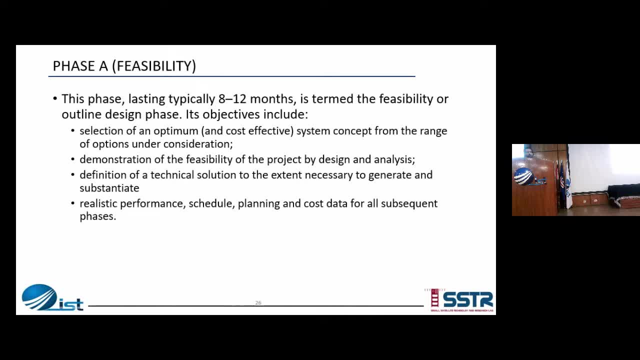 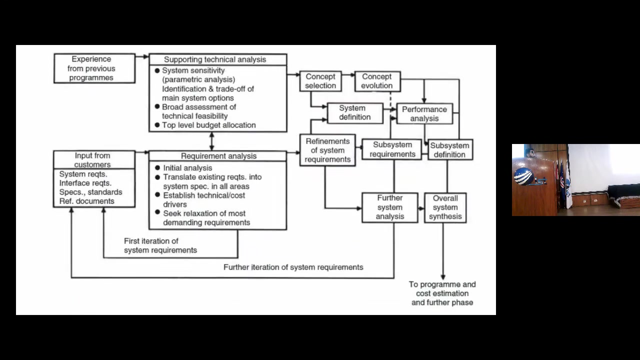 small projects like the CubeSat development. So these time that I mentioned here it would differ, But the first thing that was considered in every case is the feasibility. We decide our optimum requirements And then we demonstrate the feasibility of project. Then we have schedule, planning and cost data for all of our systems. 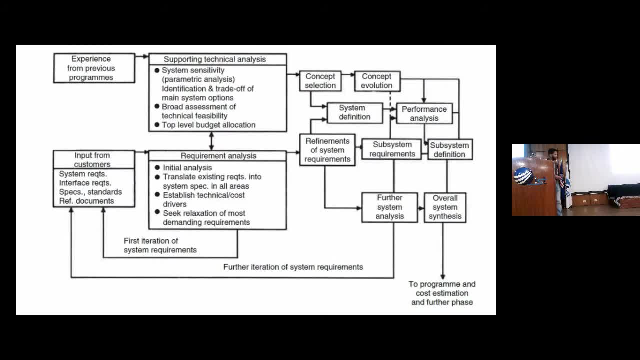 So this is a block diagram for the feasibility thing, The first one. we have some input from our customers, So this is really one block is this one, And one is this one And one is at the bottom. So in the lower line we have input from our customer in which we have system request. 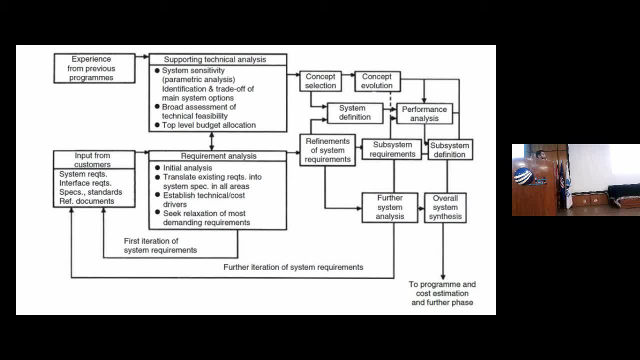 system requirements, interface requirements, And then we analyze those requirements, which consists of initial analysis, establishing technical or cost drivers, similarly seeking relaxation of most demanding requirements, And in the upper one, we have supporting technical analysis, Which consists of systems and a sensitivity, or the parametric analysis of the system. 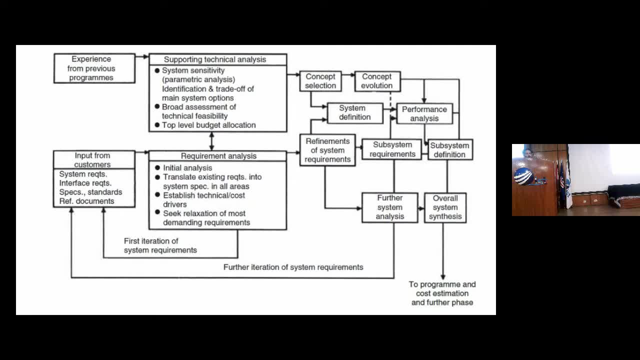 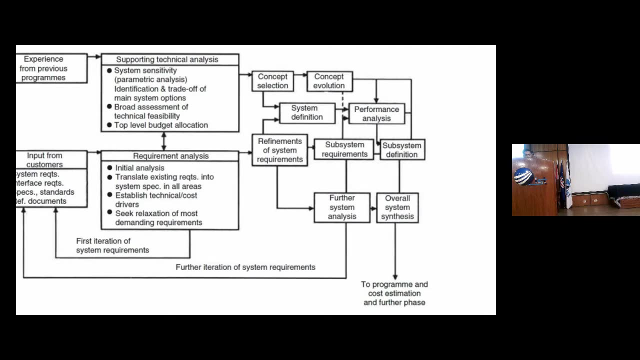 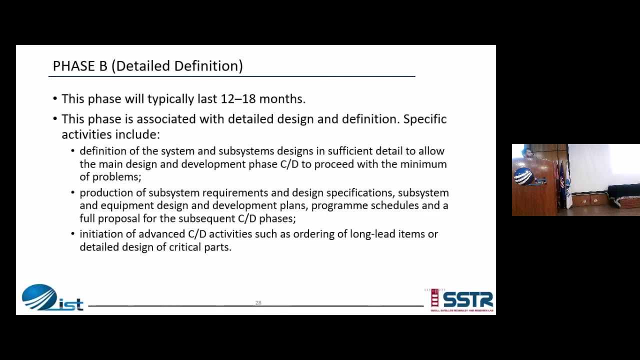 Similarly top level, budget and location, and all of these are connected further to different system definition and performance analysis modules And in the end we have to program and cost estimate our overall system. Okay, So the phase B, which is the next phase. this also according to different project. 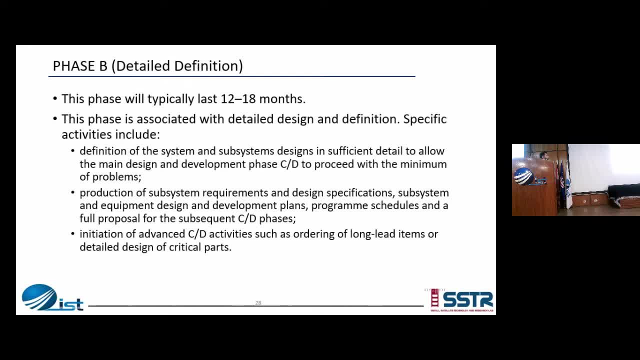 we have to design it during the design phase. So this phase is associated with the detailed design and definition. So the specific activities that are included in this phase are definition of the system and subsystem designs, Similarly, production of subsystem requirements and design specification. 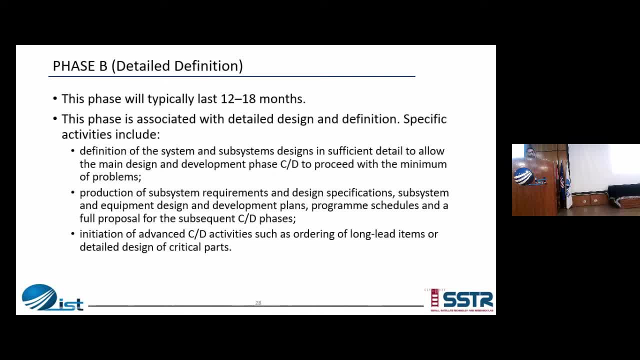 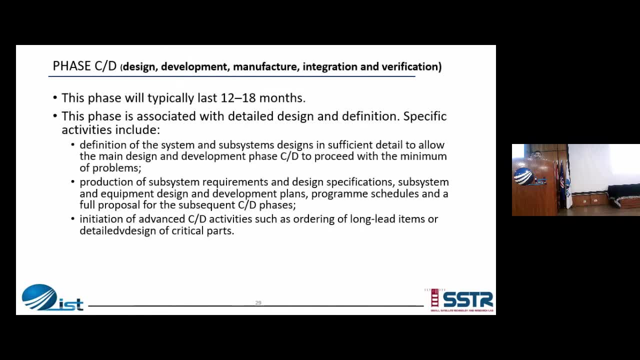 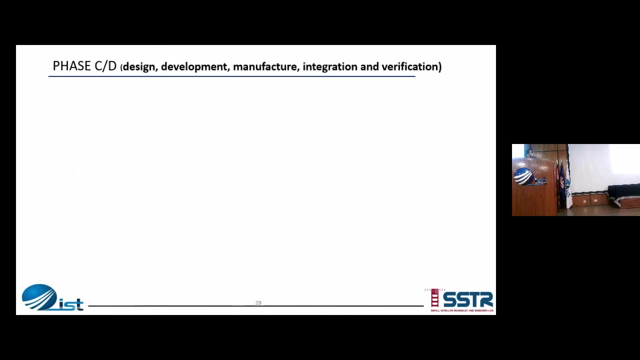 And then we initiate our C and D, which are the next phase. C and D: these phase consists of development, manufacturing and integration of the system. So in the phase B we have detailed definition about the system. Similarly, phase C, we have design, development and integration. 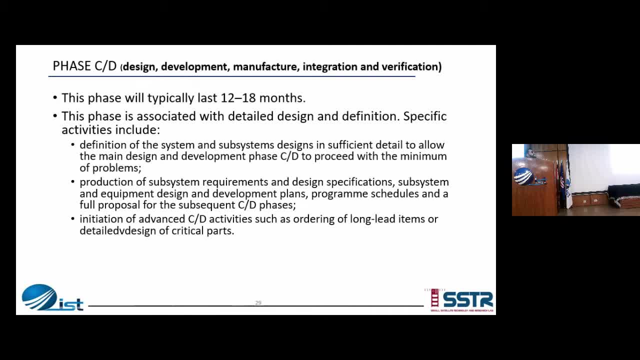 So the initiation of C and D, which are the next phase. C and D phase: we identify our parts and components, then we assemble or manufacture them, Then we integrate them. So after this C and D phase we move on into the and also there is a technology readiness. 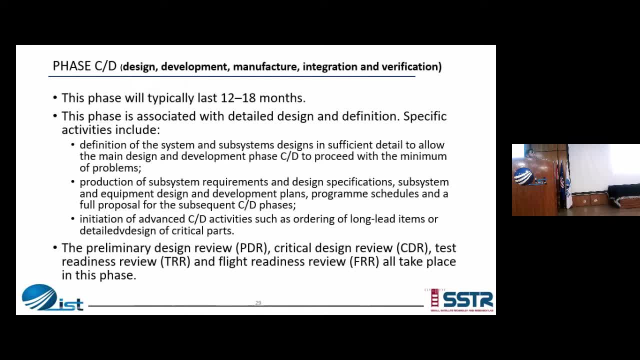 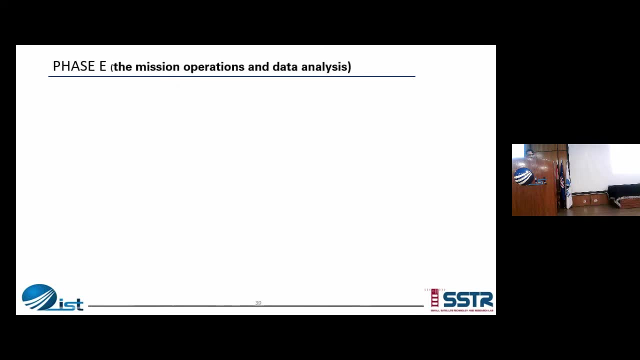 level and some other parametric definition like flight readiness review. So these are the systematic ratings which are kind of standardized, and when we develop our product We determine it is based on which level of those reviews. So the next phase, which is phasy, it consists of mission operation and data analysis. 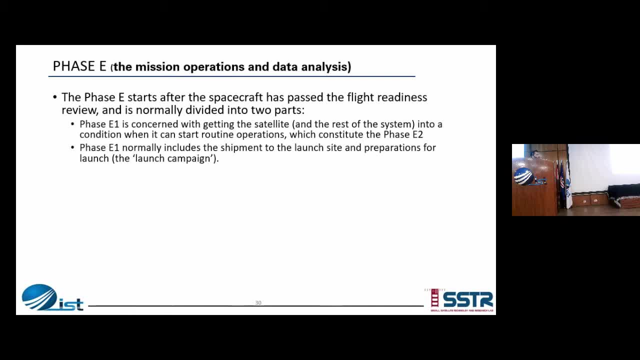 So when the integration and verification of satellite has been done or some other project. So we moved to this phase and we analyze the data which we are receiving. So phasy is concerned. So phase E is concerned, without getting the satellite into a condition. When the satellite is going to the satellite And then we move on to phase B condition when it can start routine operations and the phase even normally includes shipment to the launch site and also the preparation for the launch. these are also included in this phase. this is followed by launch and early orbit phase, which is the critical first few days. 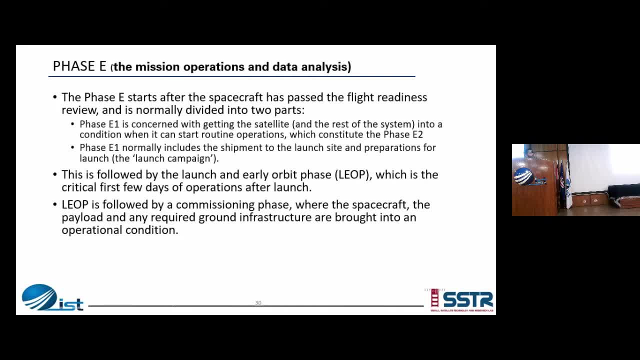 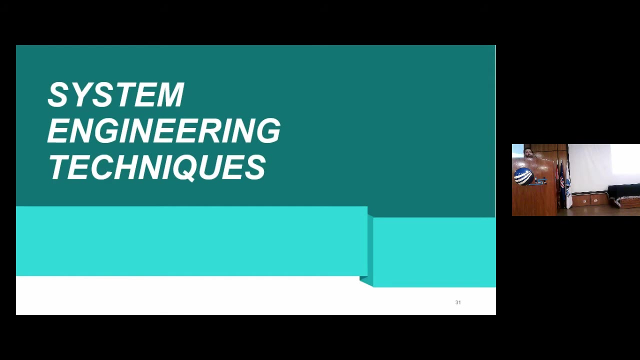 of operation after launch. then we have: this is followed by a commissioning phase where the spacecraft, payload and any required infrastructure are brought into operational condition, and at the end of commissioning we have the routine operations which rely on the ground sport. so after system phases we have a look into the system engineering techniques. what kind of 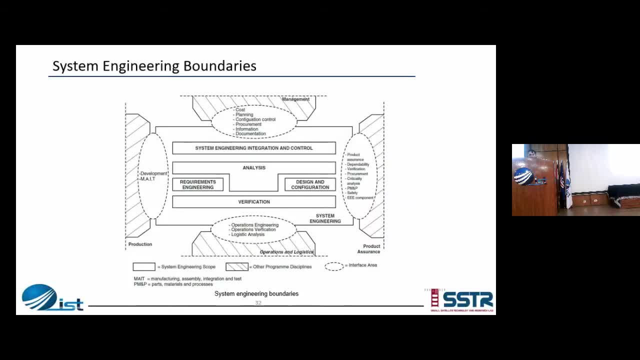 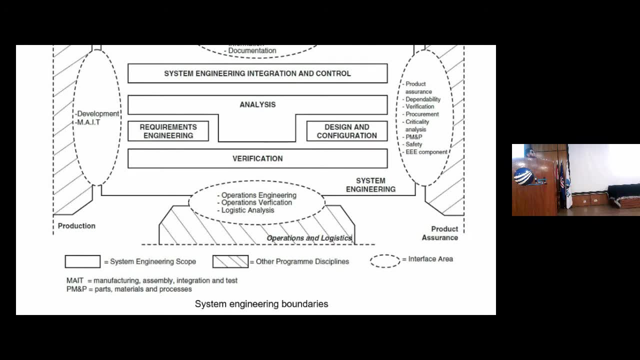 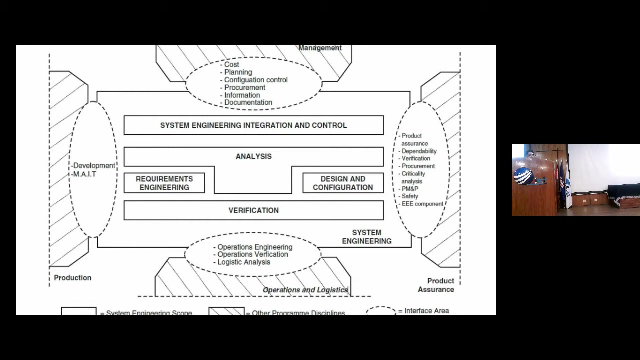 techniques we have in the system engineering. so if we look into this block diagram, the blocks which are solid like this they define the system engineering scope, and the blocks which have stripes in them they define other program disciplines. and the elliptical dotted kind of area, this shows the interface area. so it consists of development. so this comes in the interface area. 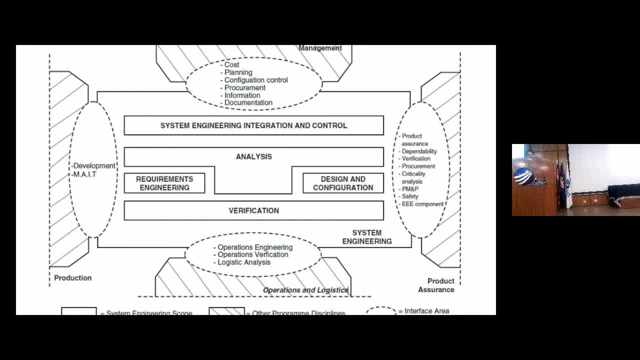 and these solid blocks. these are in the scope of the system engineering. this consists of requirement engineering, design and configuration verification. similarly, logistic analysis, operational engineering. so what comes out of the scope of system engineering? this production and product assurance? this does not comes in the scope of systems engineering. 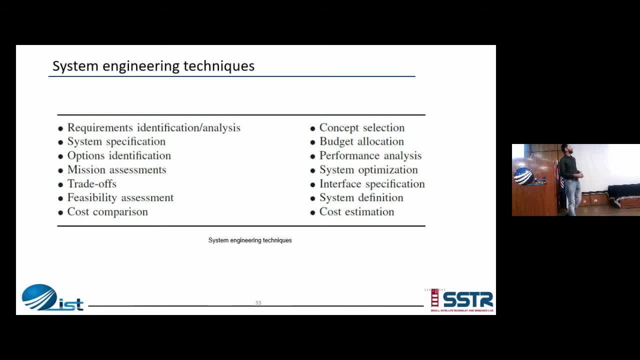 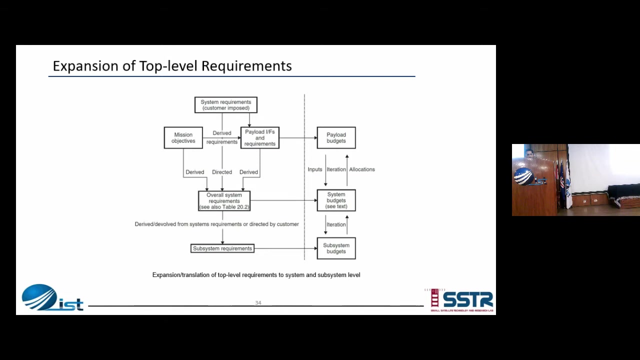 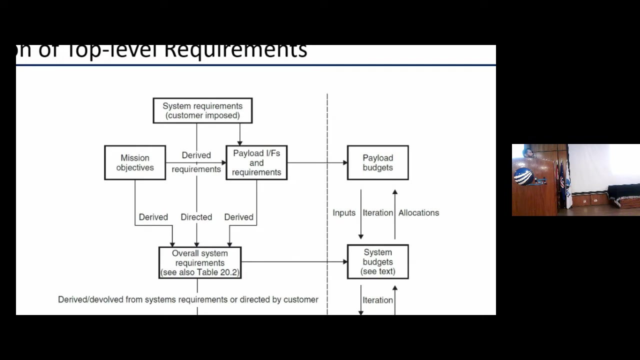 so these are the system engineering techniques that are used whenever we are developing some project. so it consists of requirements, system specification, mission assessments, trade-offs, cost comparison, budget allocation, interface specification and cost estimation. so this is expansion of the top level requirements. so on the top we have the system requirements or the customer needs. 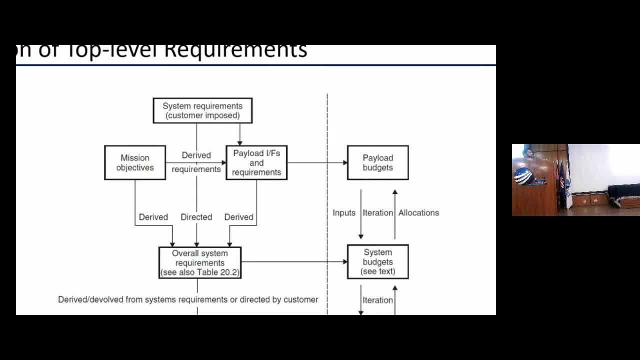 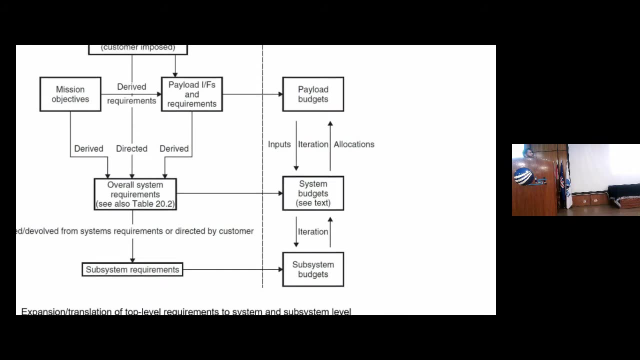 then we have payloads and requirements and on the other side we have mission objectives. so all of these are combined in the overall system requirements and on the side we have the system budgets, subsystem budgets and all of these things which are combined in the system requirements. they also lead to the subsystem level budgets, so we determine the. 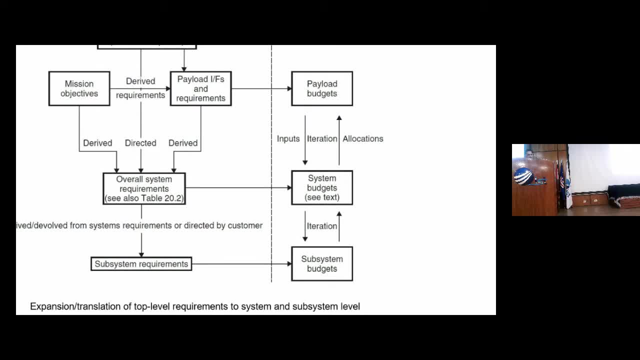 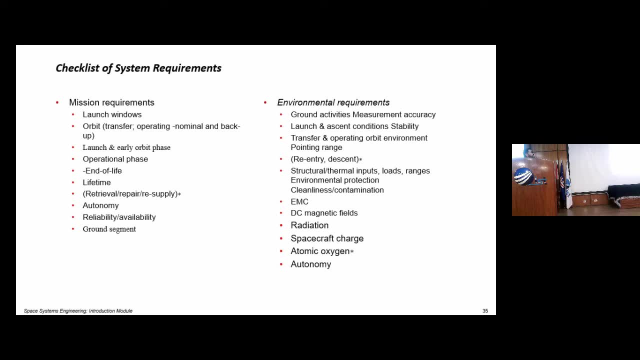 requirements at subsystem levels also. so this is the checklist which we have to make sure exist in the system requirements. so this checklist consists of different kind of modules. the first one is mission requirements. then we have to check the environmental requirements. mission requirement consists of operational phase. end of. 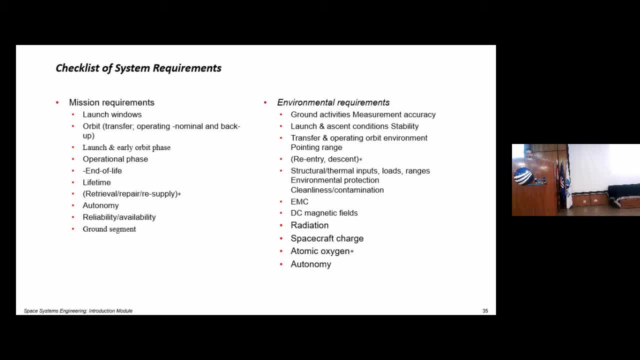 life, lifetime reliability, ground segment. and in the environmental requirements we make sure about the ground activities measurement accuracy. similarly, structural or thermal inputs, radiation at atomic oxygen level. this is applicable in some of the project. and then we analyze about the autonomy. actually there are six things in the system requirements. 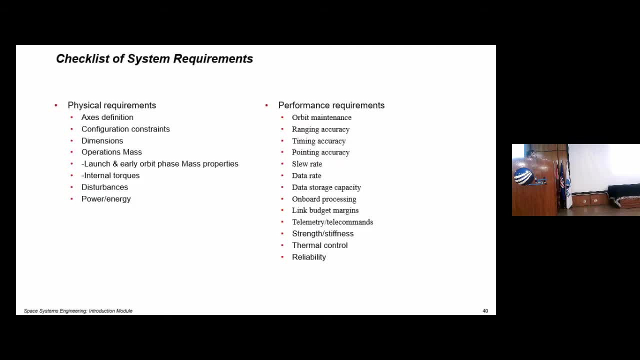 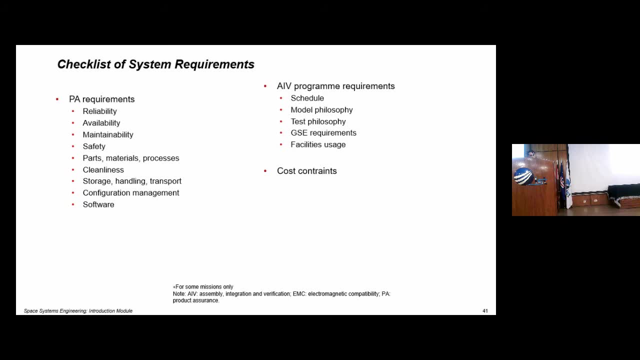 for simply saying that the Обjaw on energy source is coming. so we are complying with taiwan crude oil positive mass Dios system in the mountain or common. that see how others are referring to our government in Theater. so these are our tasks. for us, then, the task is going to be toDevelopment the system requirements. 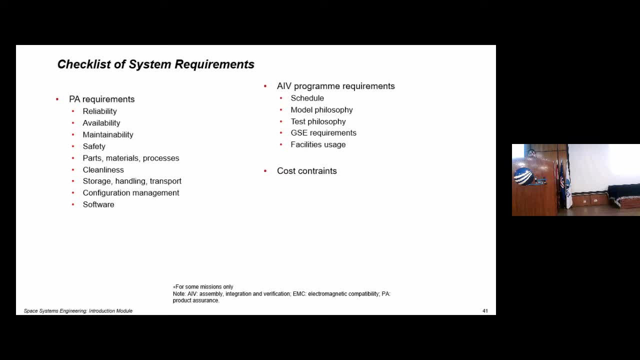 understand, on just making sure that we 24 k粒uu control level is too low. so these are all the things we want to do. there's a certain number of tasks we want to make sure of. these are job requirements, a edible requirement. so i think we have working applicationsblem Gee. there's a total of 20 a couple requirements and we have a very simple implementation on incident engineering requirements and environment requirements disagree. we are just some fairly general things to come in terms of we're going to discuss next in the models or we speak about future um, some other projects which are emergency with step by visit. there would be some other questions on the system requirements. 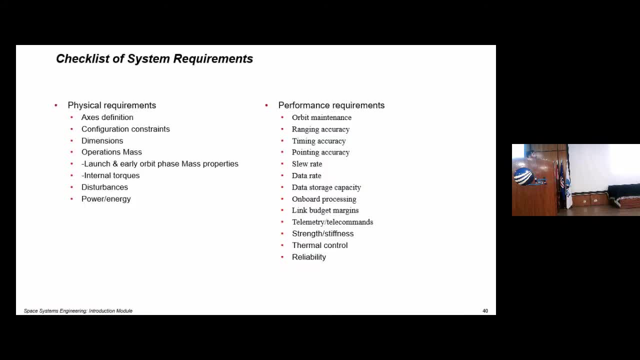 So if we look into the physical requirements, we have XS definition, dimensions, operational mass disturbances, power, energy. So these are in the physical requirements. And if we look in the performance requirements, we need to consider the orbit maintenance ranging accuracy, timing accuracy. 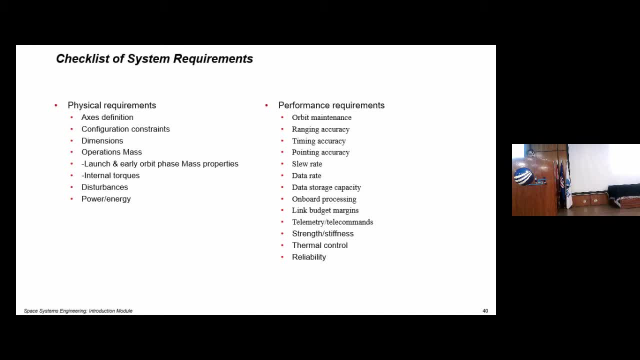 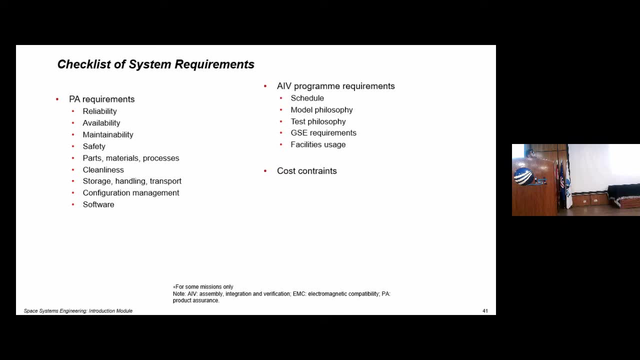 Similarly data rate, storage capacity, strength and reliability. Okay, in the product assurance requirement we have to check about reliability, availability, safety, cleanliness, storage, handling and transport and the configuration management, And if we see about the assembly integration. 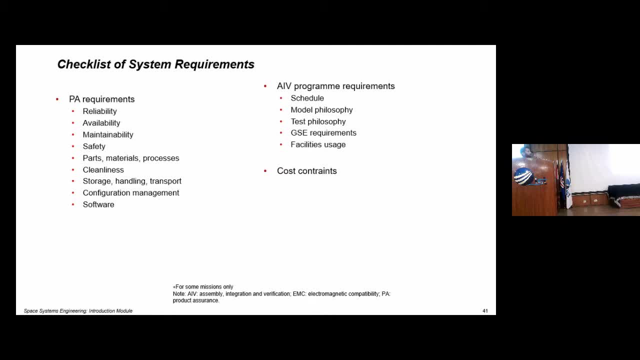 and verification requirements. we have to make sure about schedule, model, philosophy and the facilities usage And of course there is a cost constraint to each and everything. So these are system requirements. So overall there are eight requirements and every one of them have some subheadings or submodules. 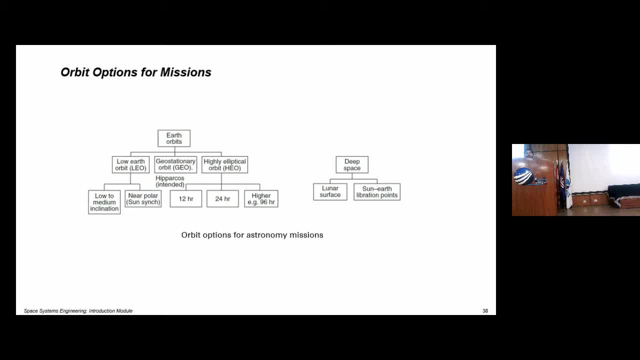 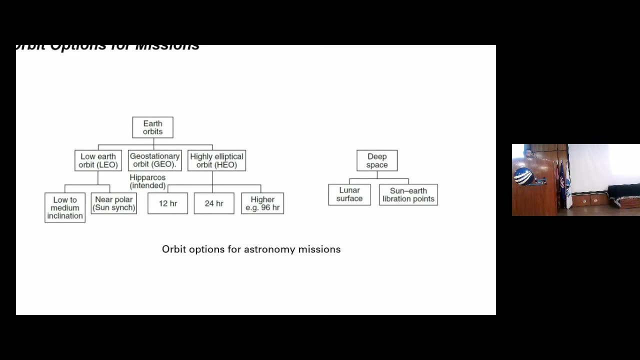 So this is the block diagram for orbit options for missions. So we can decide our orbit according to our project. So we can either have a low earth orbit or we can design for geostationary orbit, highly elliptical orbit or deep space missions. 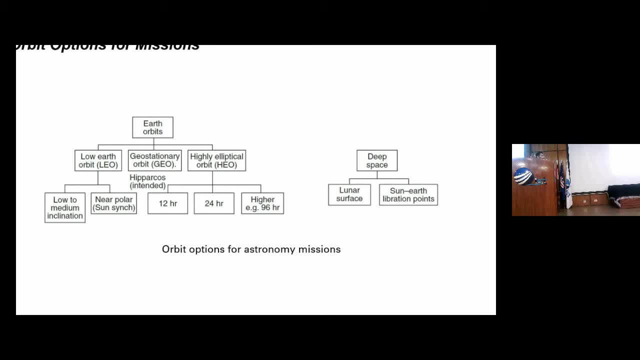 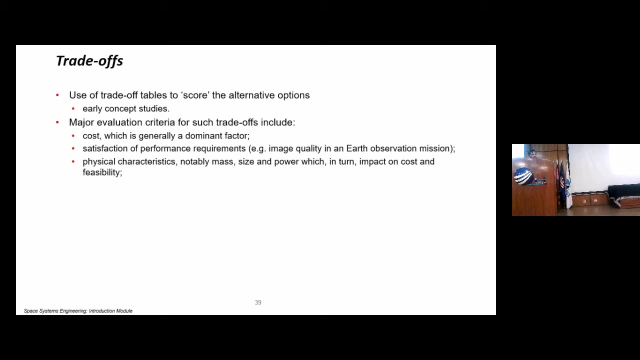 like lunar missions. So in case of CubeSats we usually make it in the LEO low earth orbit, which are at around 500 to 600 kilometers. So of course there are some trade offs and everything. So we use major evaluation criteria first for such trade-offs. so the cost is number one. we have to. 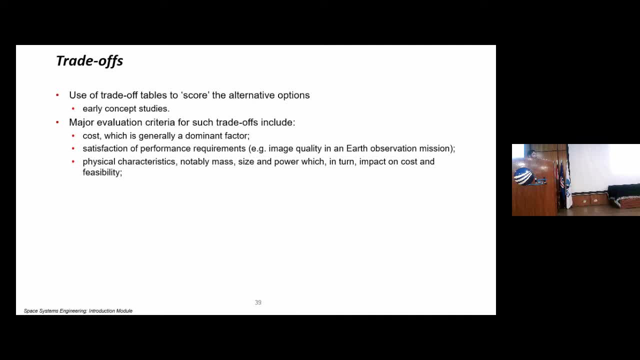 which is a dominant factor. we have to consider the cost in every case. similarly, the satisfaction, satisfaction of performance requirement. so the product which we are developing it is, we need to specify, we need to satisfy the end user about that product. similarly, there are physical characteristics which are mass, size and power. we need to have some trade-offs in that. 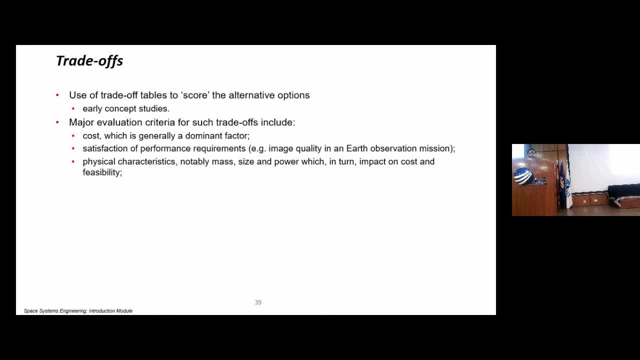 that and there would be some limitations in case of power size. so these are all considered in the design phase and we have to keep a trade-off between them. so availability of suitable hardware technology. so most of the time we design or maybe give an idea of some product, but we also have to 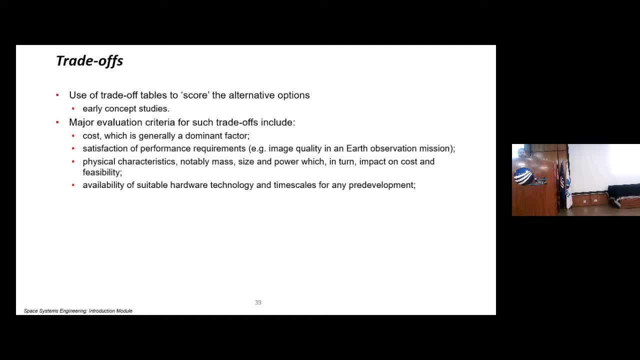 check that whether the suitable hardware technology is suitable for the product. so we need to check that whether the suitable hardware is available for that or not and we have to check the compatibility with launcher also, the launcher requirements and interface requirements. we have to consider them. then there is the flexibility to encompass alternative mission options. 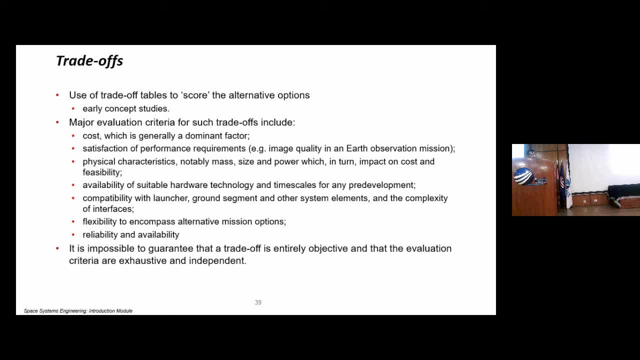 and reliability and availability. so it is almost impossible to guarantee a trade-off. that is mainly objective. so the this evaluation criteria is exhaustive and independent and we have to modify it according to our needs. so there is no standard like trade-offs, so we analyze it based on our requirements and our 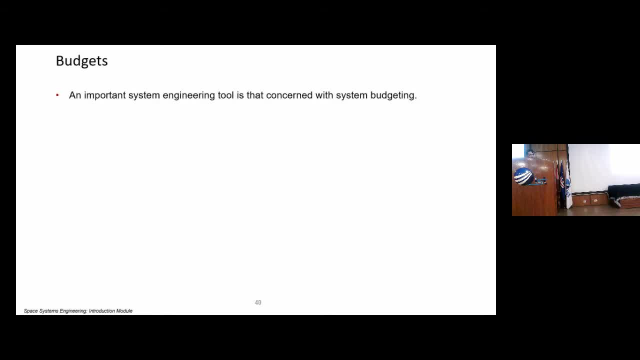 missions. next section is about budget, an important system engineering tool that is concerned with system budgeting. so at spacecraft level, the system budgets We usually make about the mass, You will only about the power, energy pointing and stabilization, Telemetry and telecommand budgets. 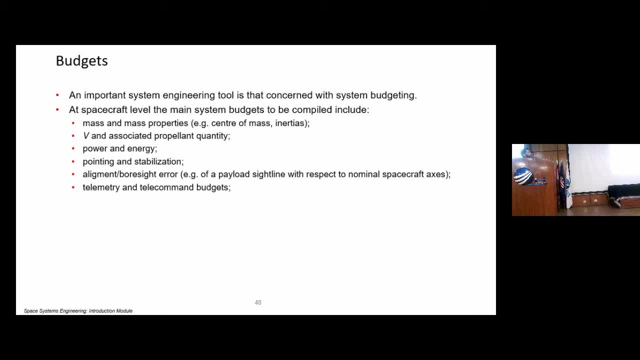 So there are different parameters in every of these budgets, so I will be demonstrating some of them. Similarly, there are data rates, storage capacity, communication, link budgets, reliability. So all of these budgets, they have some parameters in them and then the values are associated with them. 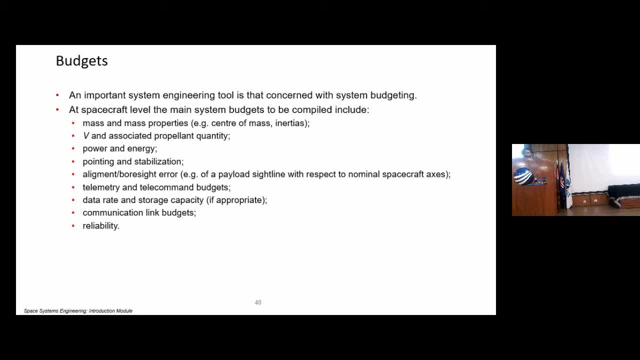 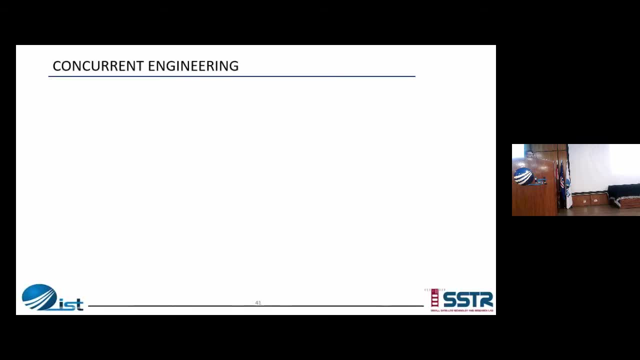 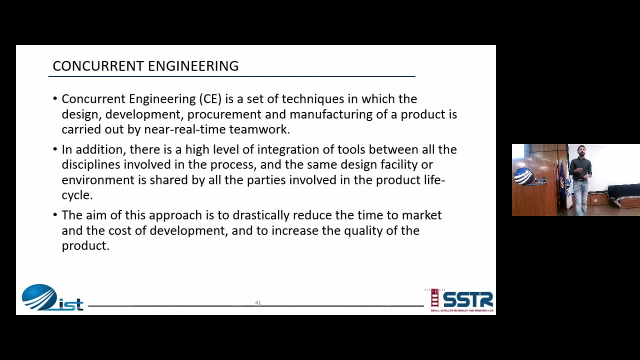 and we have to make a calculation about them. I will be demonstrating about the power, mass and link budget. So whenever we are developing some product, so we may have different kind of techniques. so it would be a sequential one or it would be that there is a center body. 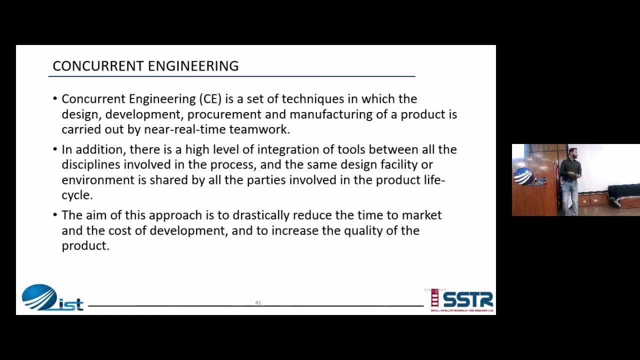 and all of the other subsystems are communicating with them. or maybe it is an advanced technique or concurrent engineering. So what happens is that all of the Things they are, all of the submodules and all of their team members They are, They have a communication between them. 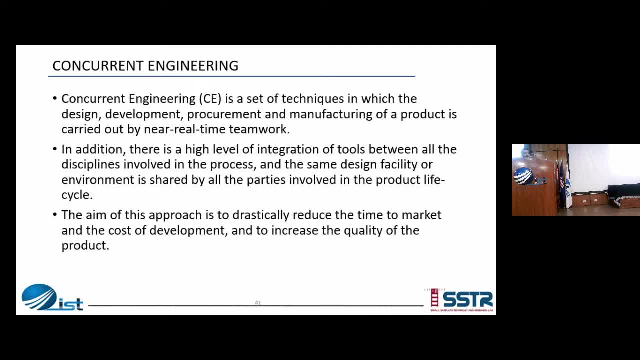 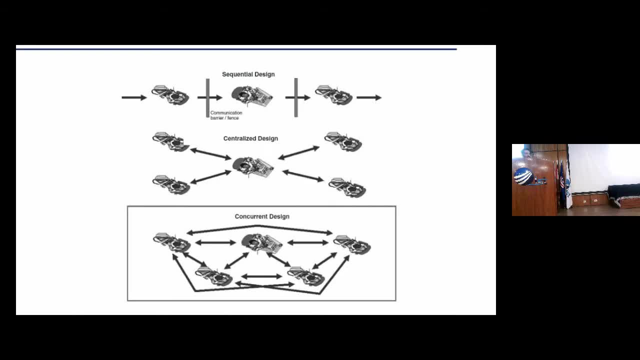 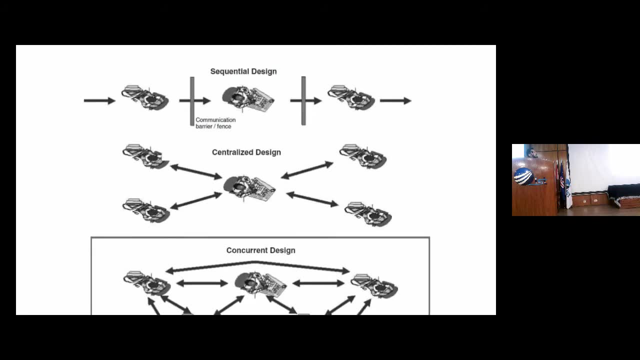 So the aim of this approach is to reduce the time and also to keep up the schedule for our project. So, if we look at this figure, So we have an option that either we do the things sequentially, like we make some component or sub some module. 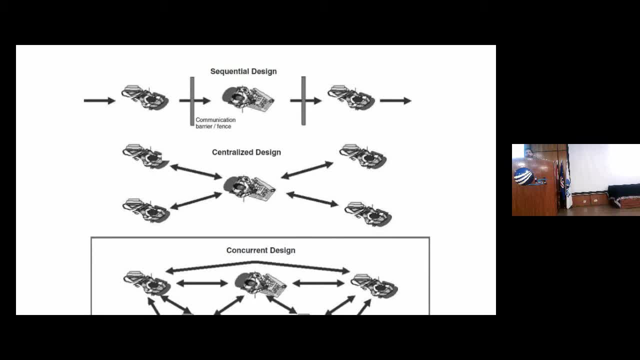 then we move on to next one, then to next one And if there is some modification, then again we I trade this cycle. or there is a possibility that we have a centralized design, that there is a central body or module and everyone is communicating with them. 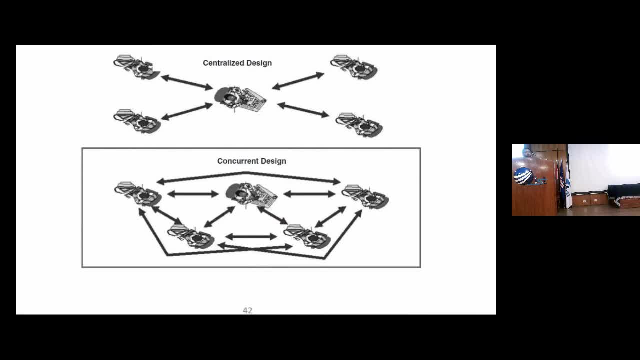 And in the last we have the concurrent design. so what happens is that all of the submodules are communicating with one another, So this is the more advanced and more efficient In terms of schedule, time and cost. so usually this concurrent design approach is used whenever we are. 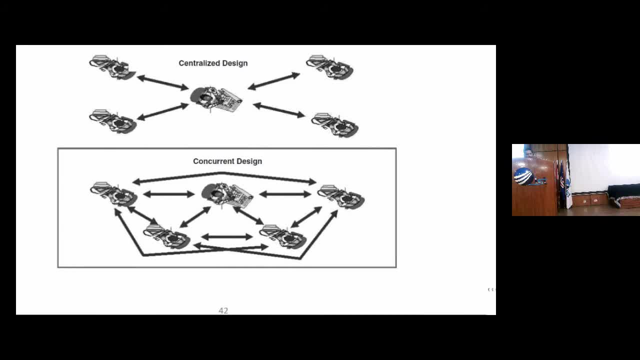 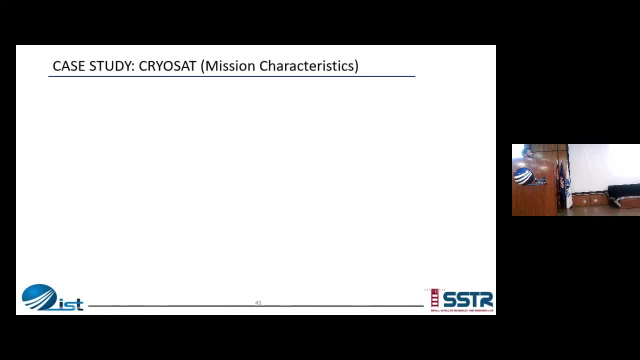 developing some spacecraft or some other projects. OK, so there is a case study about the cryosat. Cryosat is basically a satellite, so it was one of the largest or biggest satellite. So the purpose to demonstrate this case study is that why the organizations are. 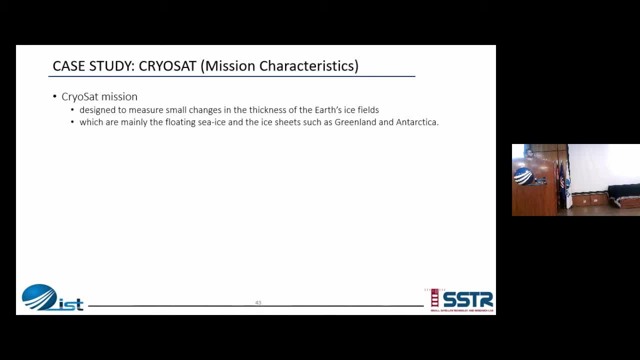 shifting towards the smaller satellites, because what a bigger satellite can do? So what happens is now that there is a constellation of satellite which could also achieve the same task that a bigger satellite is doing. So let's have a review about this case study. 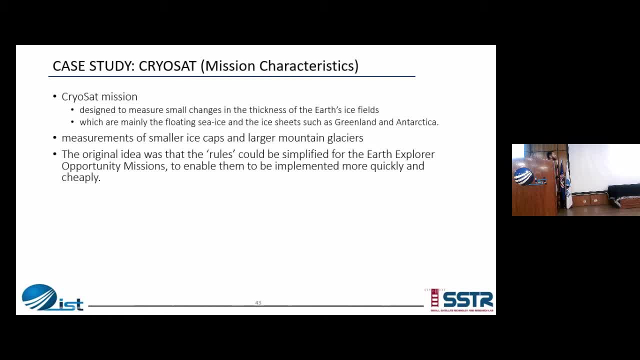 So the cryosat mission. it was designed to measure small changes in the thickness of Earth's ice field, So basically it was measuring the thickness of ice. This satellite, the purpose of the satellite, and the measurement of smaller ice gap and larger mountain glaciers. 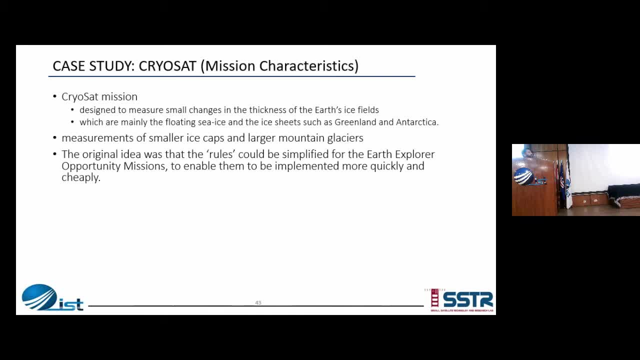 Similarly, the original idea was that rules could be simplified for Earth Explorer Opportunity Missions to enable them to be implemented more quickly and cheaply. This was thought to mean less rigorous quality, less reliable hardware and perhaps less redundant systems, But in reality it was difficult to implement two set of standards. 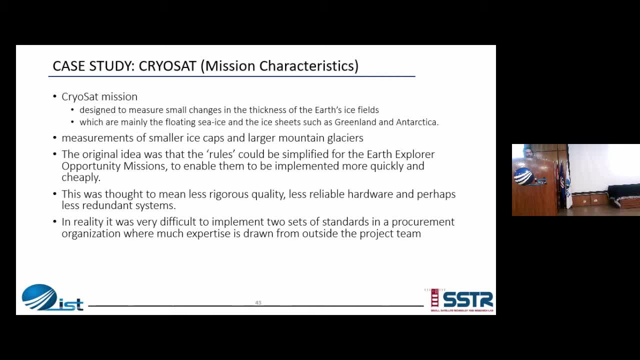 in a procurement organization where much expertise is drawn from outside the project team. So what this is telling? so this was a European Space Agency project, So initially they thought or implemented to make it at a cheap cost. but they had different organizations and they have a. 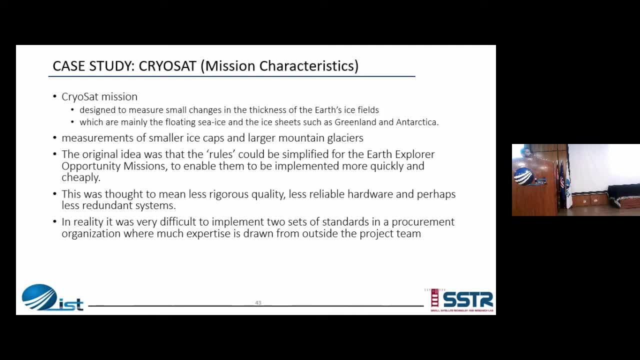 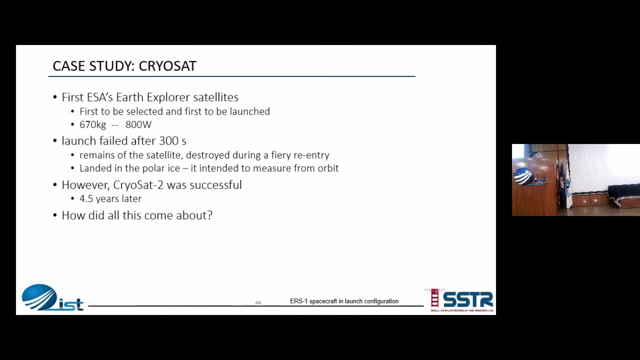 kind of collaboration. So what happened is that they turned up Increasing its cost and its time and schedule. So Let's have a further look. So this was The first Earth Explorer Satellite of European Space Agency and it was about 670 to 670 kg and the power for this satellite was 800 watts. 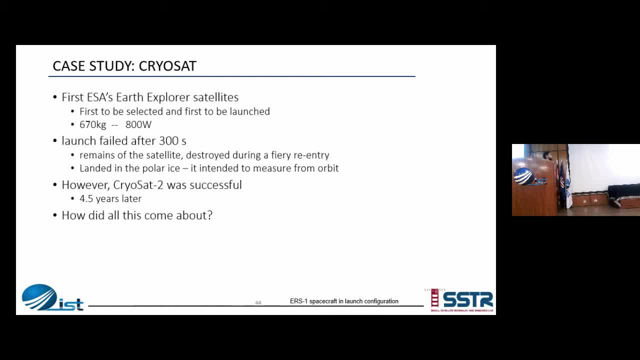 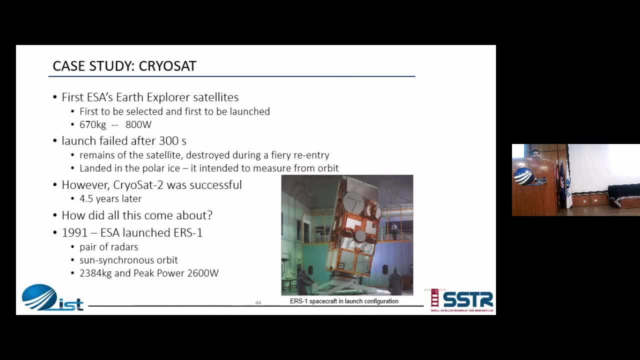 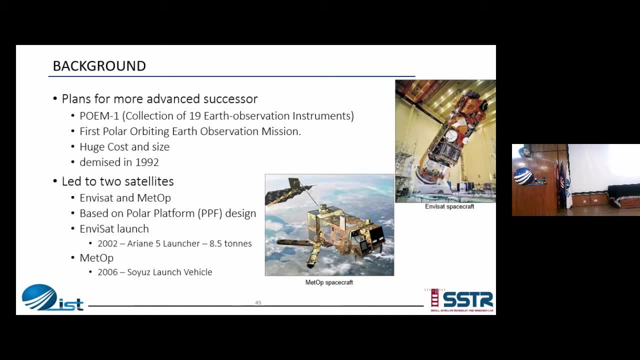 And so the kilogram and it consumed the power of 2600 Watt. So after that the plans for more advanced Missions were selected. so it consists of This point one satellite which was collection of 19 Earth observation instruments. So this was a one big satellite which 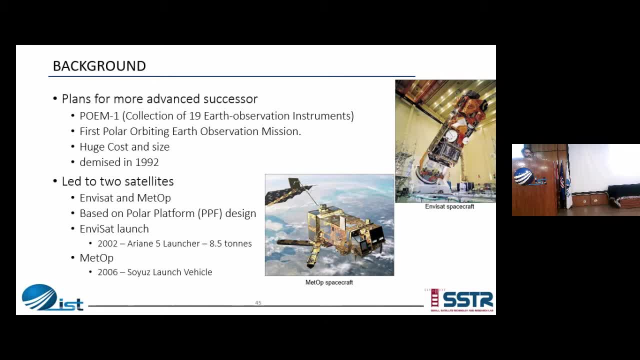 had around 19 instruments on board this satellite And it has huge cost and size and this was backed. This was demised in 1992 because of its huge size and cost. So what happened? that this led to the creation of two new satellites. 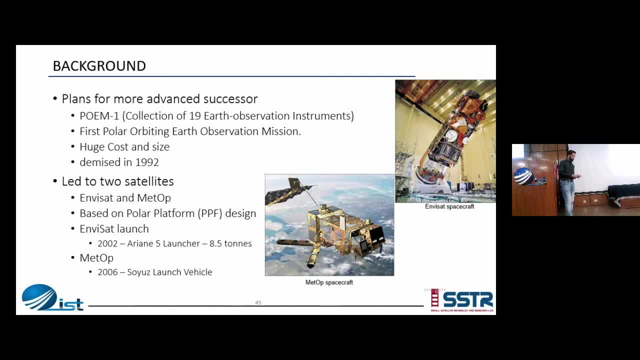 which were in reset and metal, which are also shown in these figures. So this one was made of spacecraft and this is, And we said, spacecraft. So these were also based on the polar platform design, meaning that they were designed to measure the ice or glaciers in the 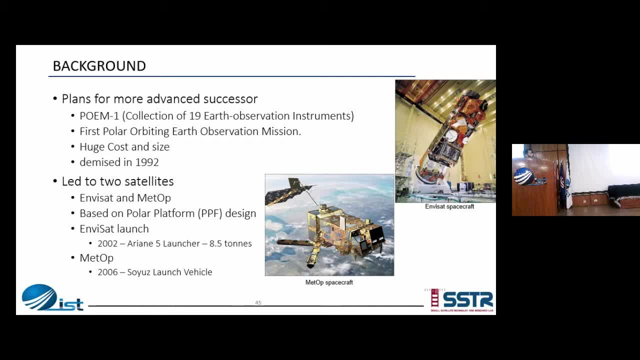 Polar regions, And this in. we said it was launched in 2002 and it was weighing around 8.5 tons, which is 8500 kilograms, So it was a big satellite. Similarly, This was also met up. It was launched in 2006.. 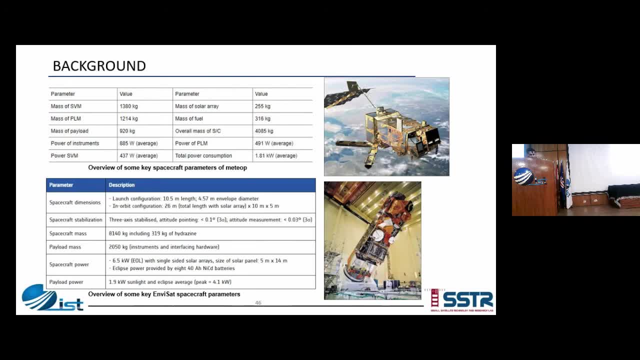 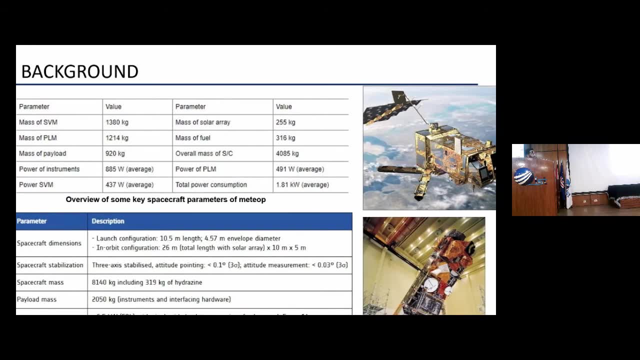 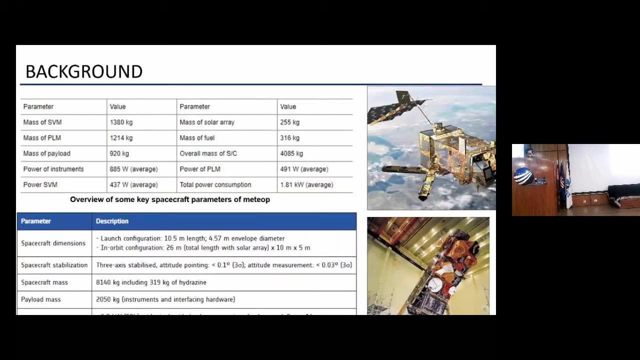 And If you look at the tables Of these satellites, so there are some parameters and values associated with them. So the first one is about my top satellite and This is showing the mass of payload, mass of instruments, So as we can see that it has huge power and mass requirements. 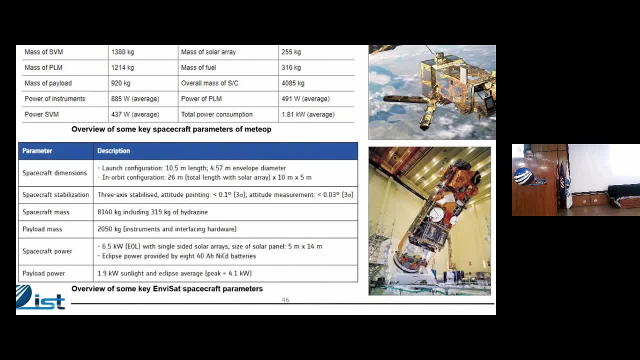 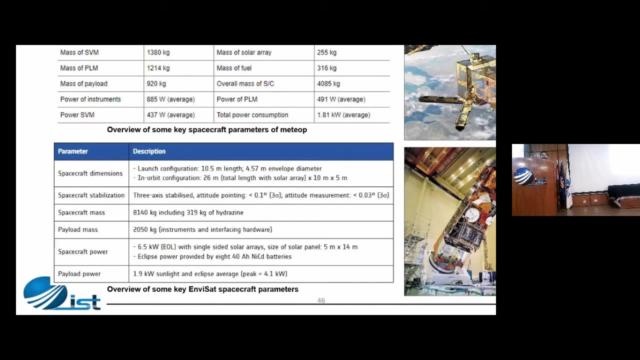 Similarly, if we look at the other one in we said that also had around the payload mass of 2000 kilogram. Similarly, the spacecraft itself was Around 8,000 kilogram. So what the purpose of basically telling all this is that how we lead to these small satellites which we 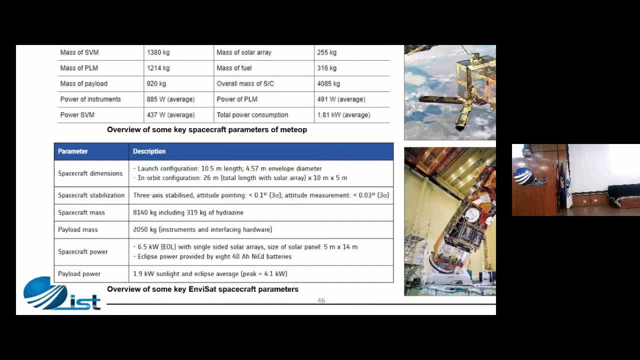 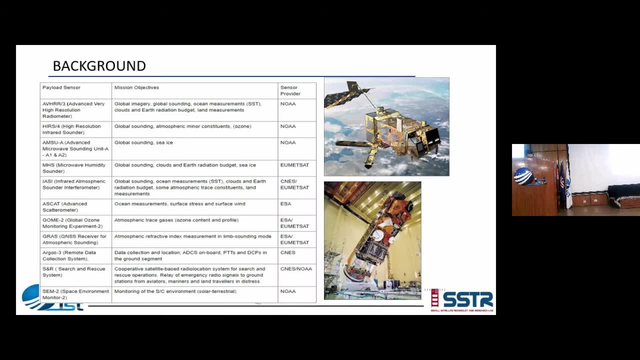 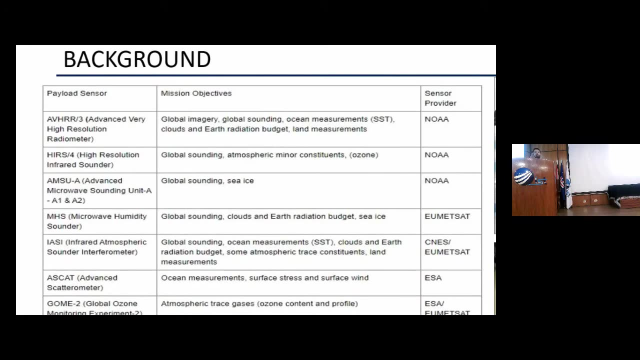 see nowadays huge satellites. So this is the story or history behind all of this. These were the biggest satellites And, as I told you that they had on board like 13 to 19 instruments which would make a different thing. So here is a list. 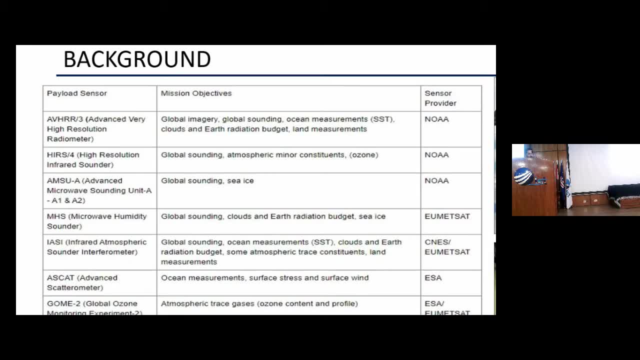 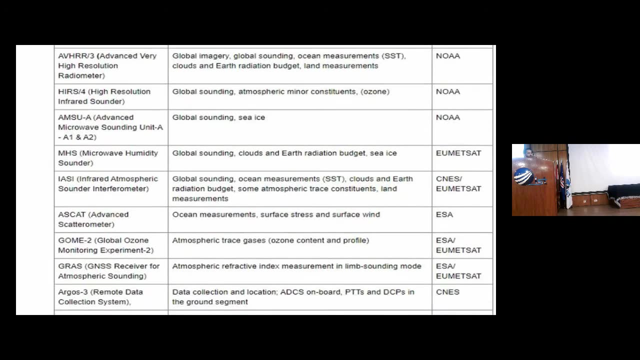 of some of the things. So if we look at them, that it had advanced very high resolution radiometer, What would it do it It wasn't used for the global imagery, global sounding ocean measurement? Similarly, if we see this one infrared atmospheric, 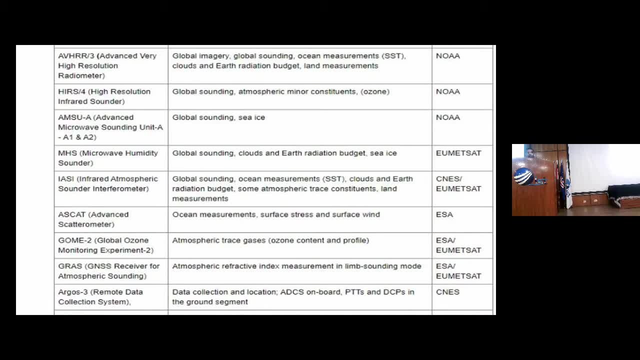 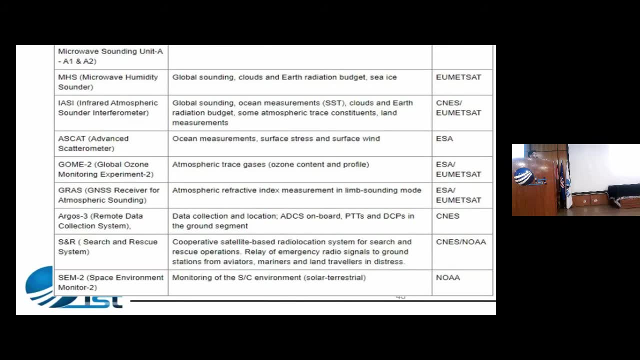 Some other inferometer, So this was used in the ocean measurement readings. Similarly cloud and Earth radiation budgets, and there is a lot of information about the solar system. So if you look at the top list, you can have a look at them later. 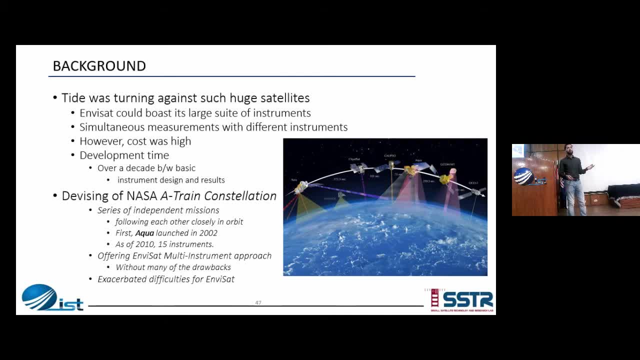 So these all of this was happening back in 19. like this all started in 1991-1992. So at the time of their launch, that was around 2000 or 2002.. What happened? that there was another mission of NASA that was. 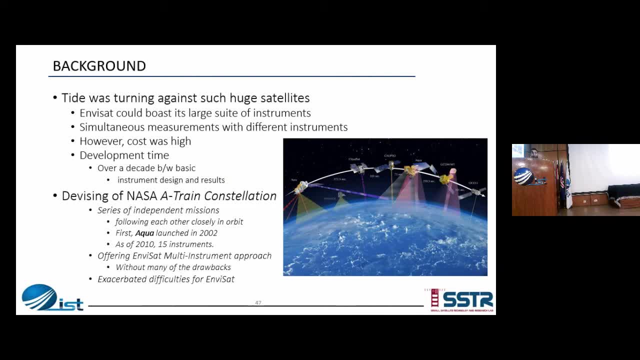 The afternoon train constellation. So what happened is that The Instruments are the measurements that the biggest satellite of European Space Agency, which had on board like 19 instruments, So the NASA- made a constellation of satellites and they all have different Instruments on board and they were also performing the similar. 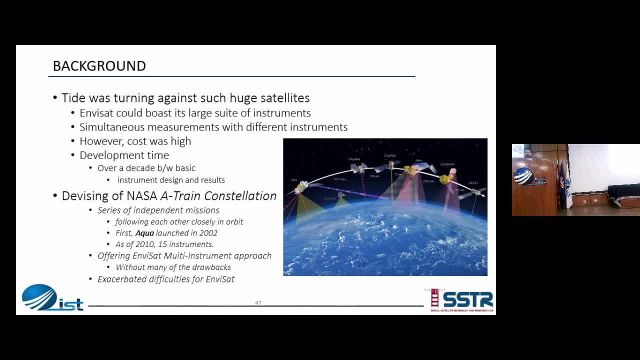 tasks. So this was the first time when this concept of constellation or the small or different, Or we can say that, dividing a bigger mission or project into smaller components, So all both of these things were equivalent, but what happened was that one of them was bigger in size. It has 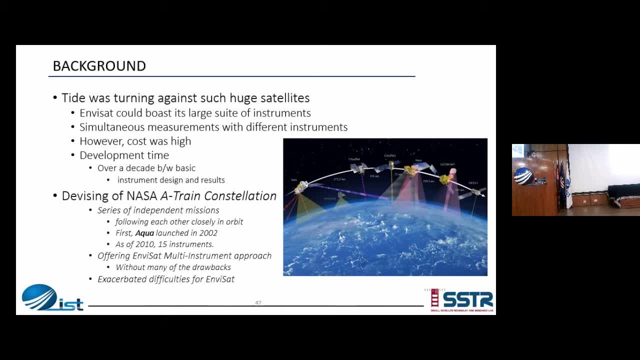 huge cost, mass and power, while the other one was smaller and it has less time schedule and development phases, But the purpose of both of them were same, So this was the first. one of it was launched in 2002 and as of 2010.. 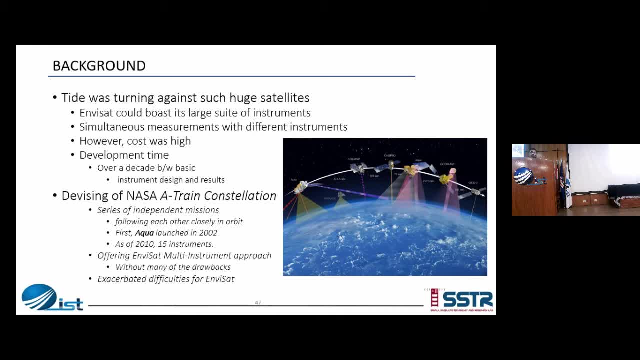 The 15 instruments, meaning 15 satellites. they have been in constellation And these cubes are the lights. They also came around data, like in 1999.. Their design specifications were identified and in 2002-2003 they started to emerge and launched. 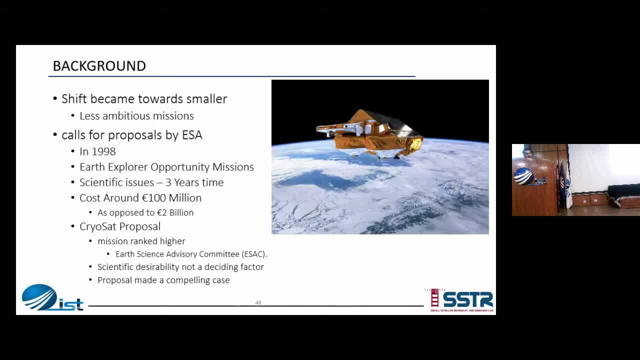 into the space. This is the history, This is the brief history about these smaller and bigger satellites. And then the shift became towards smaller. Why? Because it They were less, They have less ambitious missions and they were easy to manufacture, integrate and keep them on schedule. 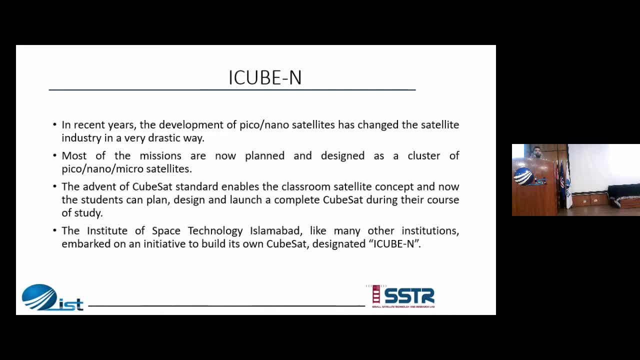 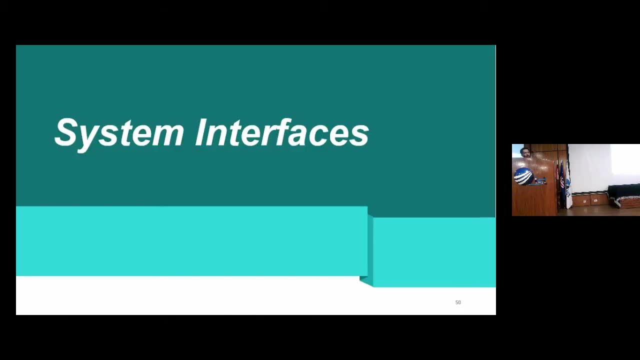 So this is a little detail of about IQ band. You already may be knowing that this is TRL lab is the first one of it, which was IQ band. It was launched back in 2013.. So so far, I have demonstrated the intro of our systems engineering. 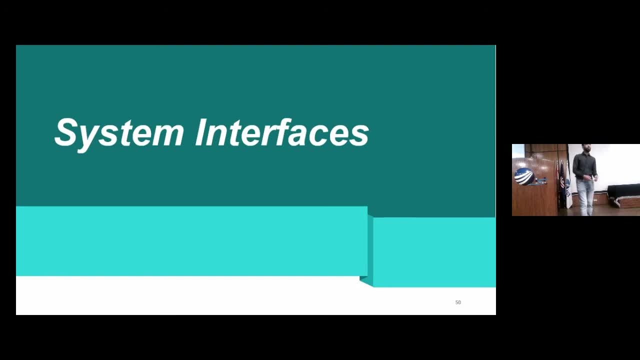 Then we discussed about different phases or techniques, about system engineering, and I told you a background about satellites, that how they were bigger in size and then eventually, Or why they shifted towards the smaller size because the same missions could be achieved by the smaller one. So now we will have a look into the system interfaces. 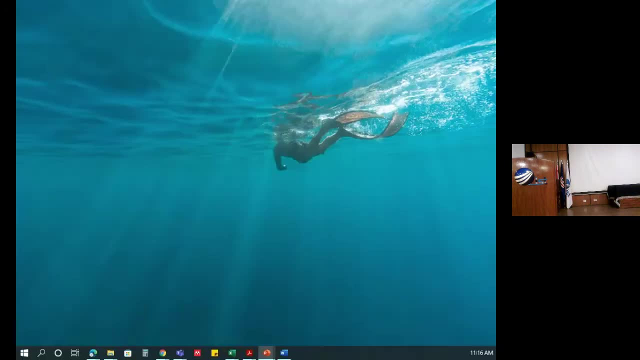 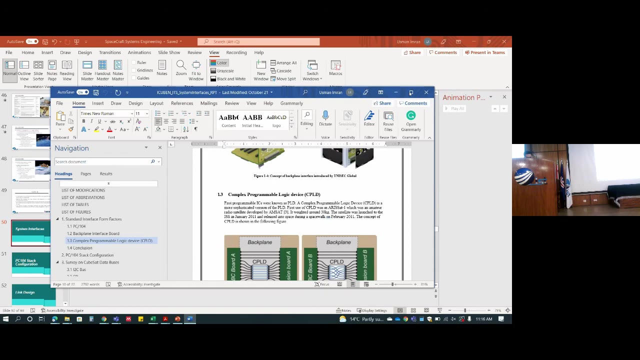 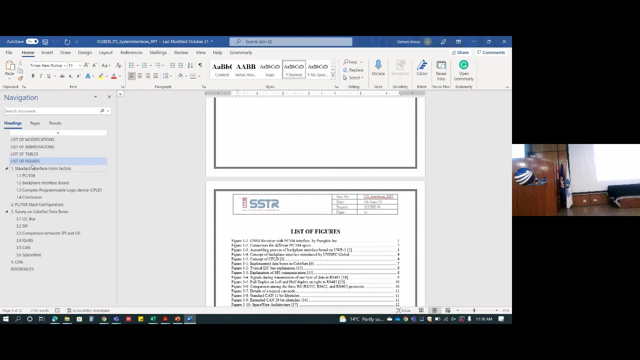 So For system interfaces, I will refer to this document or report, But- But This is a report that was released in 2019.. So it's a report that was published in 2019.. It's the first one I will show you. 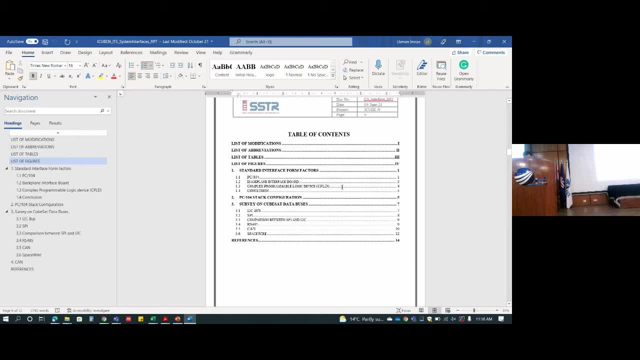 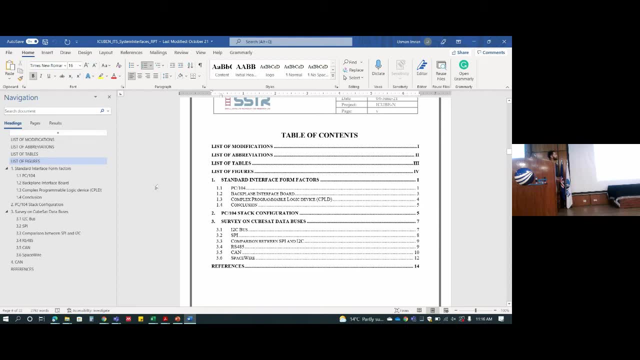 But I will try to show you the first one. OK, so we prepared this report while working on the IQ band, So the first one in this is the. OK, so we prepared this report while working on the IQ band, So the first one in this is the. 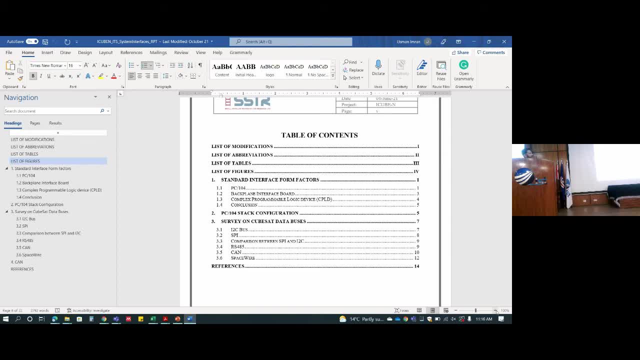 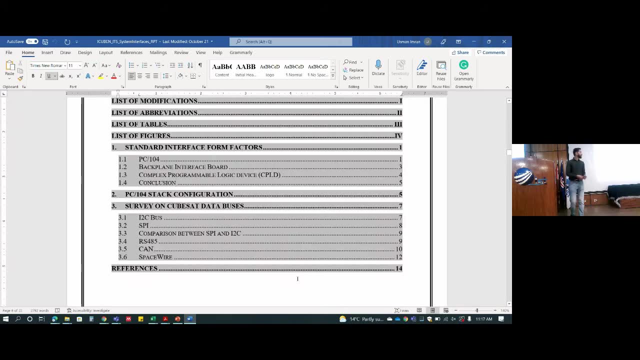 So the first one in this is the: can you see it now? okay, so we will discuss these few things in this document: standard interface, form factors, cc 104, stack configuration and the survey on cubesat databases. so as you all may have studied the spacecraft course, so can anyone of you tell me that how the subsystems of the 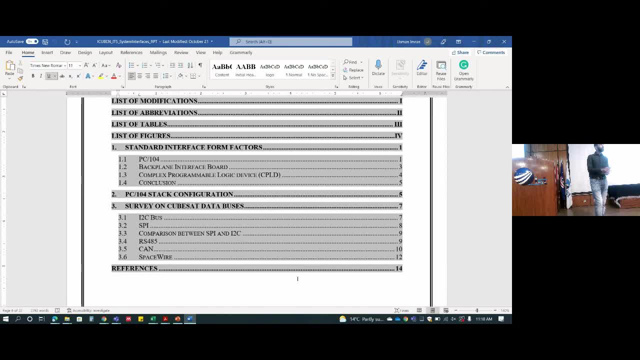 spacecraft. they are connected together like what kind of headers or connectors they use, anyone. okay, how many of you have heard about pc104? you know only you, maybe a bit so so you didn't studied about taking some spacecraft course or the connectors or headers. okay. so when we develop some satellite subsystems, we have to interconnect them. so 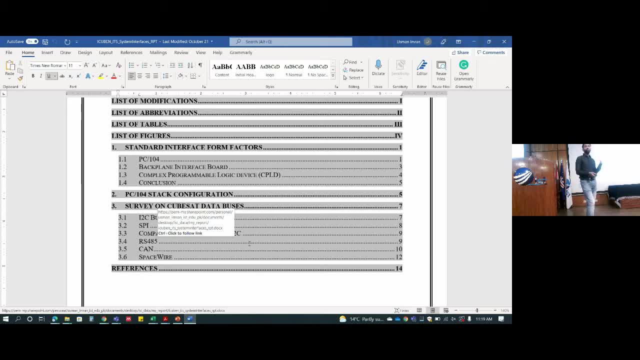 there are three possibilities that we can connect them. so the first one is the pc104, which is a kind of standard, and there is also a possibility that we use some back lay interface board, and the third one is complex programmable logic device. so i will explain all of these three one by one. 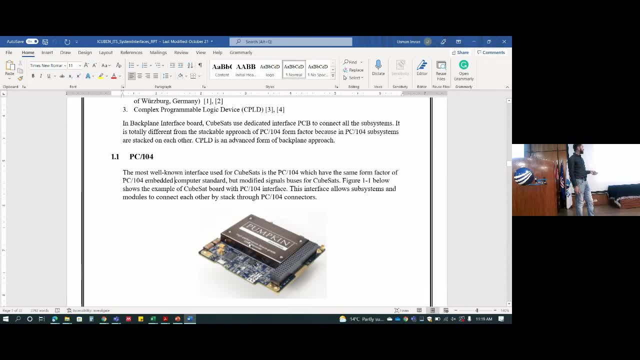 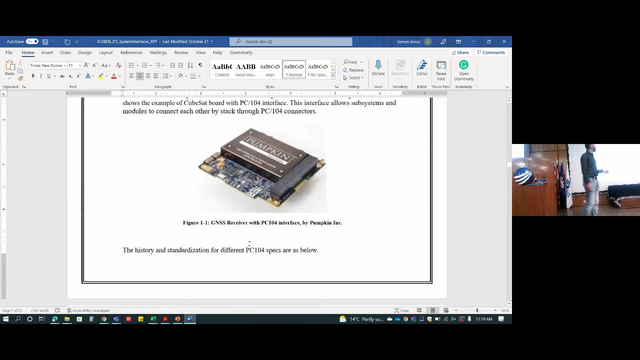 we go on to the first one. so this is an image of the nss receiver pc104, which is by pumpkin or things operation. so if you see that there is a list of connectors, so we call this form factor as pc104. so basically it has 104 connectors on its board, so most of the spacecraft subsystems. similarly, in case of 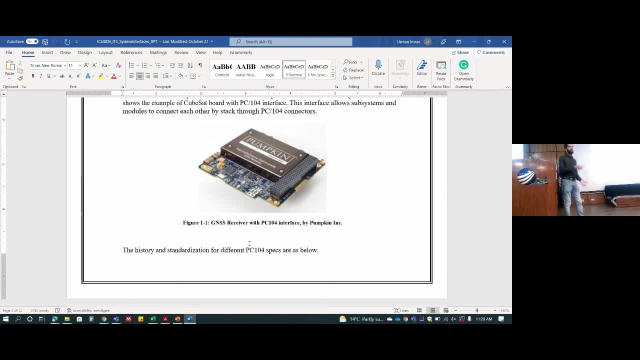 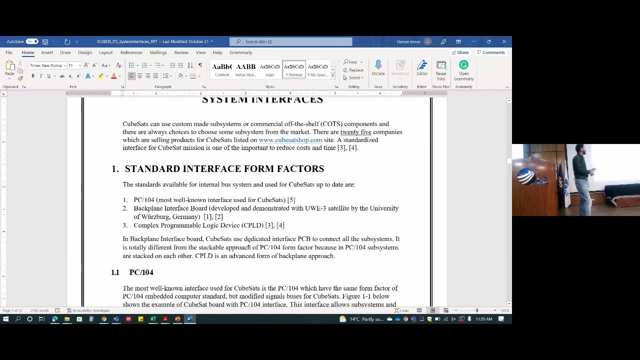 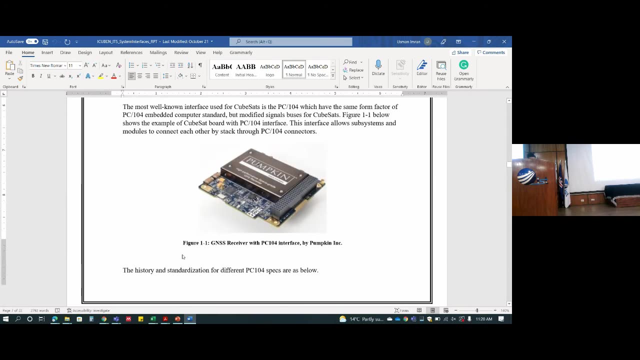 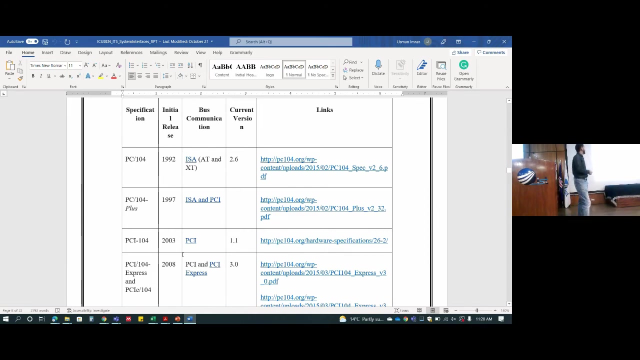 cubesets. they have this kind of form factor and they are stacked together which are interconnected. this is the first form of standard interface form factor and in case of pc104 there were different versions. the first one was released in 1992, then 1997, then 2003 and after that 2008. so they all have different kind of specifications and 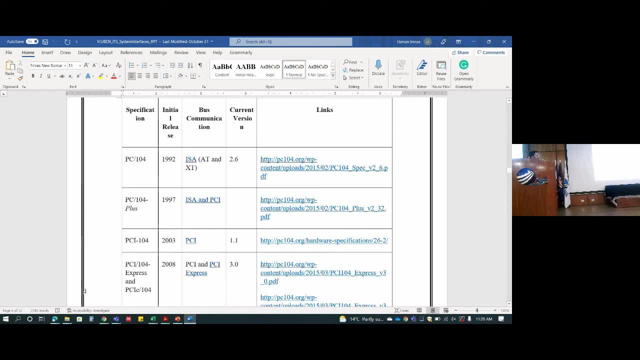 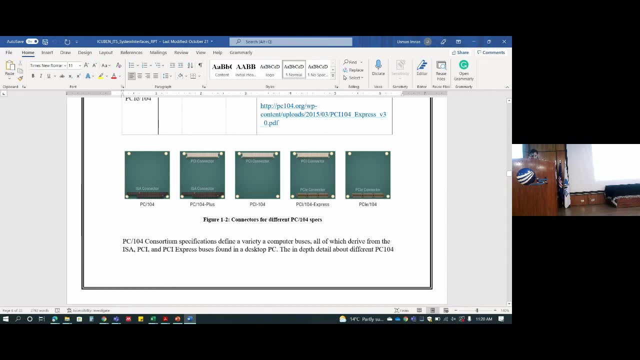 link for their further description is also provided. so, uh, nowadays and there is a PC104 express version, It has kind of three subdivided headers And then there is express one core. so they have different kind of headers and requirements and specification, but usually this PC104 we use. 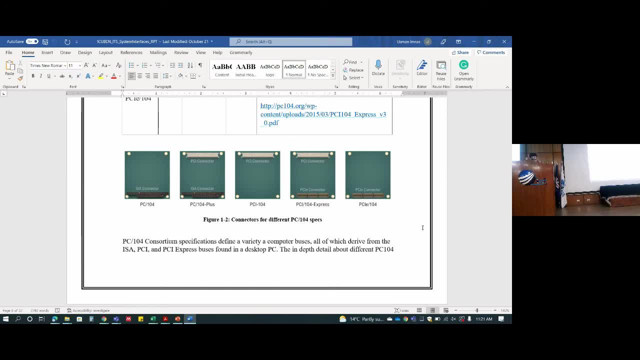 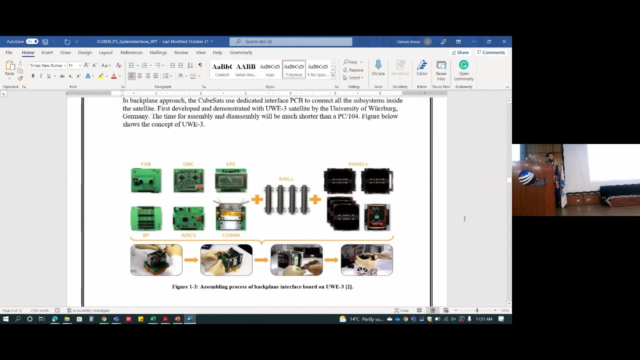 this, while the CubeSat development And also the commercially available units for the CubeSats, They also have this kind of PC104 connector. So this was the first option. The other option we can have is that we make a standard kind of board or a. 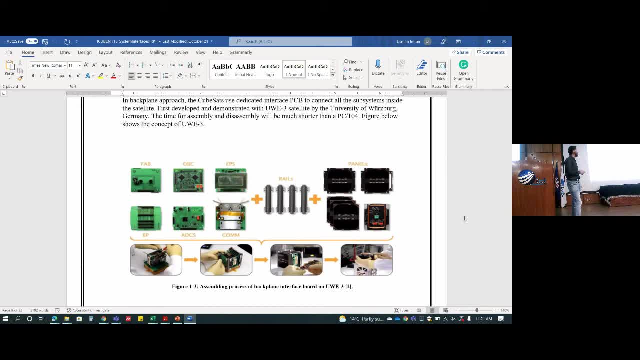 main board and what happens is that all of the sub boards they are, they got connected to that main board. If you look at this board, the pointer, so it has a lot of headers on it. So what you do is that you connect different boards- OBC, EPS- on their locations. 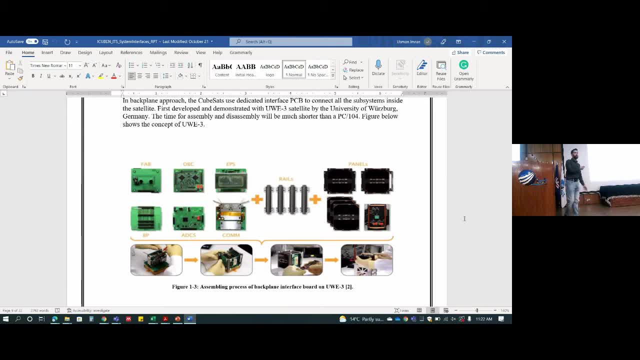 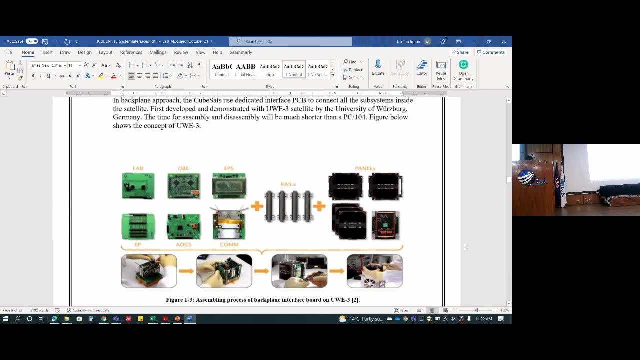 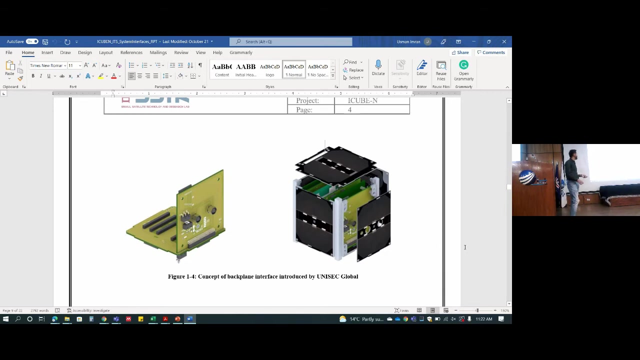 So this is also a technique or standard form of interface that can be used, but this is not much more rugged or reliable. so that's why PC104 is still used in the CubeSat lights. So this is also the second one which I was telling you. 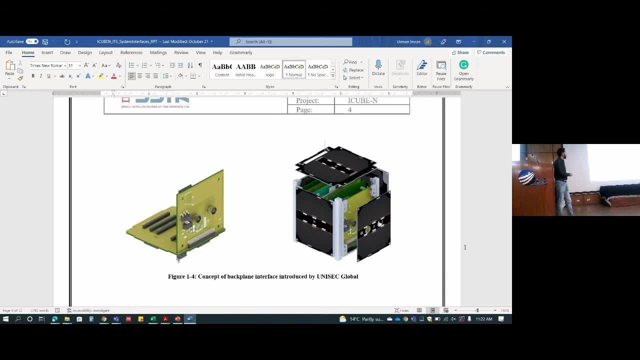 The concept of backplane interface board. so you can see there is some camera modules which is stacked on this board and there are options for other boards that can be stacked. This is not that much strong connection or reliable, so that's why we opt to use the PC104.. 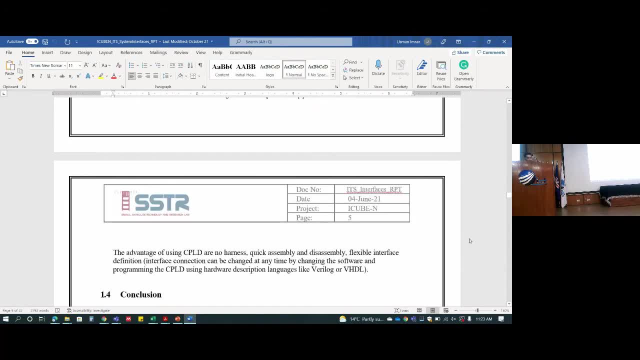 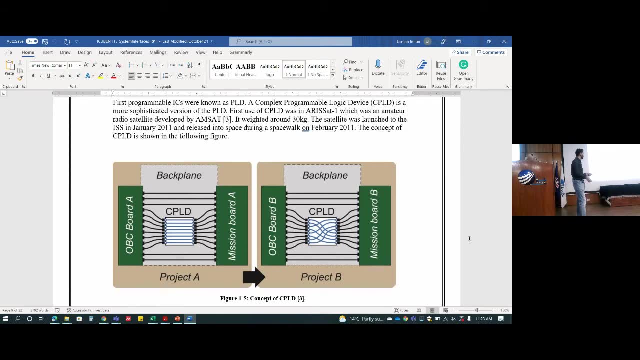 And then there is This third technique, which we call as backplane, or complex programmable logic device. So what we do is that, instead of developing different kind of stack connectors, we have a chip which is controlling the routing of all of these boards. 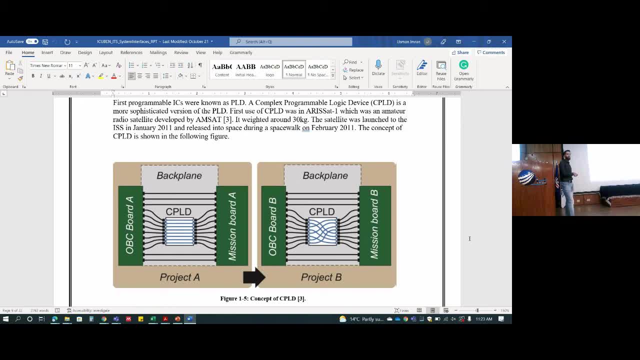 So let's say that this is mission board A and this is OBC board A. So instead of their physical connectors, like in case of PC104 or backplane interface board, we have this chip and we can program and reprogram it according to our requirement. 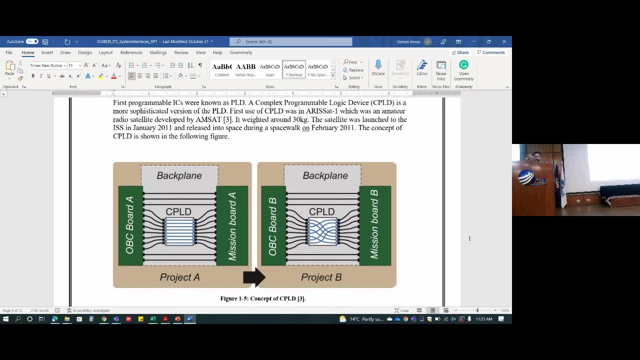 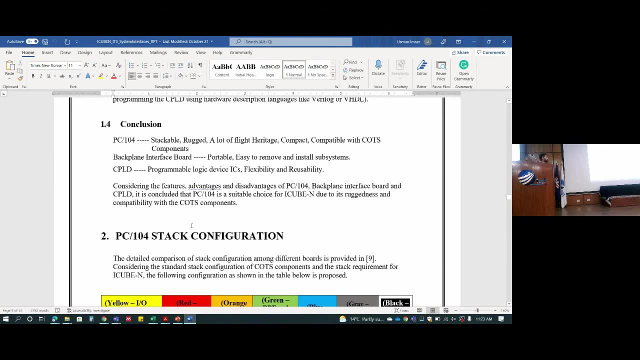 So we basically program this chip according to our requirement. So this is a conclusion about the standard interfaces. We look at the first one, PC104. why we use it? because it is stackable, It is rugged and it has a lot of flight heritage. 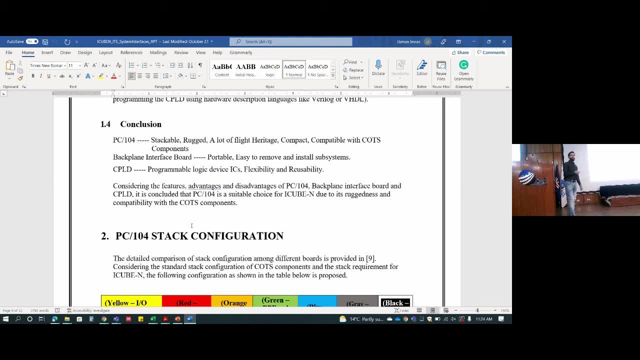 Similarly, it is compatible with commercial off the shelf components And the backplane interface board, although it is portable and easy to use and easy to install and remove also, but it is not that much rugged or reliable. And this programmable logic devices. 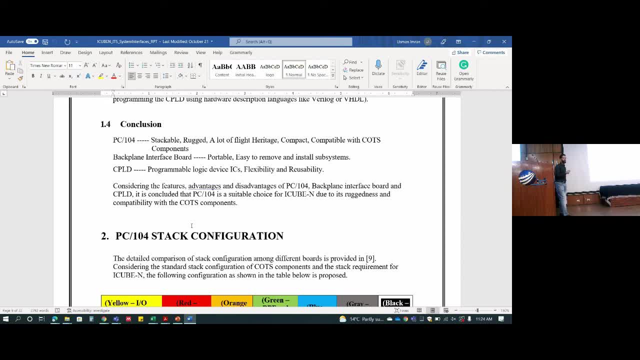 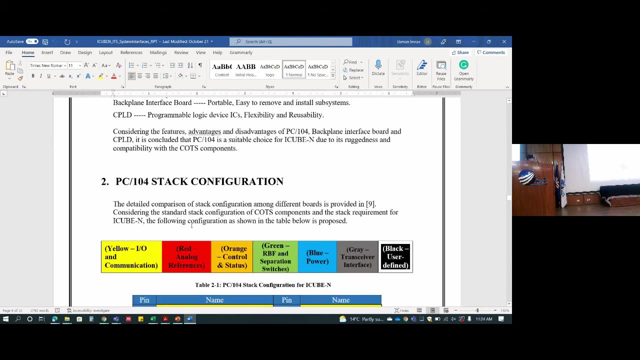 it is in the development phases. The technology has not matured that much yet but it has some usage, or flexibility and reusability are there And then maybe in future there are some advanced versions of this CPLD technique. So just a quick overview of this system. 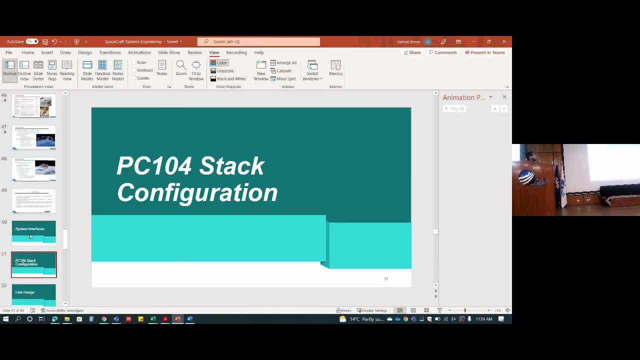 So the system interface. we will have a look on the PC104 stack configuration, So these three standard interface boards, PC104, backplane interface board and programmable logic device. So we selected PC104 out of those three And now we will have a look at how this PC104 stack is configured. 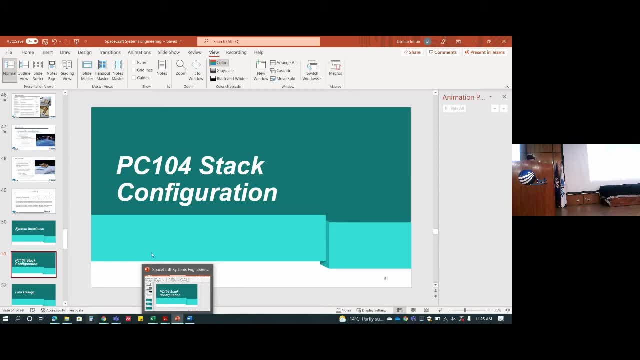 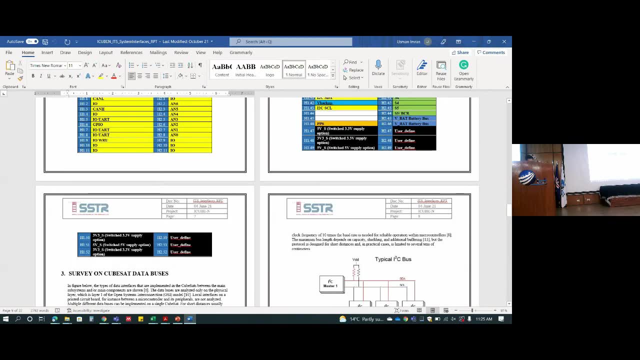 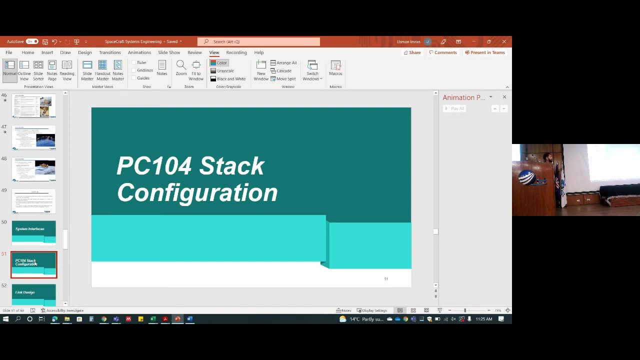 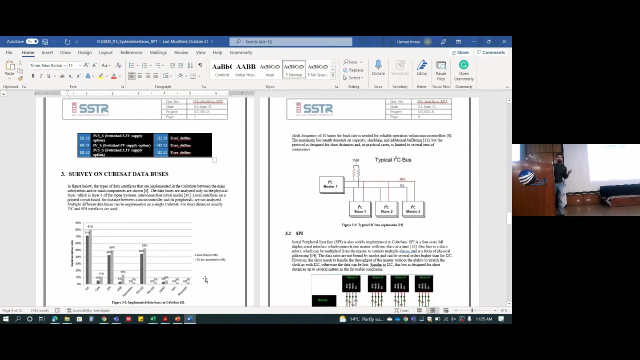 And it looks like we have this one here. So We will have a look at this later. but let's first discuss about, Let's first discuss about the CubeSat databases. Let's see how the SPIE, I2C or the CAN protocol. 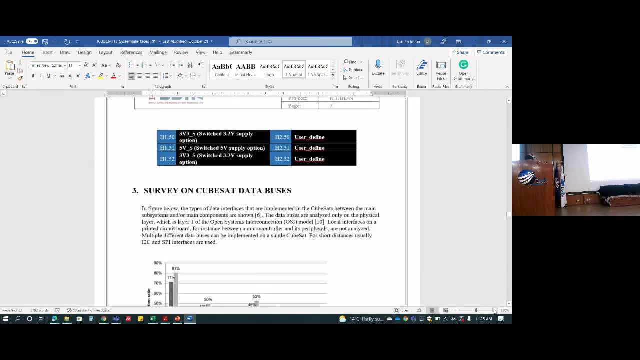 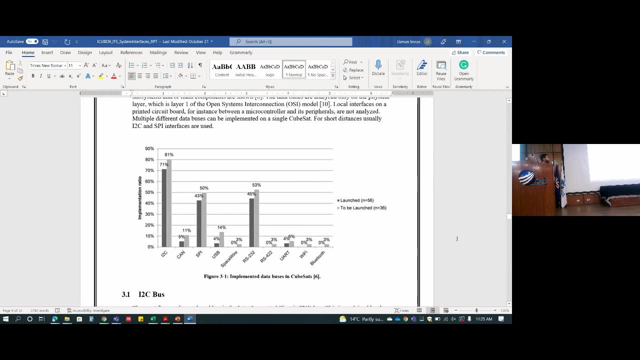 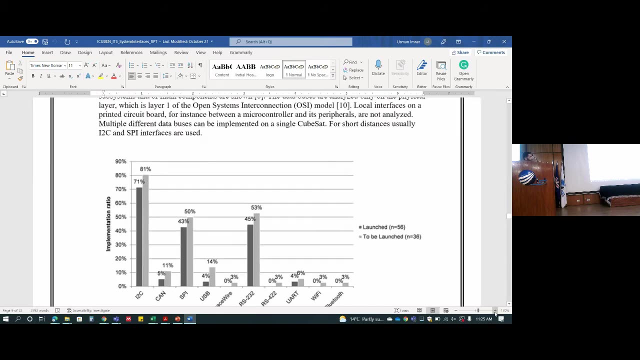 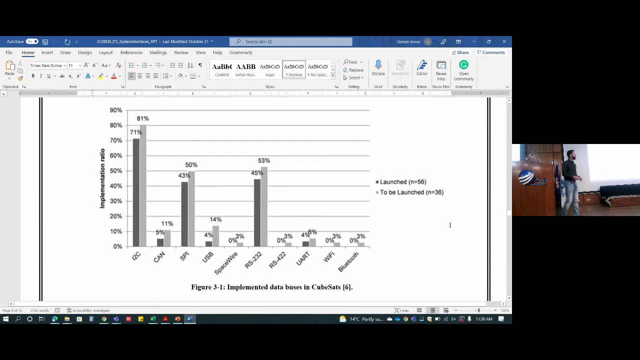 are implemented. This is a graph which shows the usage of different kind of interfaces that have been implemented in the CubeSats from the beginning of their time, 2002, up to and till 2017.. So, as we can see that the I2C- it has been initially used a lot. 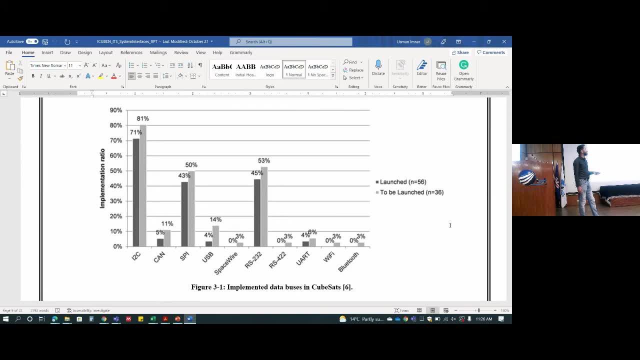 Then the CAN is around 5% in case of launch and 11% to be launched, So we can call the CAN protocol as an emerging protocol. The SPIE: it is 43 to 50%. USB: it is 4%. SpaceWire: 0 to 3%. RS-232: 45 to 53% USB. UART, WI-FI. 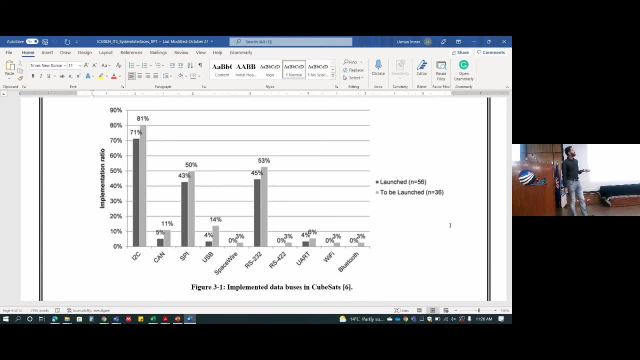 they are also between 0 to 3%. So from this we can see that the I2C- it has been used a lot, and after that SPIE and RS-232 are 485.. And in recent years We have seen that The trend is developing towards the CAN protocol. 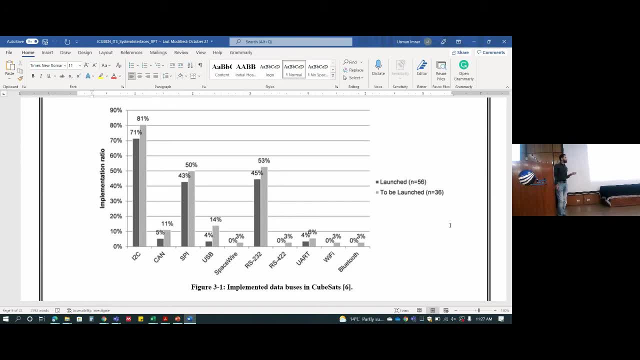 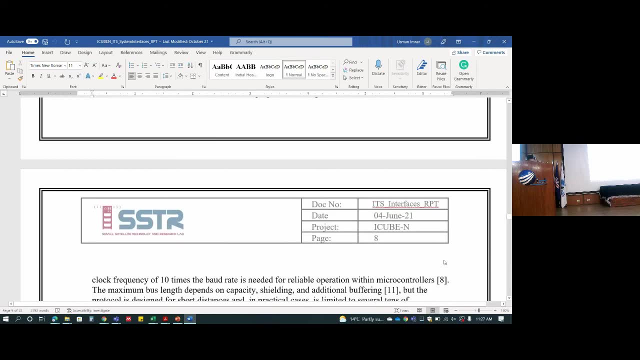 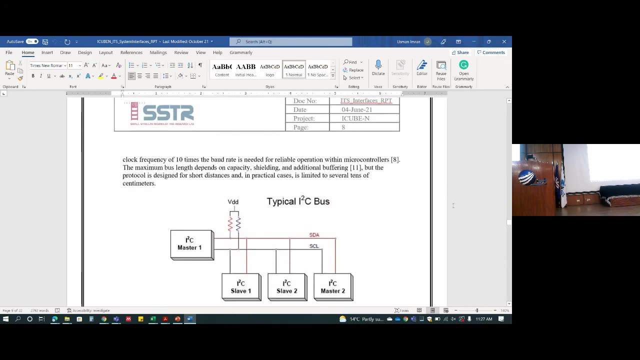 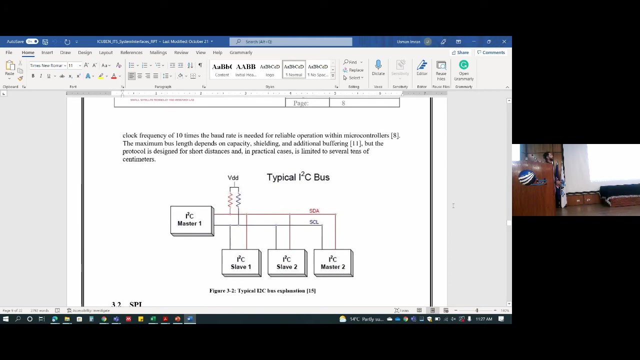 So this image. it is taken from a review paper. So now let's have a look at these I2C and CAN protocols, how they differ. So in case of I2C protocol, We have a master device and then there are number of slave device and they all are connected. 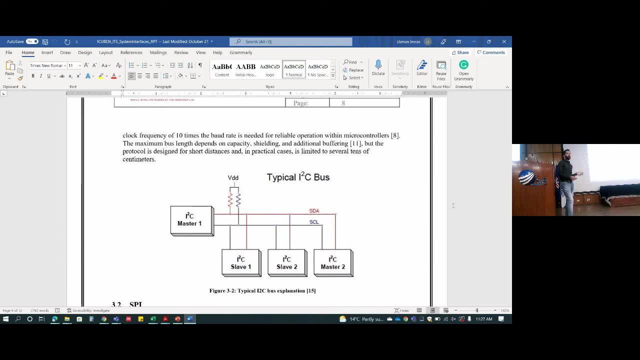 We have two line buses: one is data SCA and the second one is SCL clock signal. So its data rate is around 100 to 400 kilobit per second and this is the configuration for I2C. And if we have a look at SPIE, 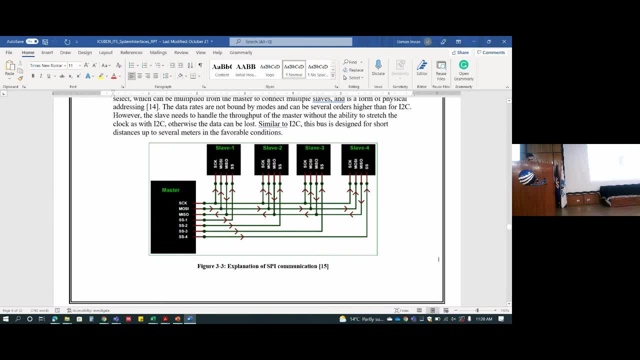 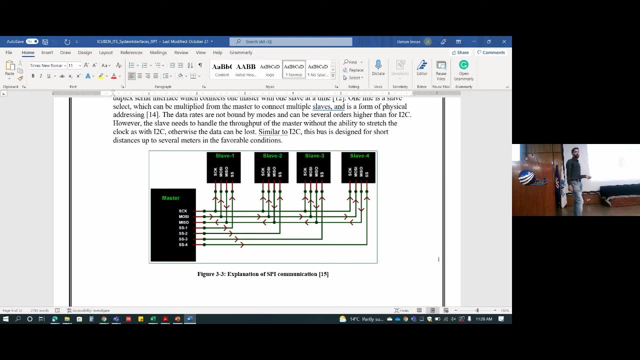 So It also has master and slave concept, but there are different number of signal lines in this one. So in I2C we have two lines, SCA and SCL, but in this case we have clock and master out slave input and master in slave output, and then we have this selection line also. 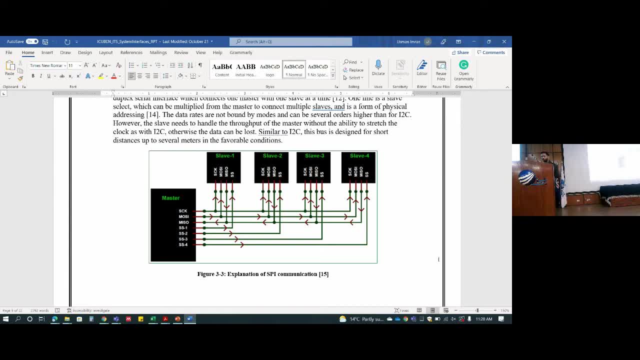 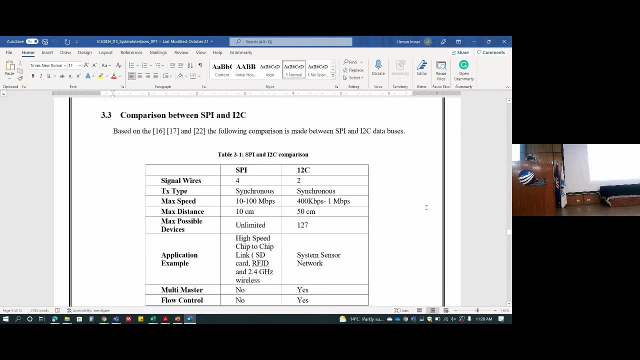 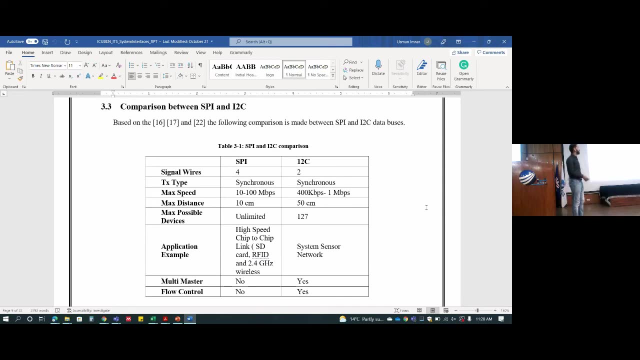 So typically this has four lines and in case of I2C we have two data lines. So this is a comparison between. so whenever we are selecting some protocol for our device, we make a comparison between them. So the SPI they are four signal wise, I2C have two, because both of them are synchronous. 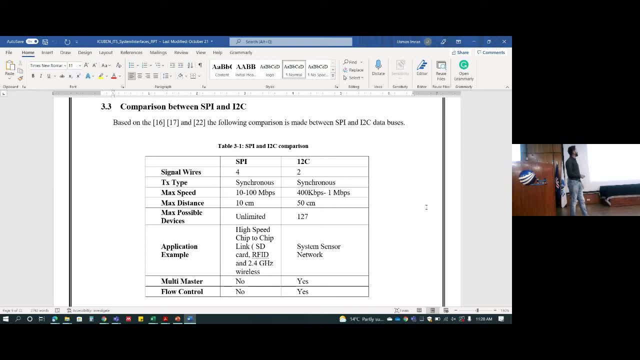 So SPI. it has slightly higher data rate than I2C and maximum distance for SPI is 10 centimeter, for I2C is 50 centimeter. So this is the comparison between I2C and SPI. So that's it, Thank you. The maximum possible devices up to 127 are limited And in case of SPI we can only have so if the monster is not possible, we can only have one monster and other devices, but in case of I2C we can have multiple And the flow control. 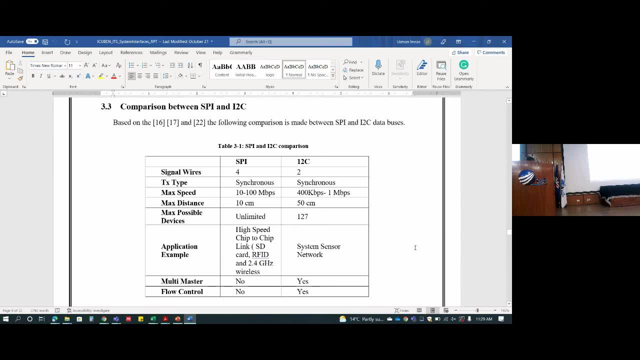 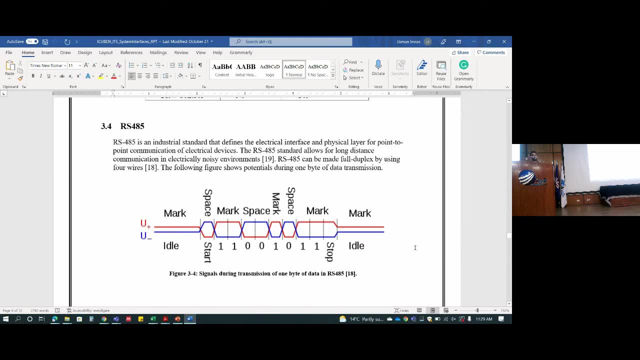 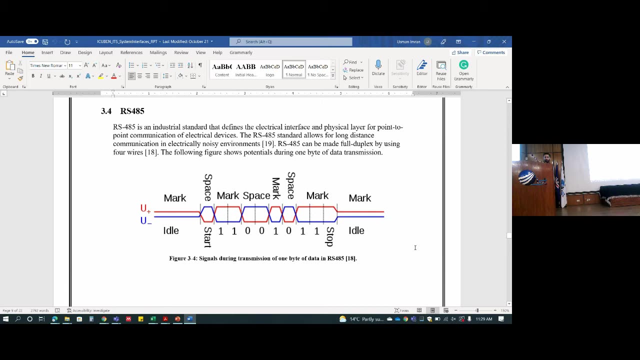 is no in case of SPI and for I2C it is yes. So this is for the SPI and I2C. So now let's have a look at the RS protocol. So there are three RS: 232, 485 and 422.. 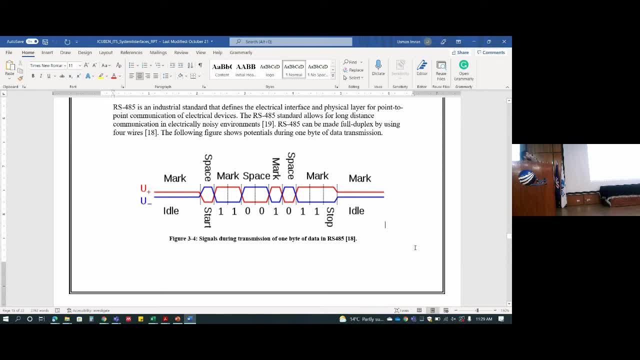 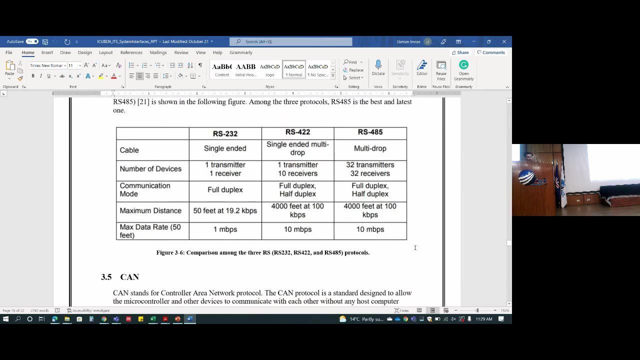 So this is signal for the RS 485 protocol. It consists of mark then space, So basically this is at a bit level, so you don't need to have a look into it. Let's move on to the comparison between RS 232,. 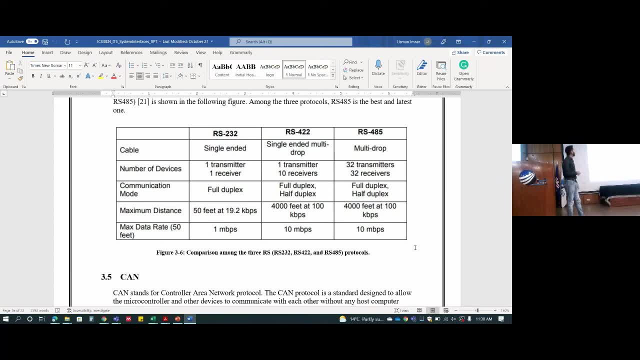 422 and 485.. So the table is single ended. In case of RS 485, we have multiple. The number of devices in RS 232 were one transmitter, one receiver, And for RS 482, it was one transmitter, ten receivers. For RS 485,, 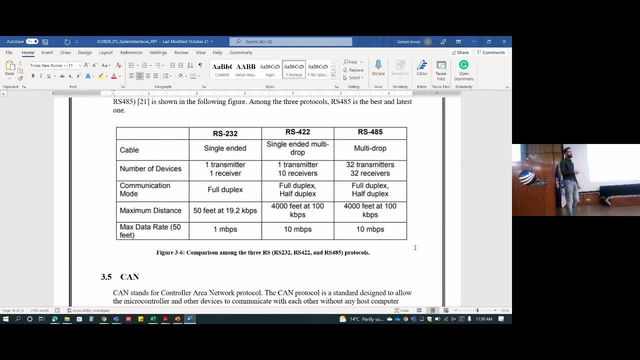 32 transmitter and 32 receivers. So in this RS series we can say that the RS 485 is the most latest or it has more data rate. So in case of 232, it is one Mbps, for 422, 10 Bps and for 485 also 10.. But the number of receivers 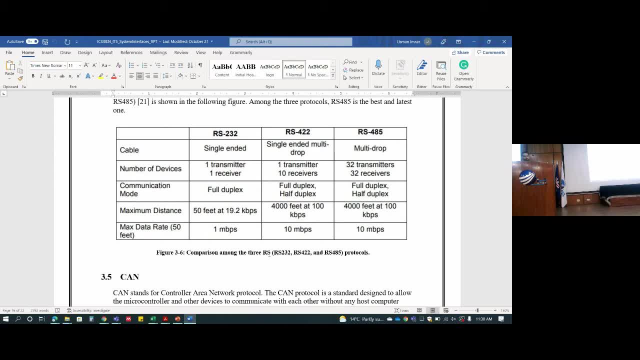 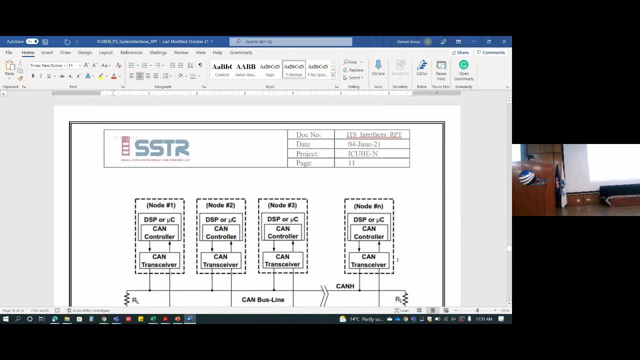 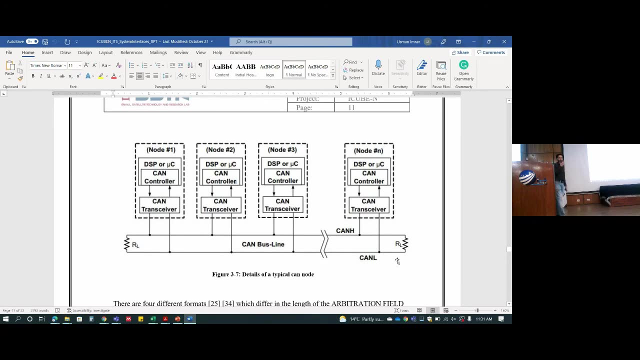 and transmitters are more better in case of RS 485.. The next one is CAN protocol. So this is the configuration for CAN protocol. So, instead of the master or slave concept, what happens is that we have two lines, CAN high and CAN low, And we don't have some master or slave. 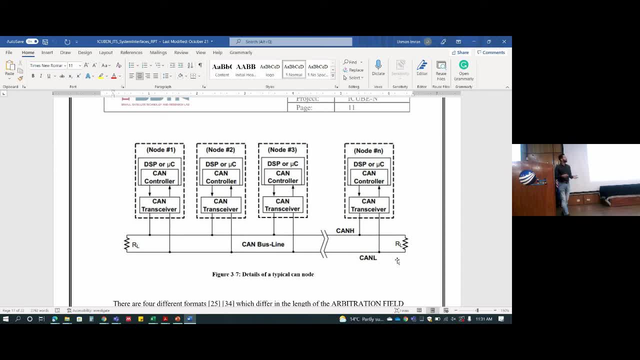 And it works on the basis of the message format. So this node one, let's say this is a block one, some OBC. node two, we can say this is ADCS. we can say node three, some other node. So they all have a CAN receiver and a CAN controller on them. 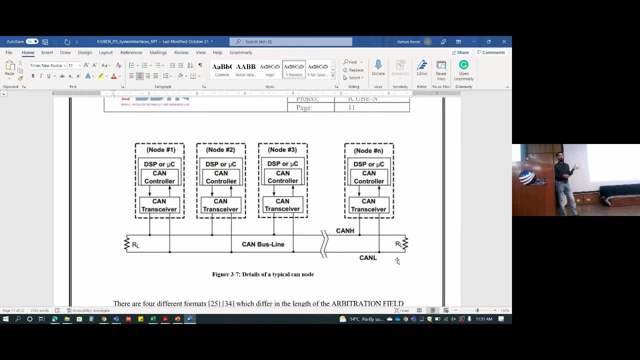 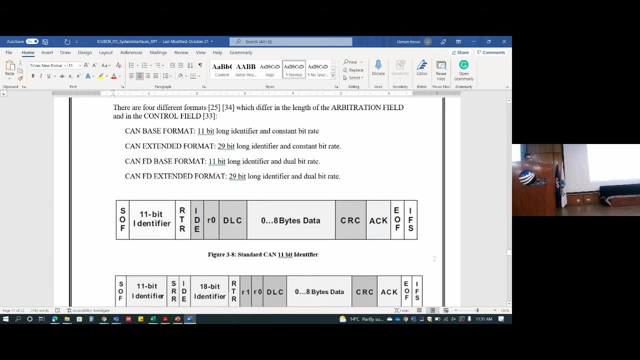 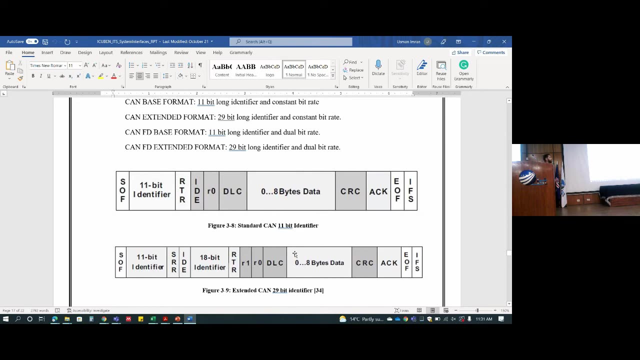 So whenever they want to communicate, they send a message on these CAN high and low line And that message is in the format of: in this format. So there is a start bit, then 11 bit identifier, Then we have different number of checks. 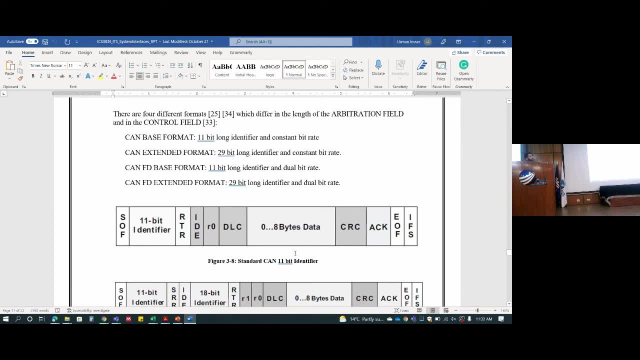 RTR IDE and then comes the eight byte data And then also there are some check bits like redundancy check, acknowledgement bit. So this is the bit structure or the message format for the CAN protocol. There are further two standardized CAN, like one is 11,. 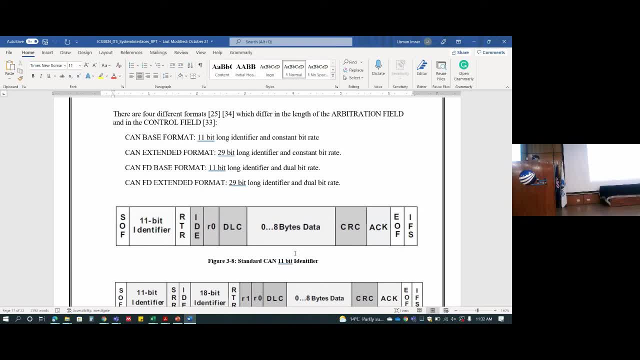 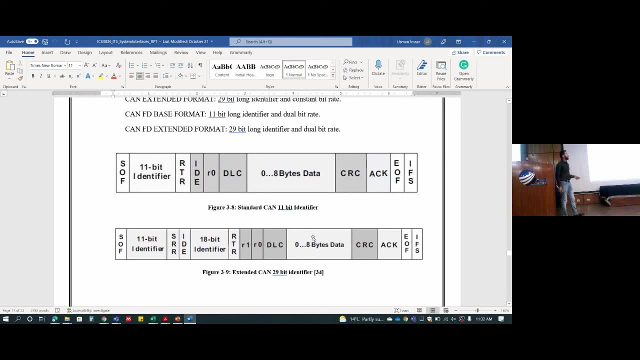 one has 11 bit identifier and the other one has 29 bit identifier. So the number of bits of identifiers are different in each case, but the number of data bytes and the redundancy or acknowledgement bits, they are same in all of the cases. 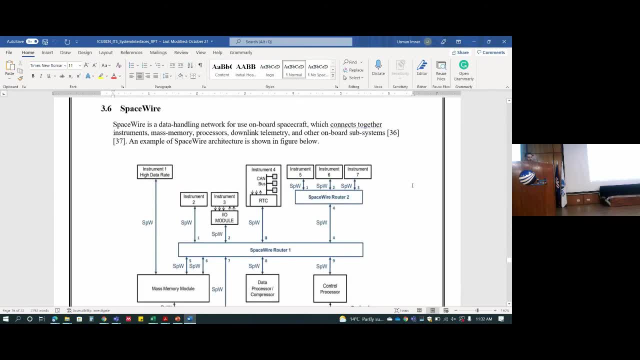 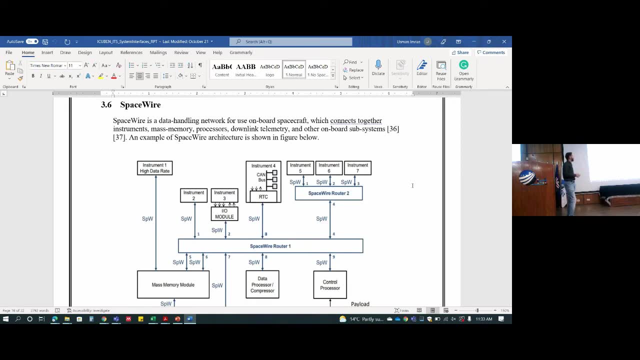 And then there is a space wire protocol which is used also by some of the largest satellites, or maybe more so. they also have these kinds of protocols. But what the limitation or restriction is in this protocol? that they have specialized routers and hardware for their purpose. 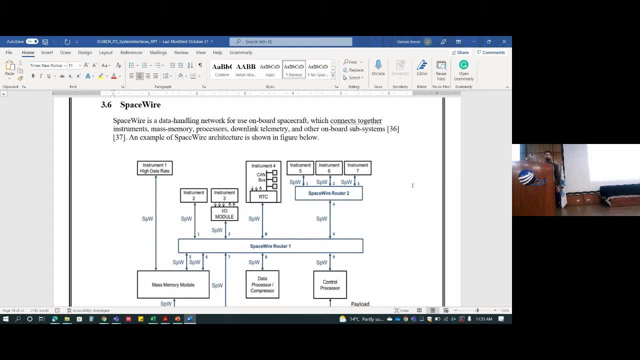 So this is not easily available for everyone or every user. So what we do is that we have to decide some protocol from I2C, SPI, CAN or the three series of RS, RS-422, 485.. So making a comparison among them, 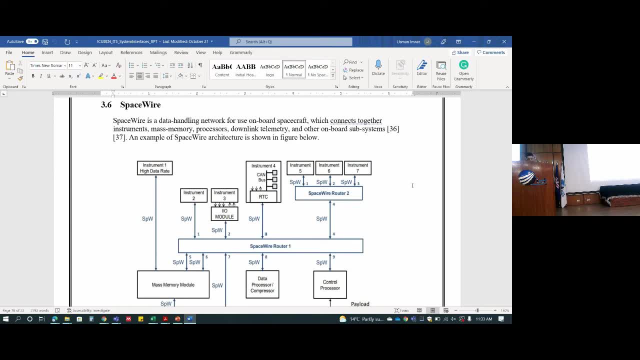 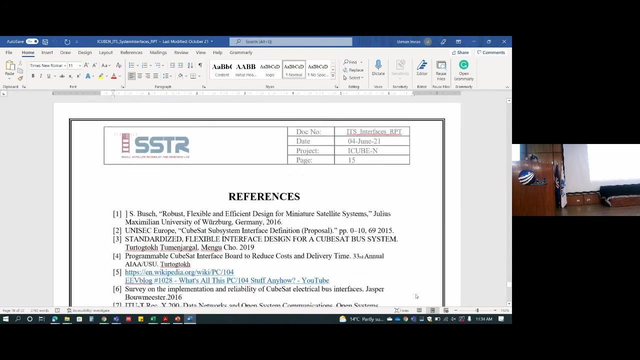 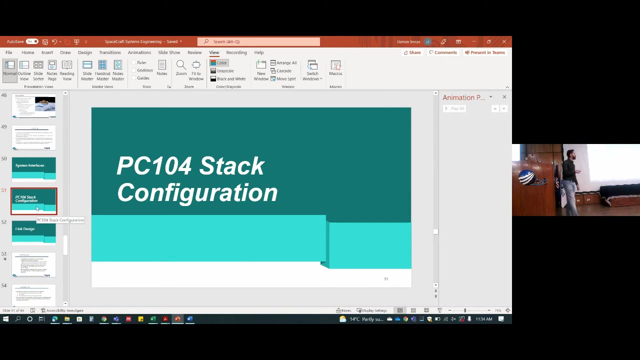 and developing the trend, we decided to have the CAN for our IQ-BEN. So this was some detail about the different kinds of protocols. Okay, so that was all in the protocol section. So if I summarize it, it has four to five protocols. 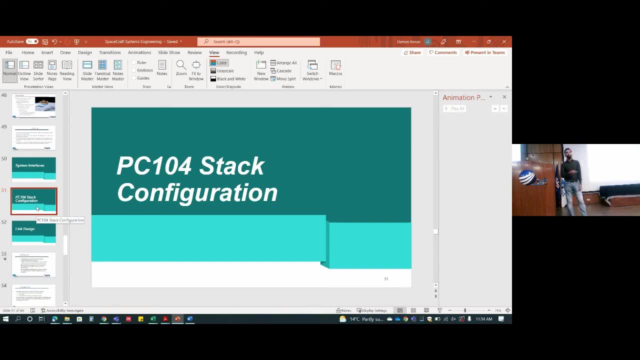 I2C, SPI, CAN and three series of RS protocols And if we have to decide some protocol, we make it based on comparison And we check our requirement: number of transmitter receivers and the number of and kind of data transfer format. 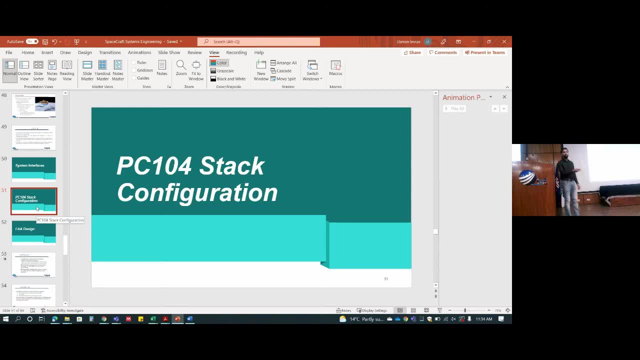 Like it has. one has master-slave, other has the message format. And then I told you that in the current development of satellites the whole shift has been towards the CAN protocol because of its message format And data rate also, and the number of devices. 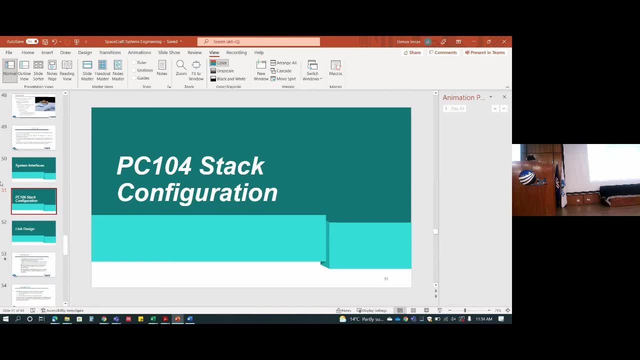 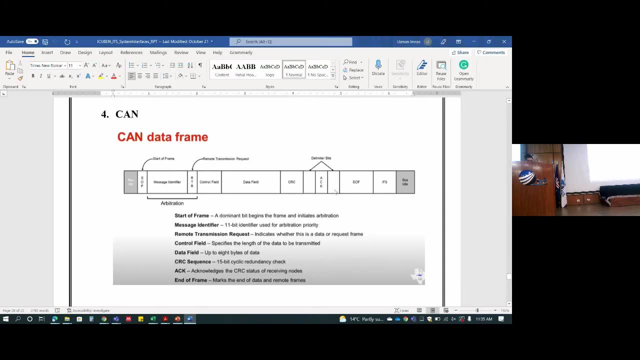 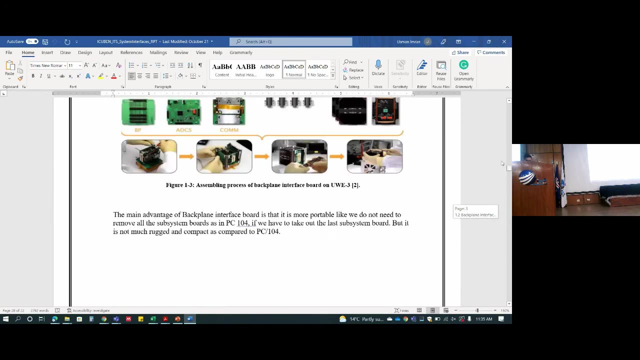 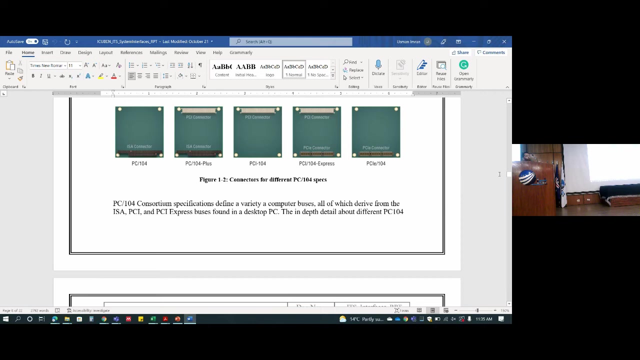 there can also be a lot of them. So the next: now we will move to PC-104 stack configuration, So this connector which I showed you that most of the Cube satellites have this kind of connector, and we stack them. So now let's have a look at. 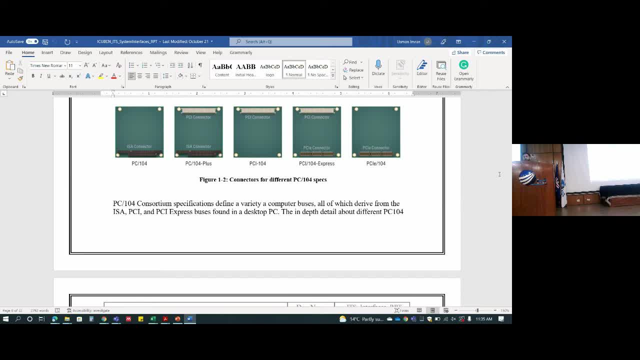 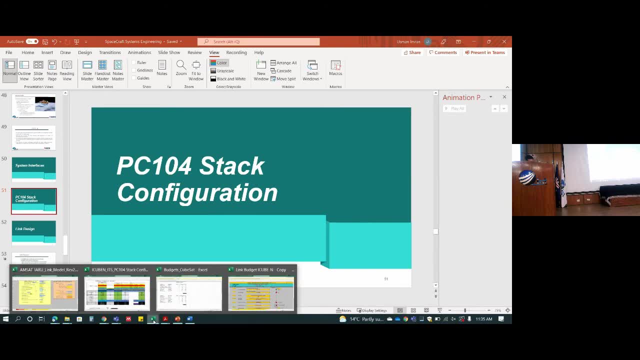 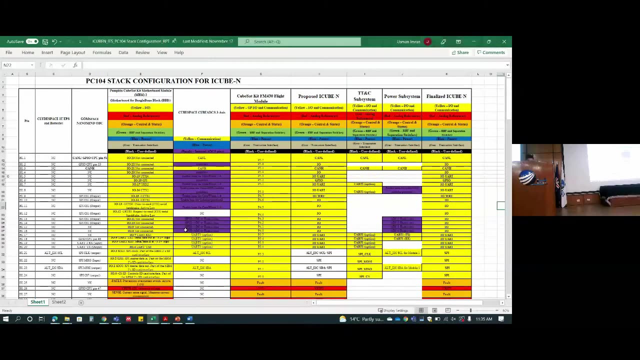 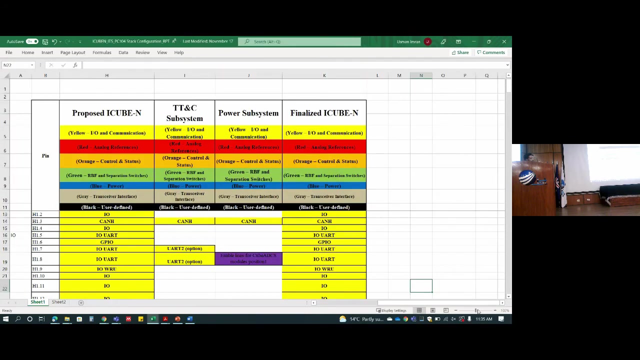 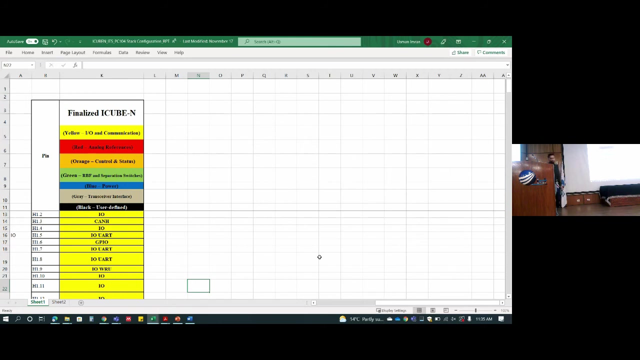 how their pins are numbered and how we decide which pin will have what kind of functions. Okay, can you last member, can you see this clearly, This light? Okay, so the color sequence is that the yellow is for input and output communication. 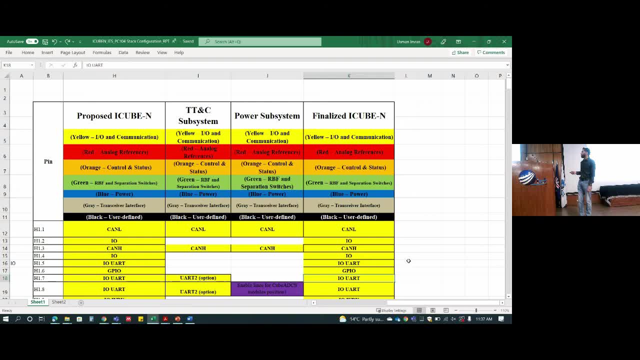 red is for analog reference, orange defines the control and status bits, green is for remove before flight and some separation switches, blue is for power gray for transceiver and black is for user defined. So most of these if you look at this table, 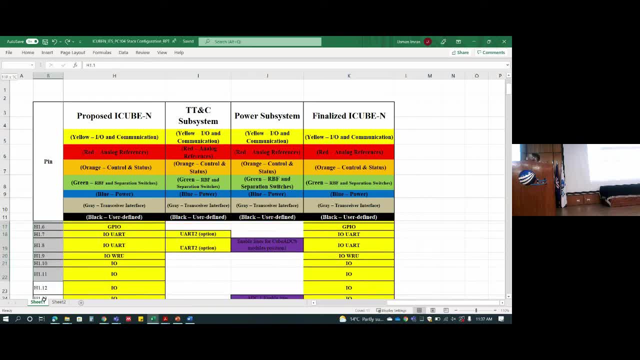 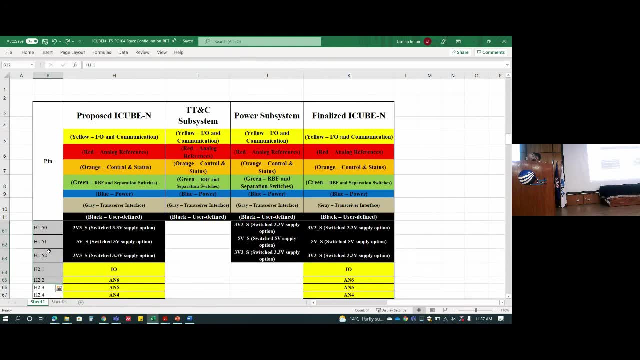 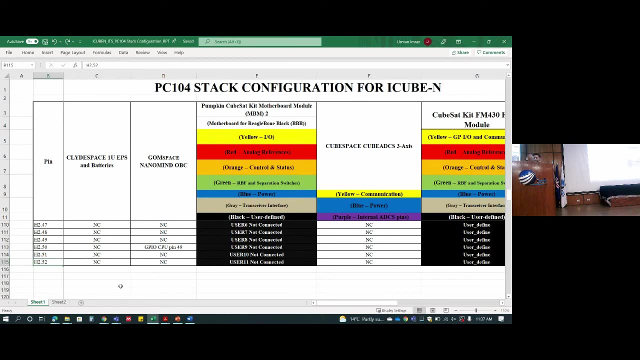 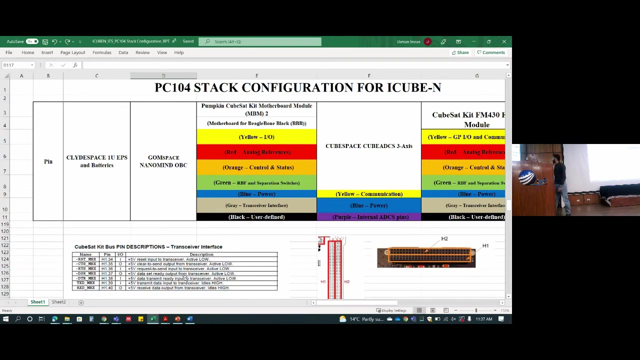 this column. it is numbered from H1 up to H52.. So this is header one. And then, if you look at H2, this is also numbered from H2.1 to H2.52.. So this is the header definition. 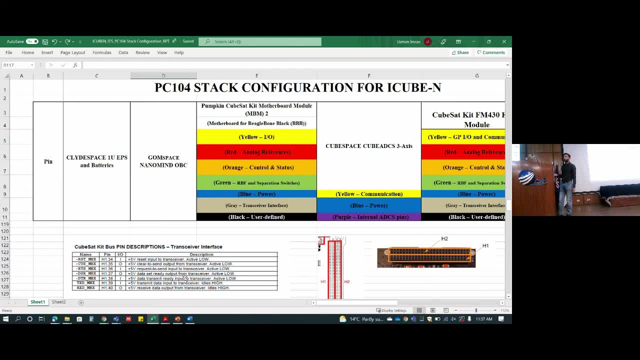 This one is: this is header and it has 52 pins. Similarly the H2 header two. it also has 52 pins. So now we have to decide that, okay, this pin will have power, This will have some I2C signals. 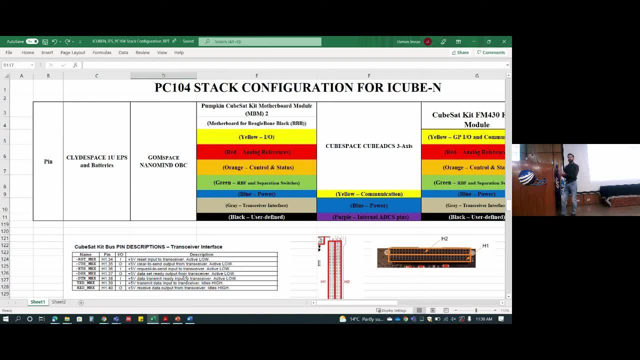 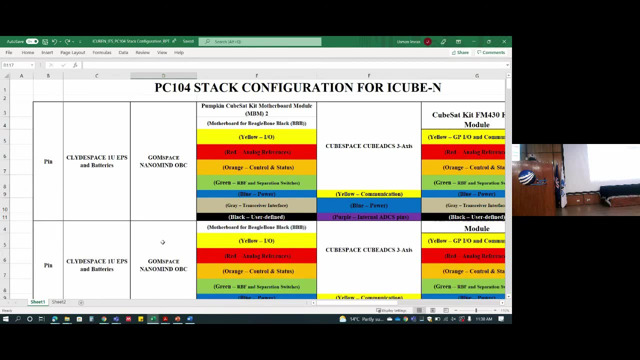 but how do we decide that? So there is some standard for that also, And there are some user defined pins. We can also define them accordingly. So let's say that, for example, if we have a look at some commercially available boards, 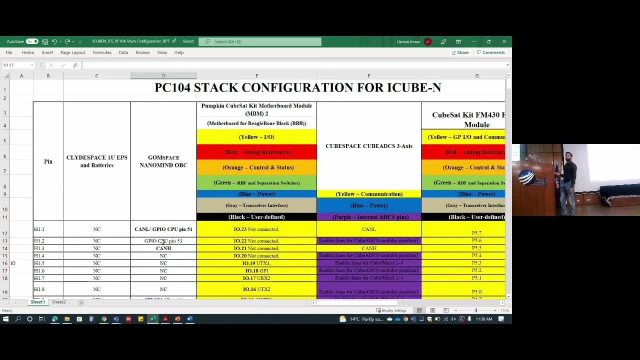 so this one is GOM space Nanomind OBC. So if we see what it has on header one and header three, we see that it has CAN low and CAN high signal. Similarly, if we check for the CUBE ADCS. 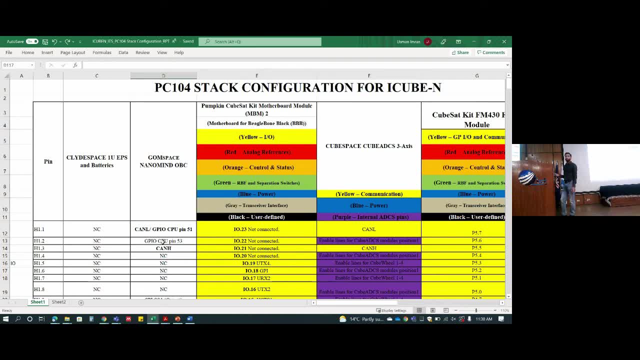 it also has CAN low, CAN high. So this is showing that it is kind of a standard. So whenever we we route our board so we have to put the CAN on pin one and pin three. So this is one example for that. 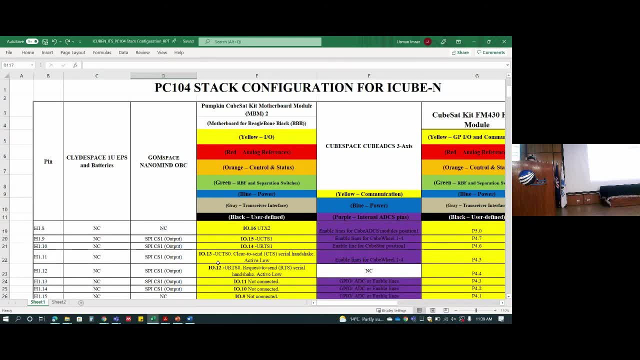 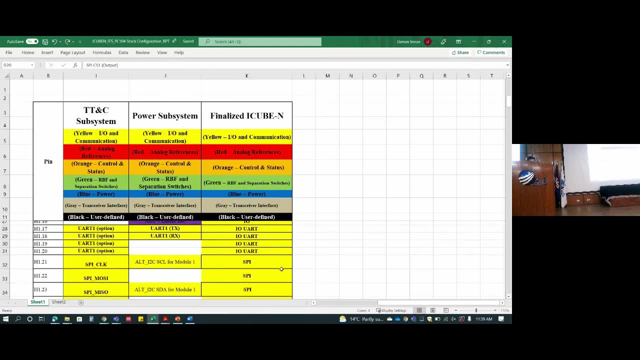 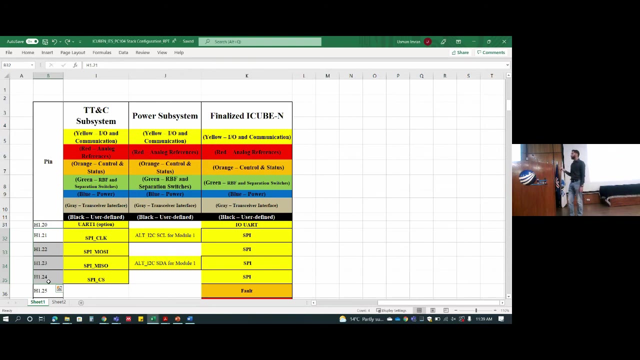 If you look at header one, if you look at header 21 to 25, so they also have the SPI protocol signal. So if we are using, we need to define them at these pins, H21 to 25.. So this is also kind of standard. 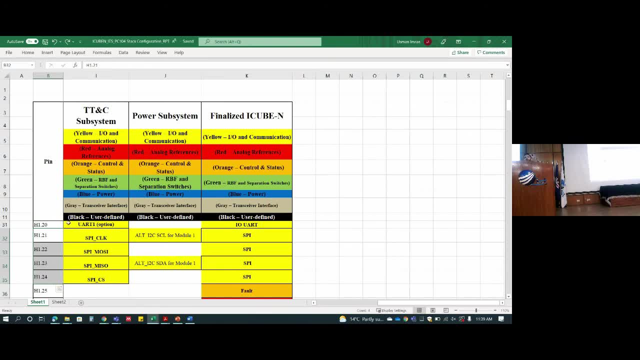 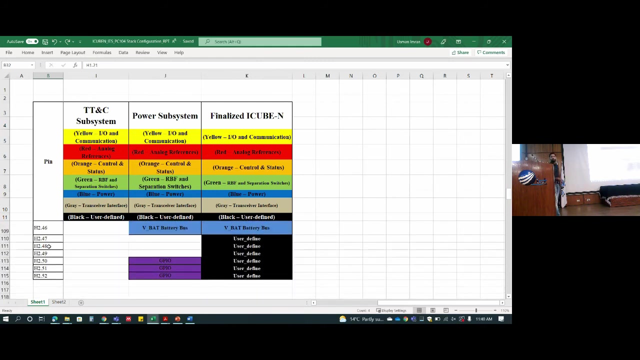 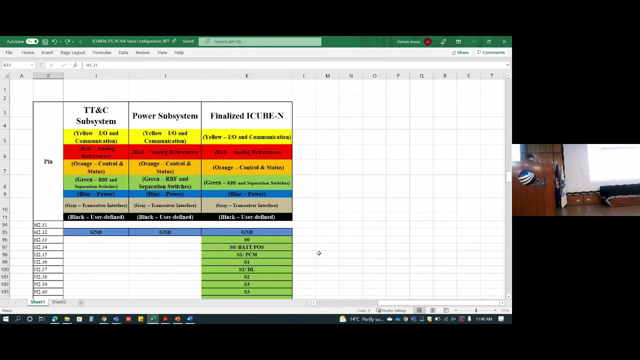 So, when we define the pin for this PC104 stack configuration, the pins which are standard, we keep them as standard And what we can do is that let's say if we want to doевой or standardised, As I told you about the CAN, which is on header 1 and 3.. Similarly, if we have 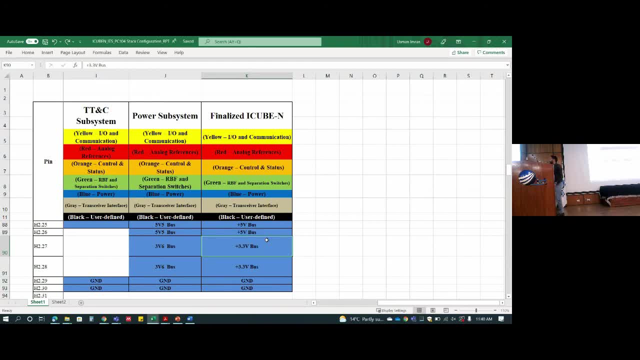 a look at the power buses. so we always have five board at header 2.25,, 2.26.. So whenever, if you are developing a board by yourself, it will be on same, and if you buy a commercial board, it would also be same. So the purpose is to maintain compatibility so that if you 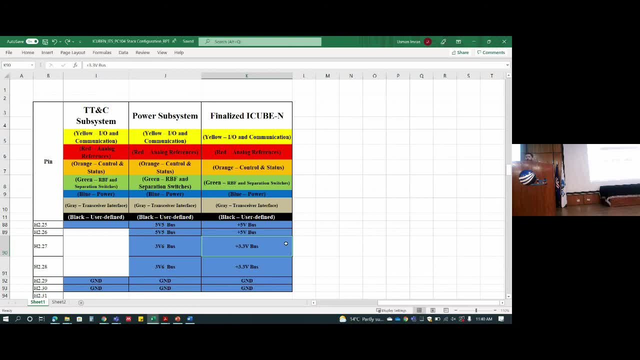 buy some commercial component and some of you are developing yourself so you can stack them together properly. So this is the purpose of this PC 104 stack configuration. So, if I summarise it, it says it has one of four pins, some of them are standardised and their 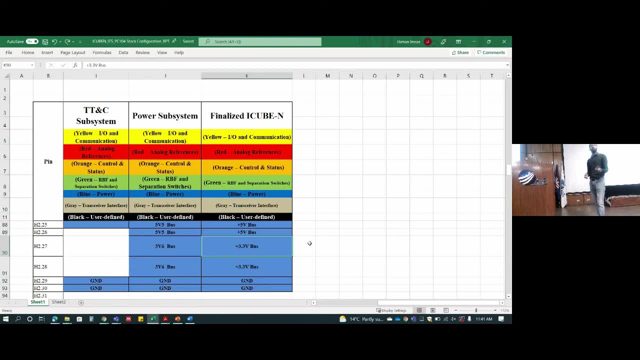 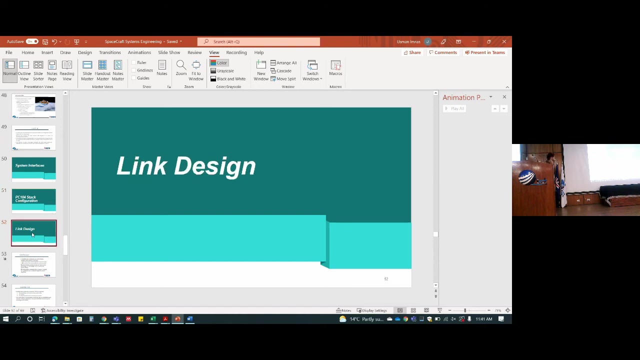 pin numbers are defined already and there are options for each of them. So if you are looking for user-defined pins, we can define them according to our payload or requirement, And so this is all in the PC 104 stack configuration. Next thing is about link design or link budget. 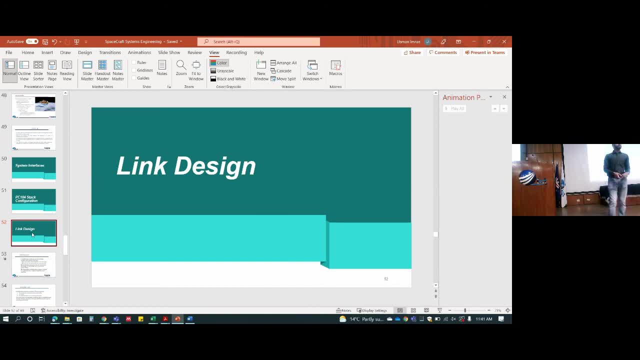 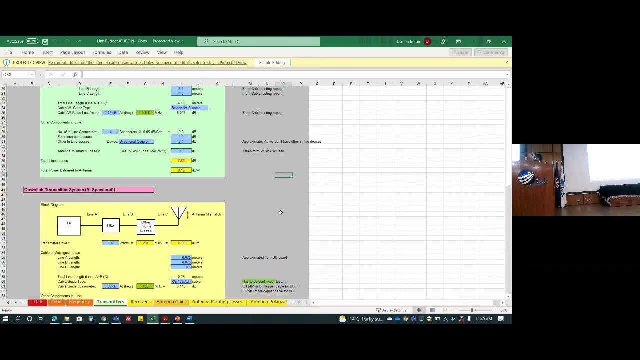 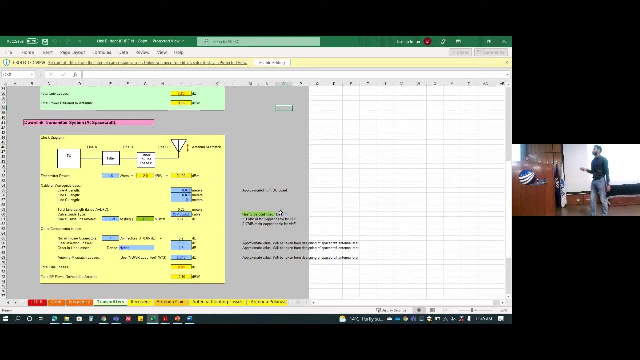 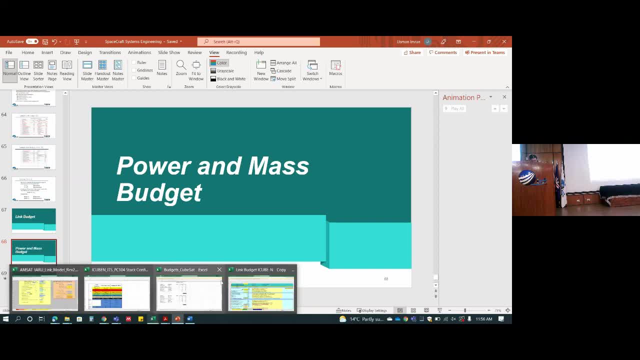 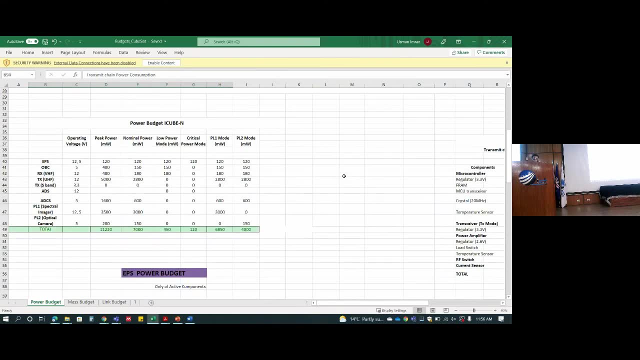